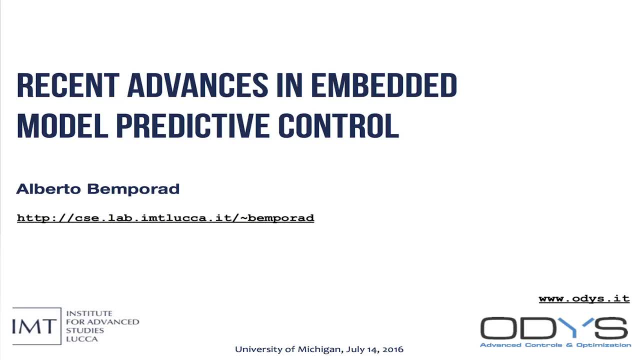 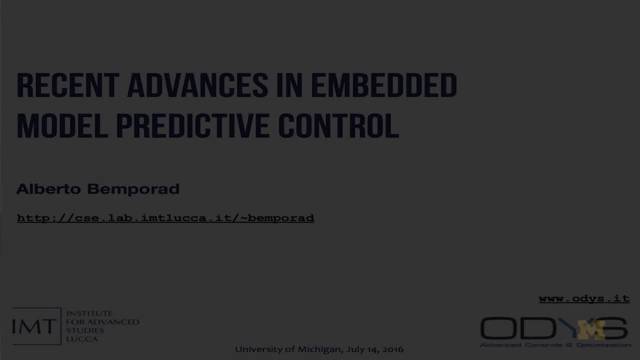 Well, thanks a lot, Ilya, for the kind introductions. Thanks everybody for coming, And I'd like to thank Ilya also for inviting me here in Ann Arbor to spend the summer here as a visiting professor. So I am very grateful for the opportunity. 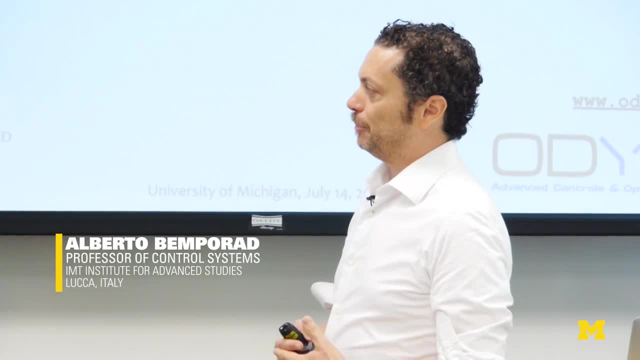 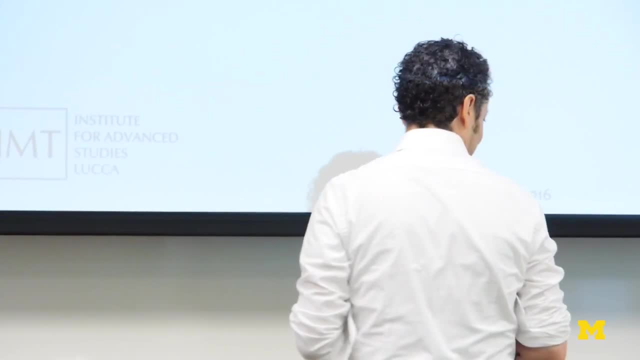 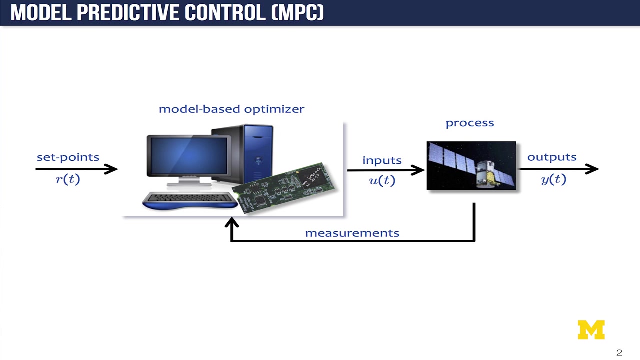 So today I am going to give an introduction to MPC and also cover some of recent research activities we have been doing in this field together with my research group In LUCA. So just a quick introduction of what MPC is. So you have a control problem. 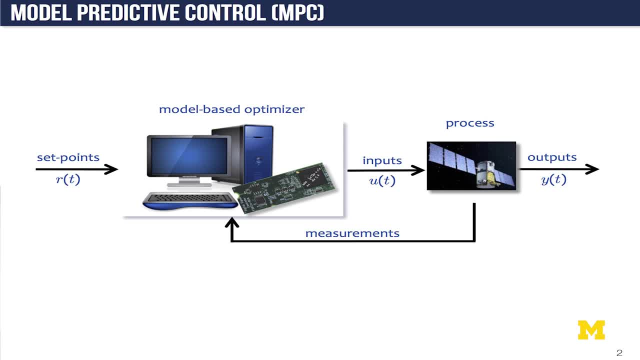 You have a system, You need to manipulate the inputs to the system and, as in every control problem, so that the outputs of the system track a given set points, And you want to do this in closed loop using measurements coming from sensors on the process. 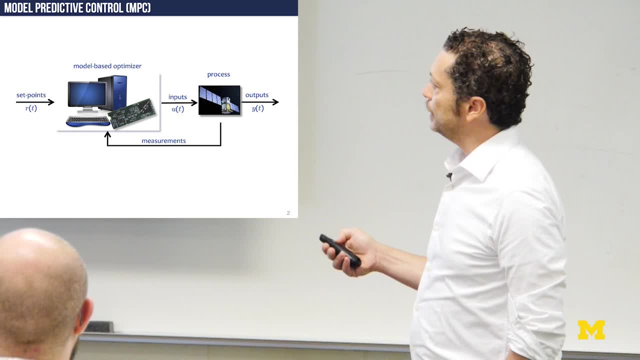 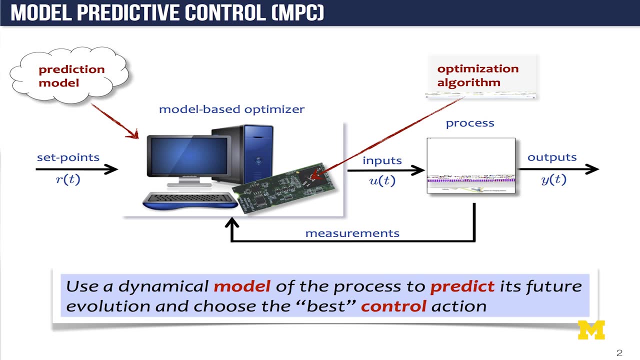 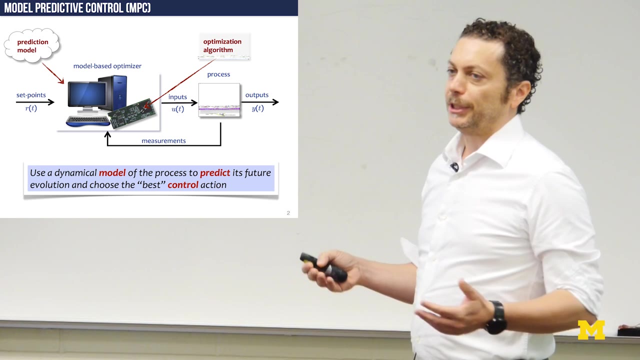 And the peculiarity of MPC is that it's using It's a model explicitly of the process to make predictions of what the future evolution of the process will be, depending on how you choose future control actions And, based on these predictions, you 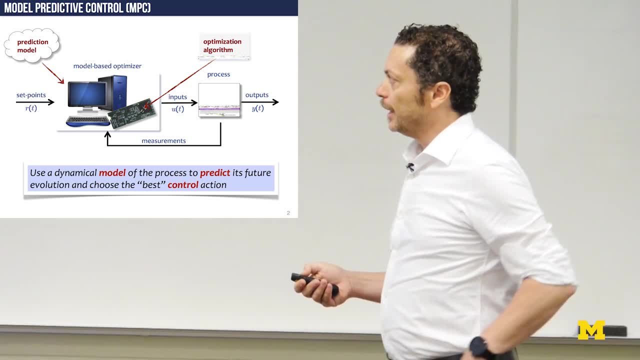 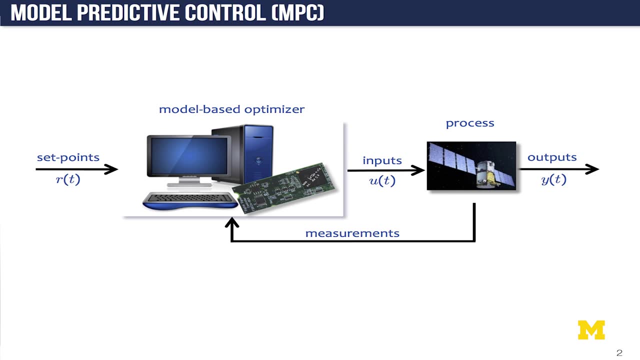 want to choose the best control action And this technique. it's applicable not only to special classes of system but to many classes of system like, for example, in aerospace for attitude control, the satellite for example, or in out of model control to control the torque of an engine, say. 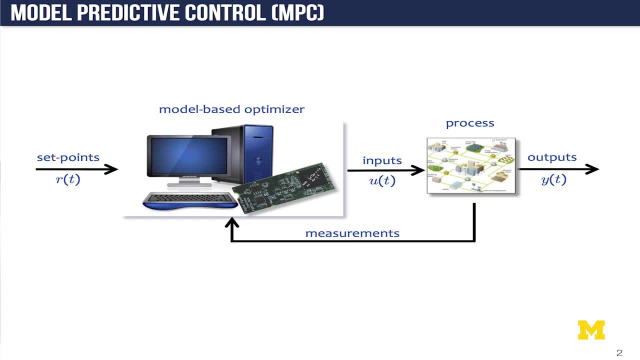 Or in chemical engineering, it's a bioprocess, or in smart grid. I will give you examples of different applications where the same ideas I'm going to talk about today are applicable. So what does it mean to choose the best control action based on predictions? 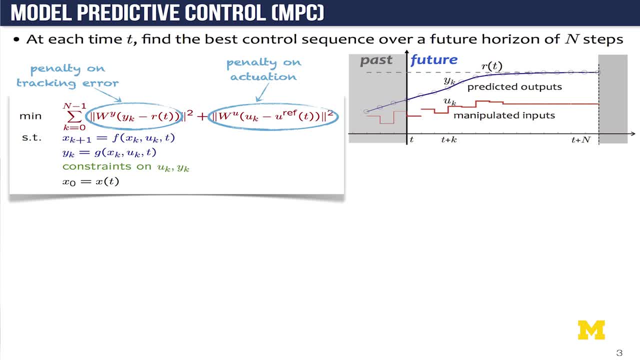 Let me state this a bit more formally And let me explain how the mechanism of MPC works. So let's say, now is the current time t. You use the model, which is the one written here in blue, to predict what the output is based. 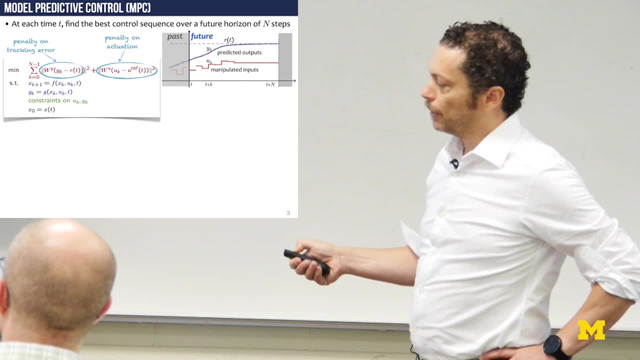 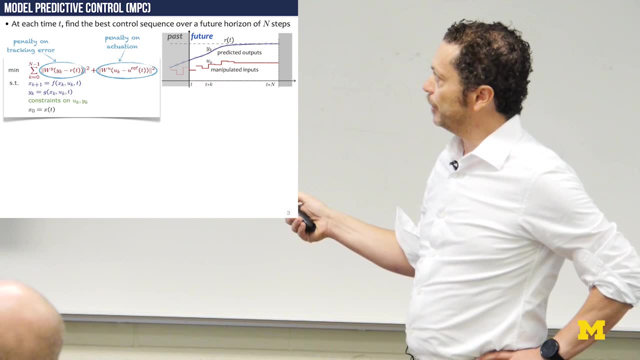 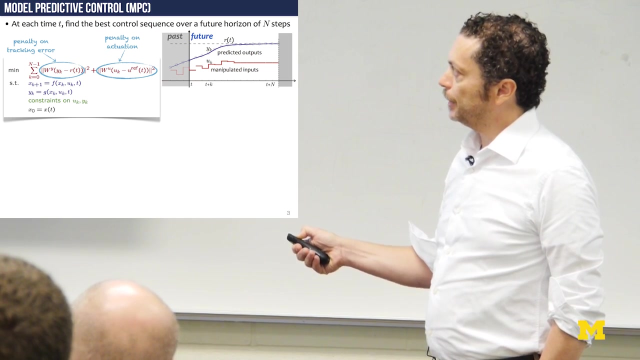 on possible selections of the input sequence, And then you solve this optimal control problem. You look ahead n steps in the future, so from the current time t to time t plus n, And the cost that you want to minimize is a trade-off between tracking the reference signal. 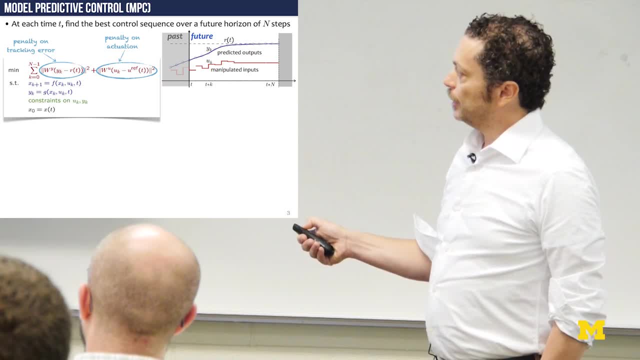 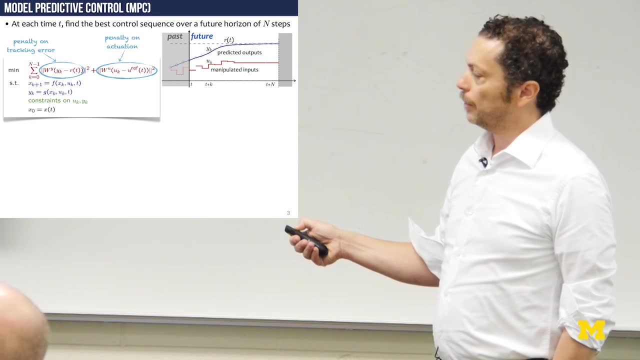 so you would like to have y as close as possible to r, the desired reference, Right The reference. but also you want to control what the actuators are doing. So you would like to have, for example, the actuators close to an optimal level for the actuators. 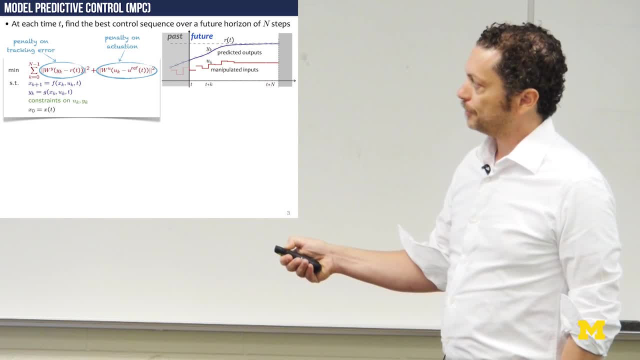 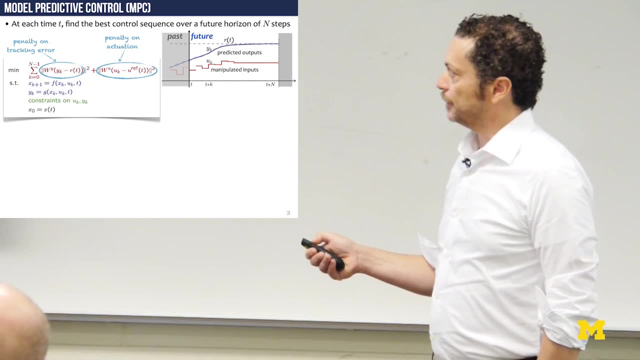 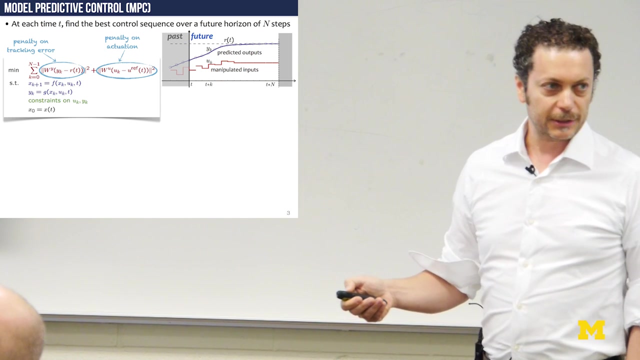 And this u ref may be optimized as a function of r to meet a higher order- let's say optimization criteria- And you solve this problem. The interesting feature of this formulation is that you can include constraints, So you can find the best. 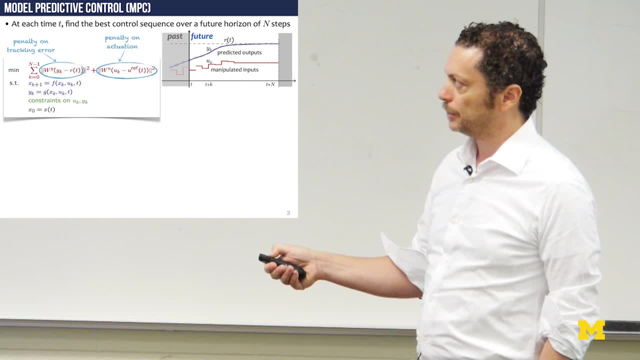 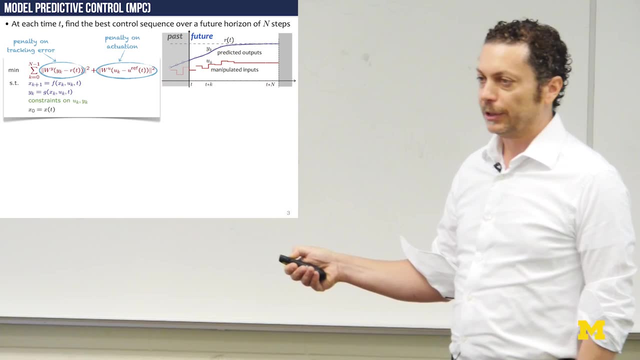 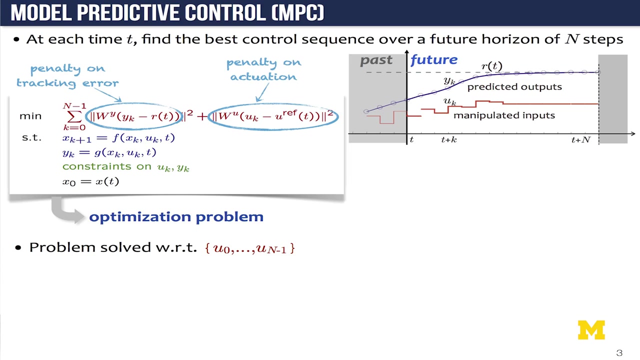 You can find the best control sequence solving this cost function subject to dynamics, but that they also meet some constraints. These could be constraints on manipulated variables on the inputs, u and also constraints on the outputs or the state vector as well. OK, so let's say you can solve this problem with respect. 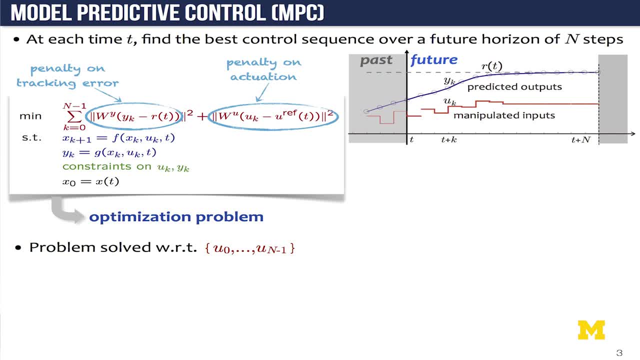 to a sequence of future optimal moves. Then what you do? you just apply the first sample of the optimal sequence- This would be the current u that you provide to the process, to the actuators of the process, And then you just trash away the rest of the sequence. 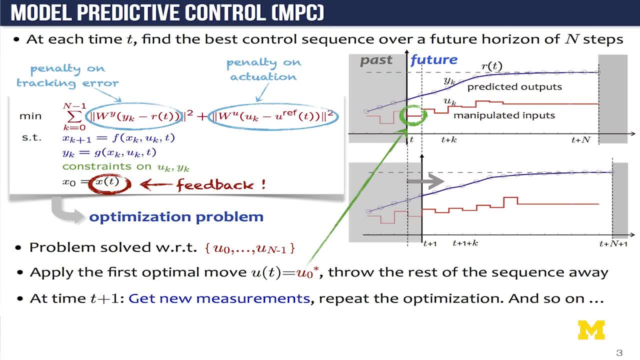 because at the next time step you will repeat the optimization over a shifted horizon- between the next time t plus 1 and t plus n plus 1, get the new sequence, which may be different from the previous one if things have changed from one step. 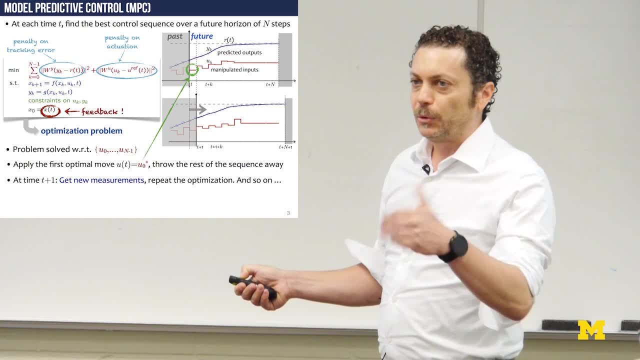 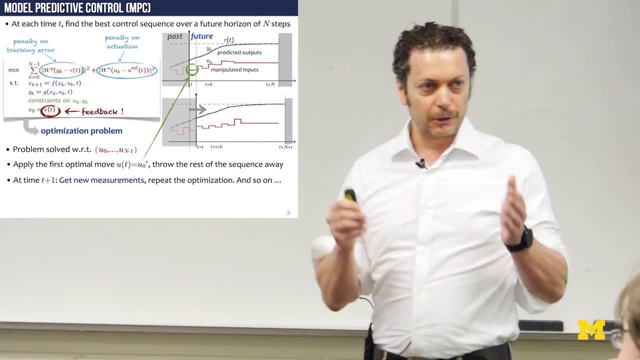 to another that you couldn't predict, And then you keep doing these repeated optimizations, And then you keep doing these repeated optimizations at every single sample step. This is also called receding horizon control, because the horizon where you optimize is receding over time. 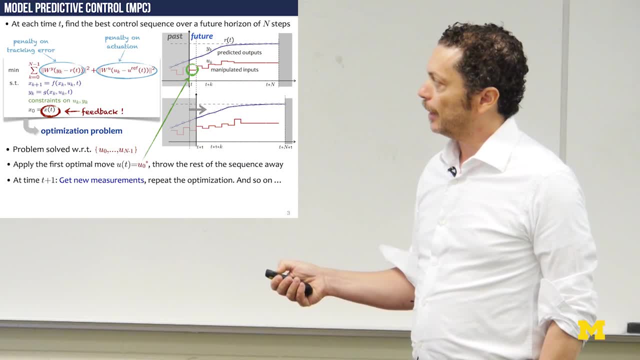 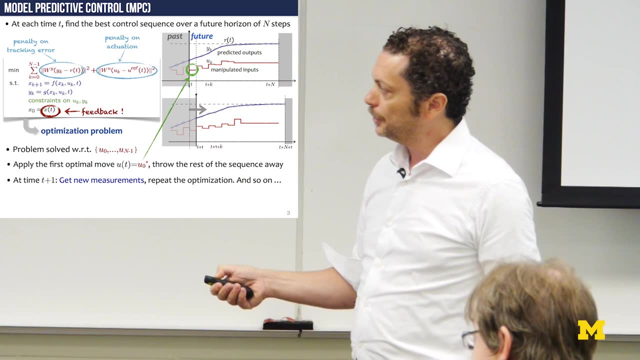 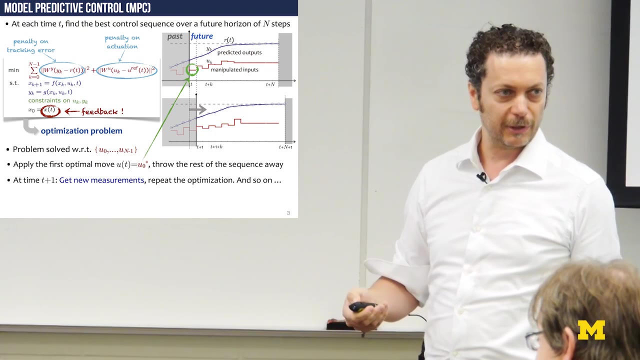 Now why doing this repeated optimization? The whole motivation is that you have a feedback control low, in spite of the fact that you are using an open loop controller based on open loop predictions. Then your decision, the? u that you apply, is always a function of the current state. 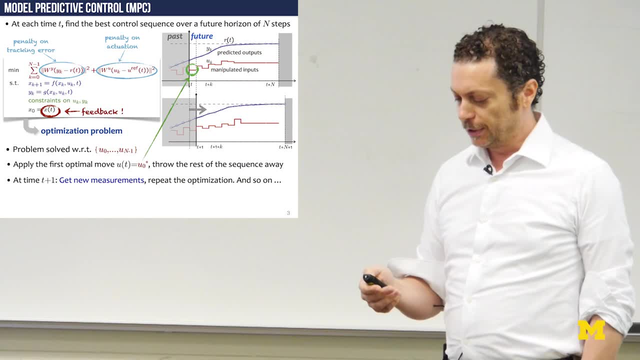 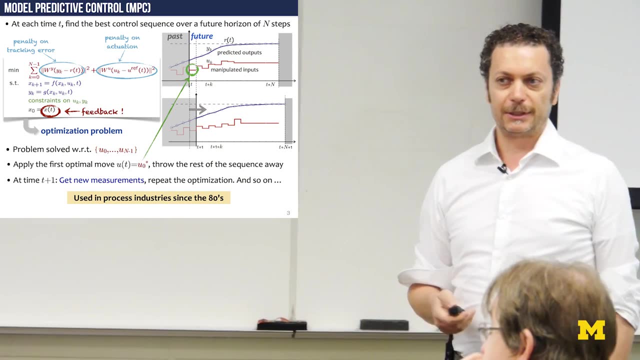 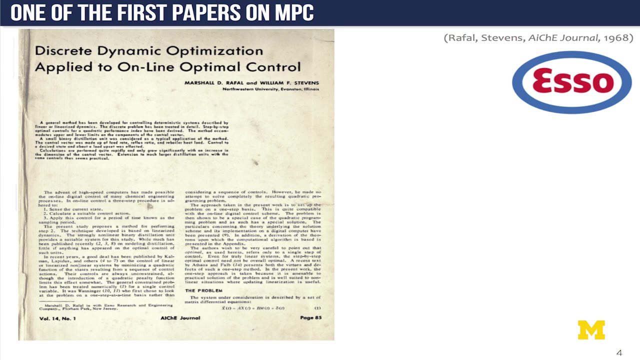 The current state. So indeed, this is a truly feedback control policy And this has been used in the process industries since the 80s, So it's not a new technique. Actually, if you dig back in the literature, this is probably one of the first MPC papers. 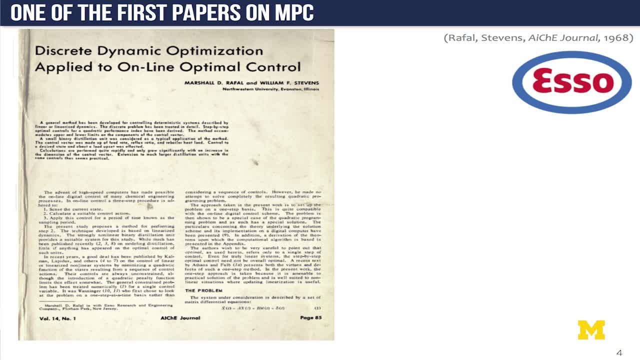 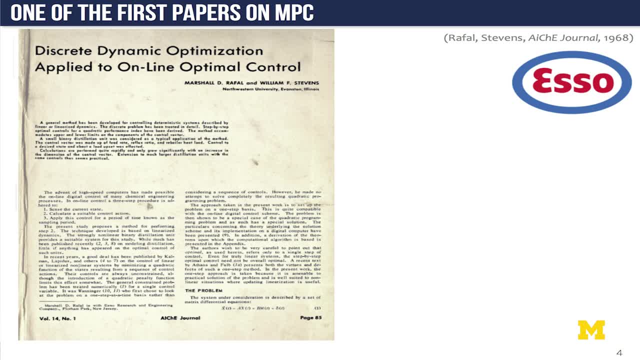 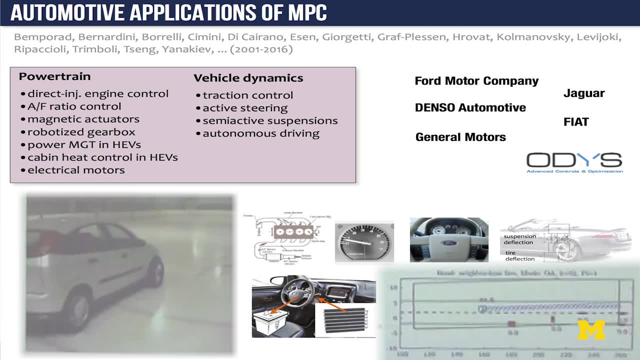 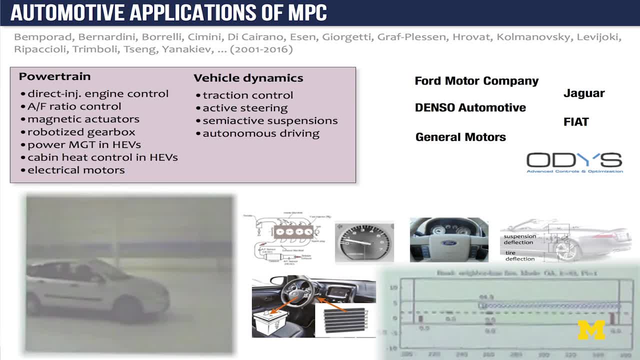 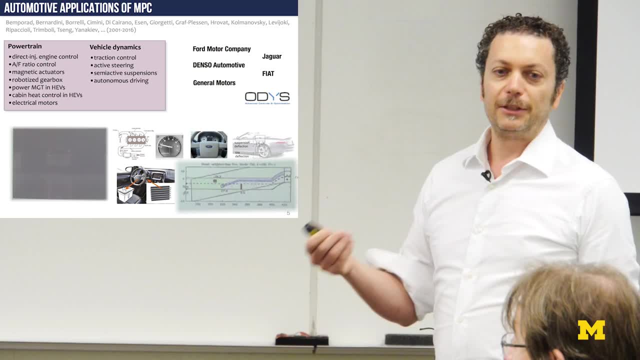 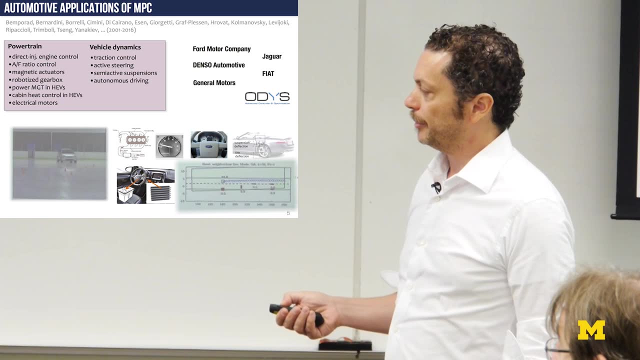 of MPC in other domains than traditional process control domains And in particular with Ilia and Davor Robat at Ford and other people at Ford, we have been looking at different control problems using MPC techniques to solve the control problem going from traction. 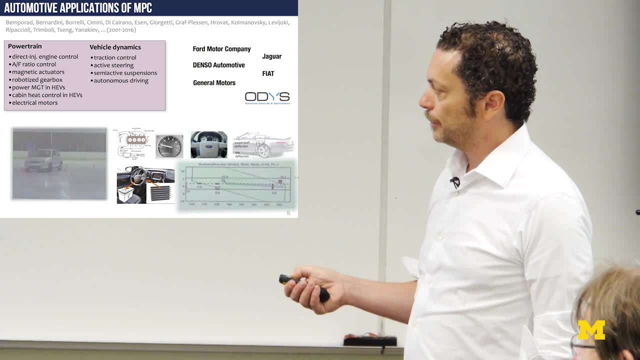 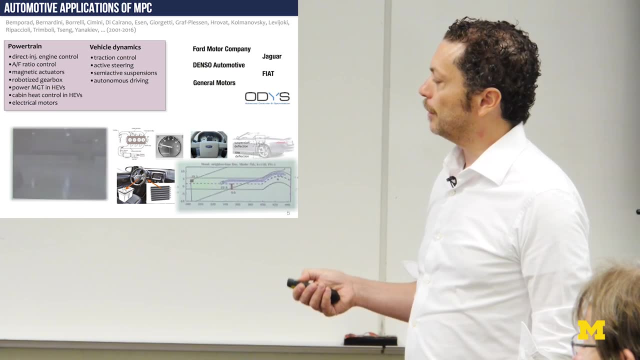 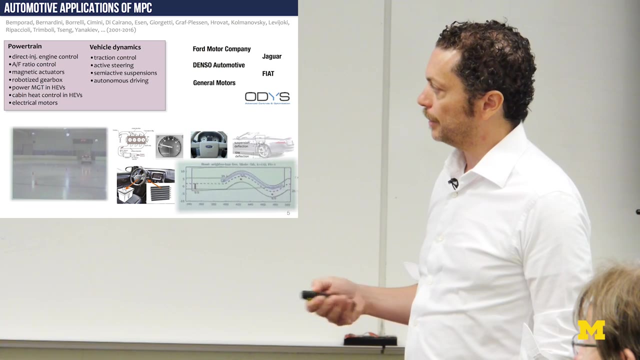 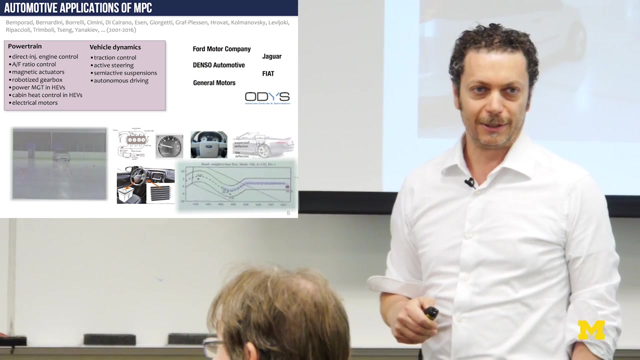 control, to steering and differential braking, to control of suspensions, engine control, cabin heat control And- this is a recent application we're doing with Denso Automotive, together with our company, All this on autonomous driving. So all these applications have been dealt with using MPC ideas. 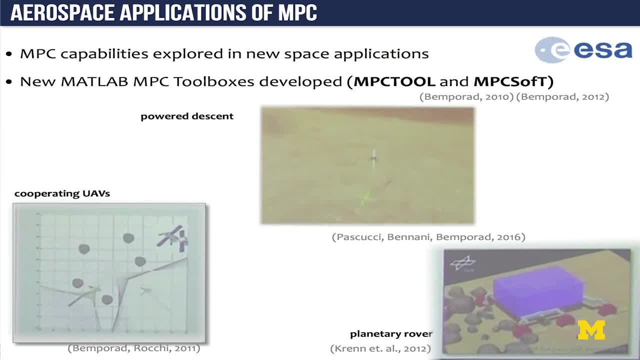 And also I've been involved, as Ilya was mentioning, together with the European Space Agency, on applications of MPC in the aerospace domain. In particular, we have been looking at MPC for power descent on a planet, for cooperating UAVs moving among obstacles. 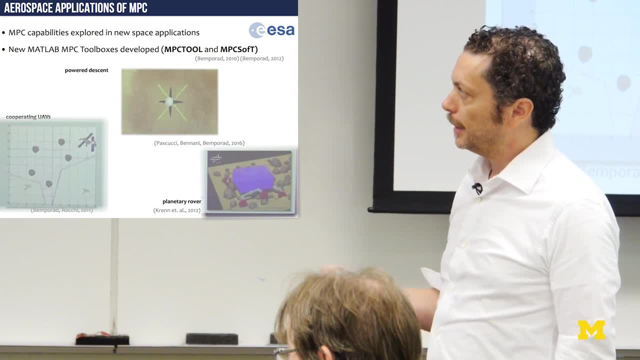 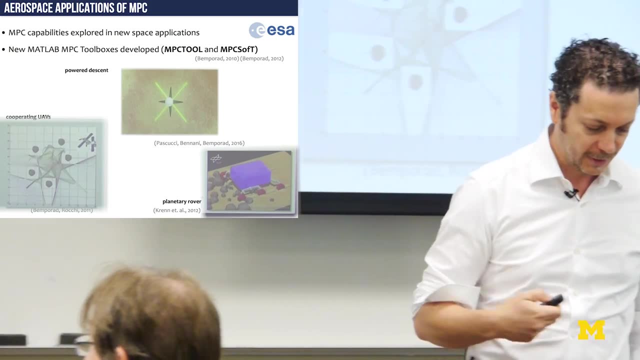 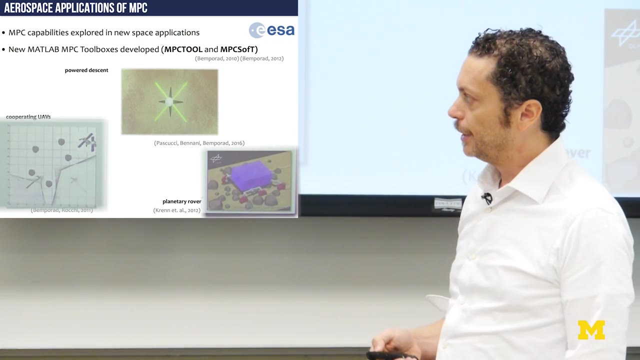 And also for locomotion of planetary rovers. I've been developing these two toolboxes that the space agency asked me for for giving European industries in the aerospace domain tools for being able to solve MPC problems, And other groups have been working on the application. 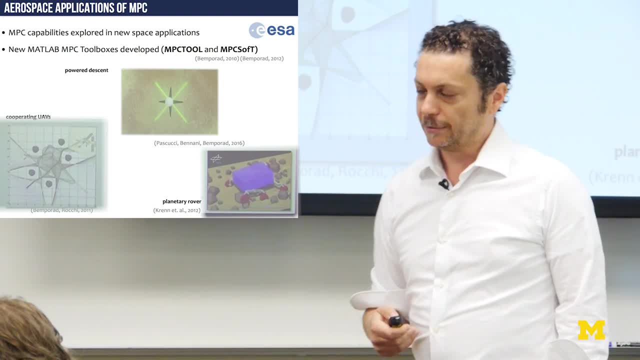 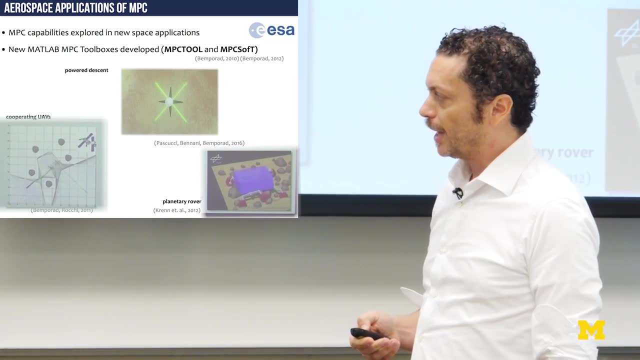 of MPC in aerospace. One is Ilya's group. There are others around the world. So I would say MPC started in the processing industries, as it's now. Thank you, That is now spreading into other industries- automotive, It's happening now, aerospace. 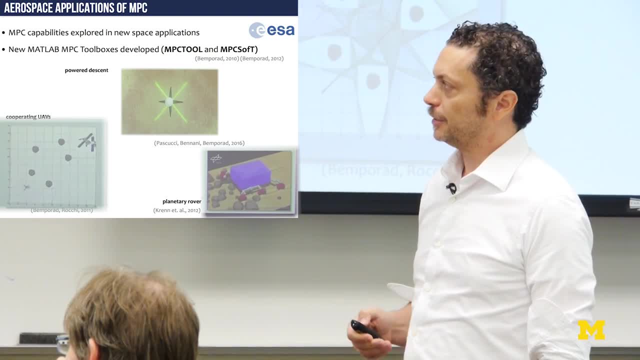 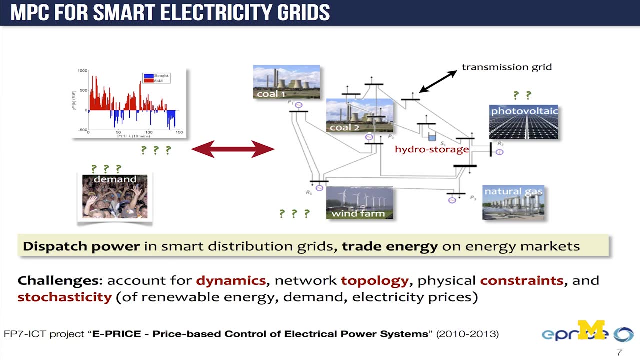 It's a bit slower, but it will happen too, And other domains as well. And here are other sample domains where I've been working on using MPC ideas again to solve problems in a smart grid where you want to decide in real time how to dispatch power. 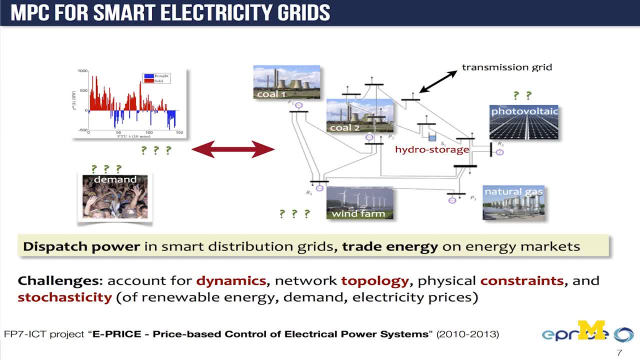 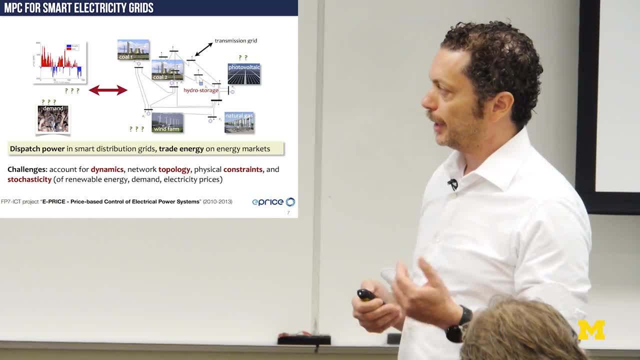 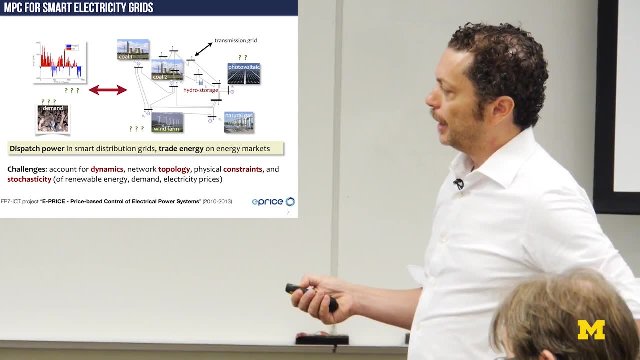 on a distribution grid And also how to trade energy on the auxiliary service market using MPC ideas. Here the problem is a bit different in type from the automotive or the aerospace problems, meaning that the dynamics is a larger scale and mainly because you have stochasticity heavily involved. 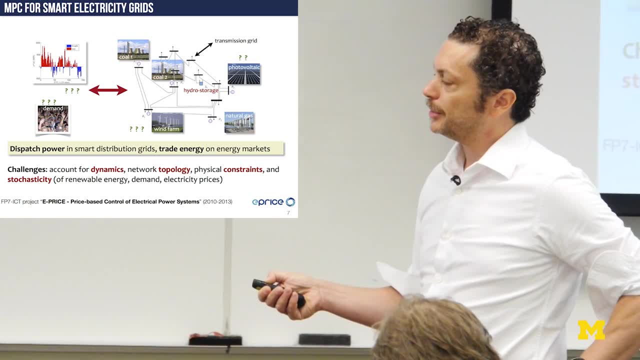 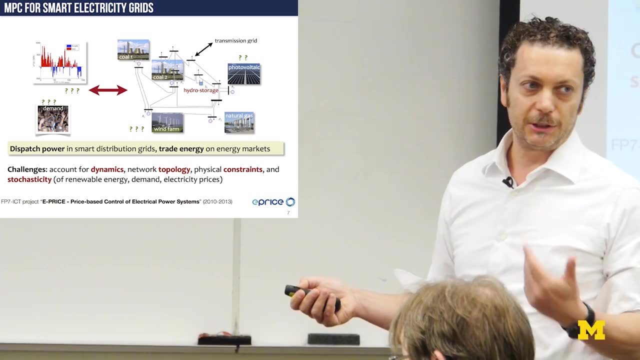 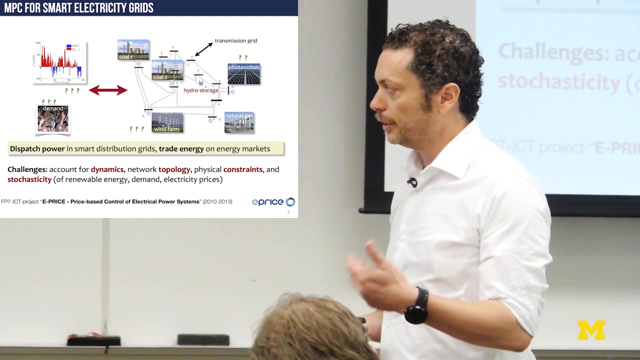 in the problem formulation. For example, in these type of problems, the energy price, the demand for energy from consumers and the amount of renewable energy that is available, those are all stochastic variables that you have to take into account to make a meaningful optimization. 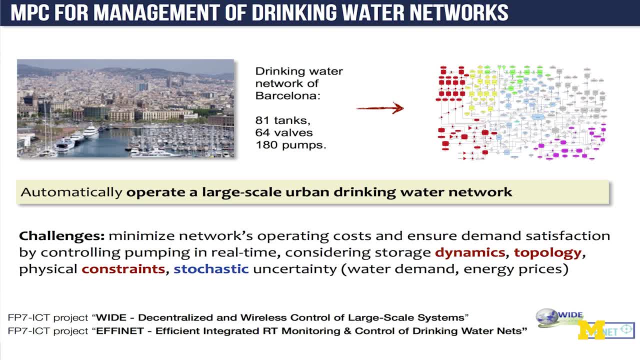 And similarly in another domain of control of drinking water networks. here you have a similar problem. It's not electricity flows, but it's water flows. What you need to optimize is mainly how to pump water in different places. This is out of a project we did together. 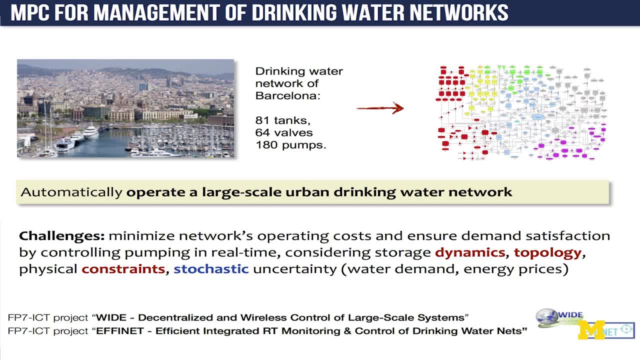 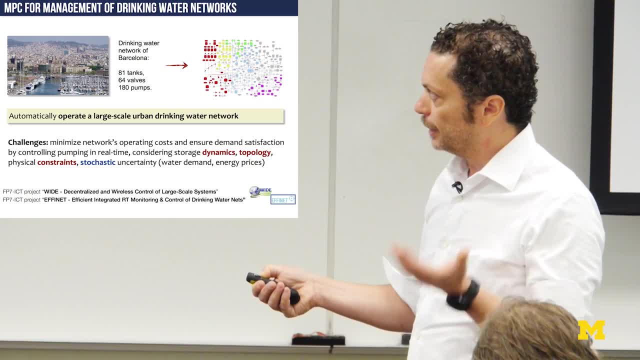 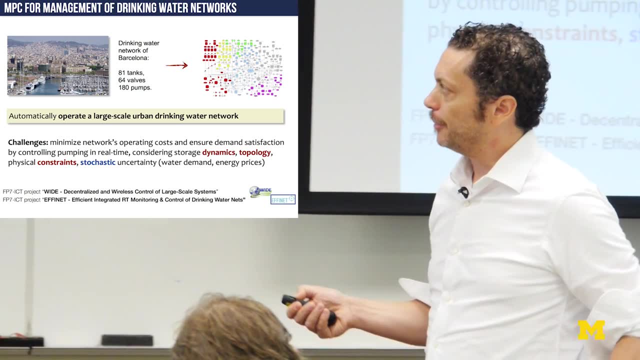 with the University of Barcelona and other partners, And the network is the network of the city of Barcelona. And you see, the system is quite large scale. It has 81 tanks, 64 valves, 80 pumps, so quite a large scale problem. 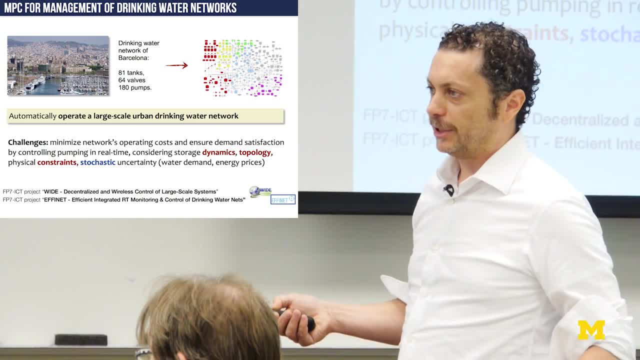 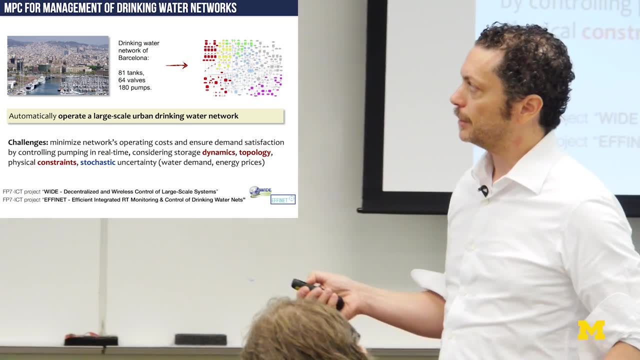 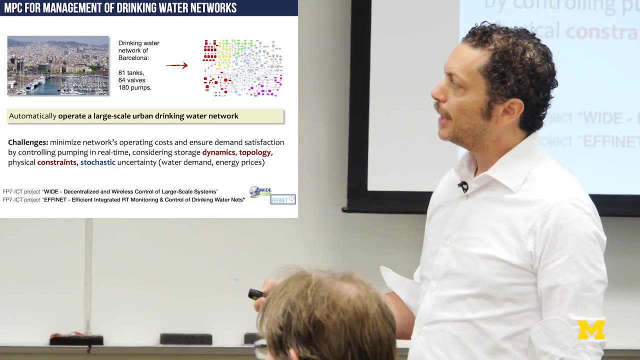 And here also you have uncertainty due to demand and also to energy prices for pumping. So what we have been doing is to apply, in this case, stochastic MPC formulations to solve this problem and to solve this efficiently, So to provide efficient ways in real time. 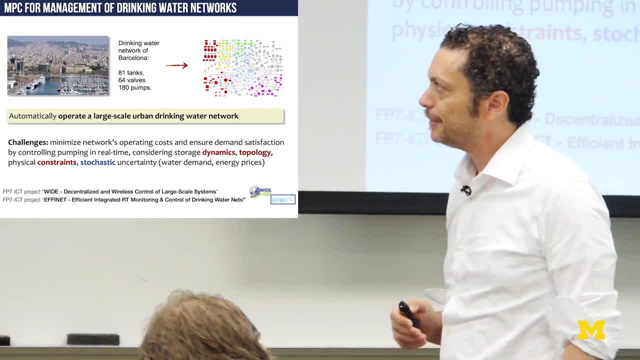 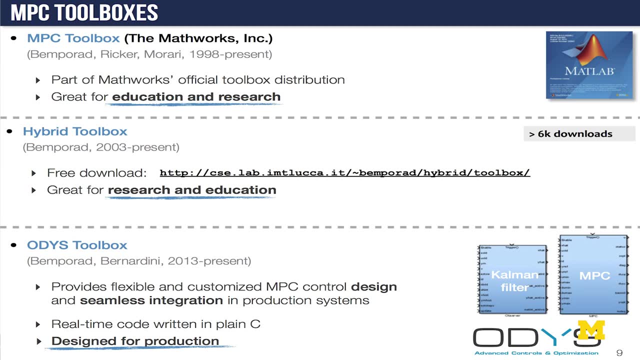 to decide how much water to pump from one part to another of the city. Now, all different applications and what they have in common is the theoretical background and also the tools that also Ida was mentioning before that are necessary if you want to be successful in applications. 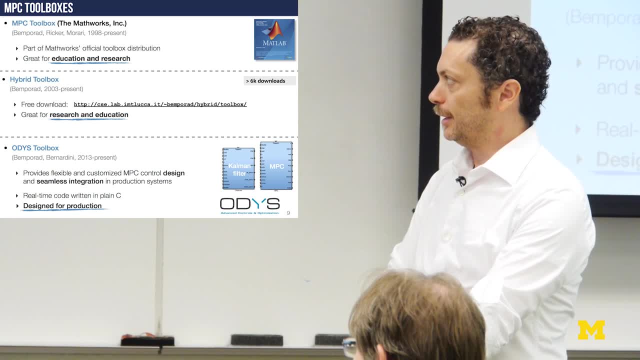 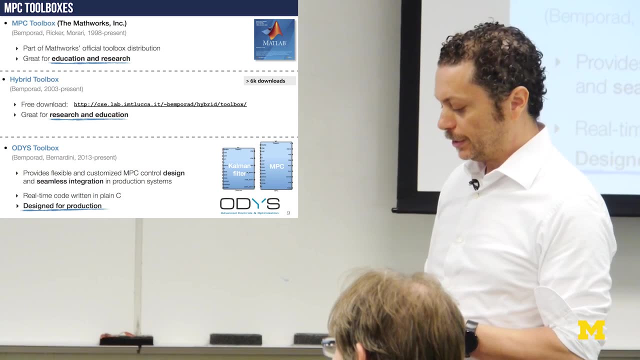 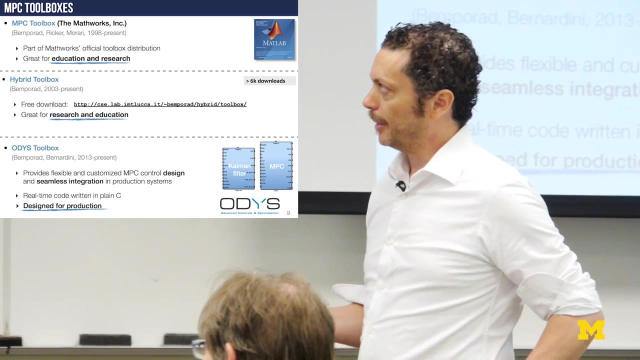 Without good toolboxes that help you formulating the control problem and doing simulation and also doing code development in case of real industrial applications. here I'm listing the ones I've been involved. The MPC toolbox is the one from the Matworks. You have the Matlab CD. 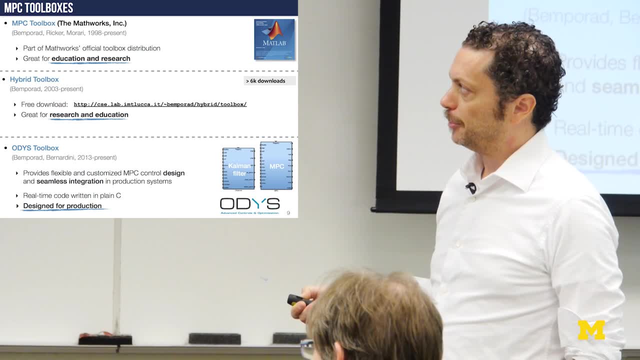 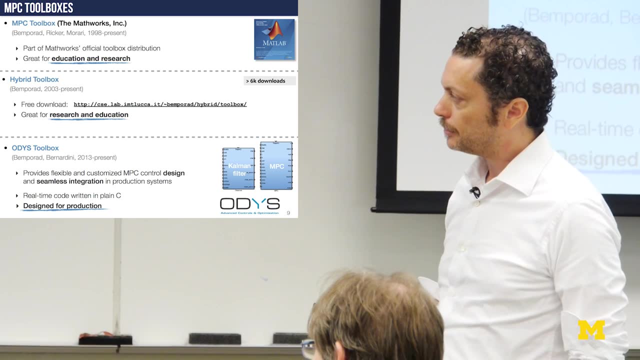 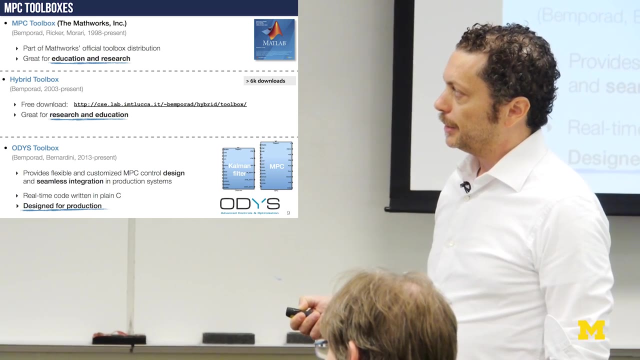 It does a lot of things for linear MPC and lately, linear parameter and time varying MPC. I think it's very good for education and also, to a certain extent, for research purposes. The hybrid toolbox I've been developing mainly for research, out of my research on hybrid model predictive control. 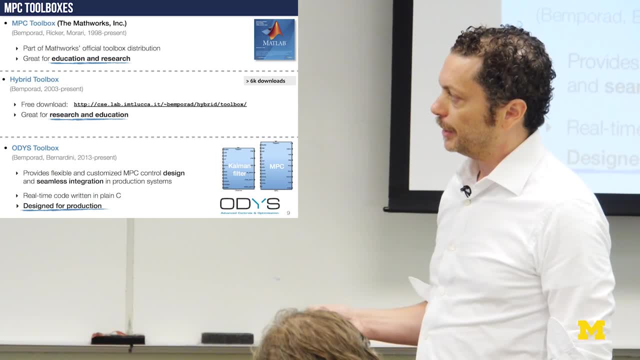 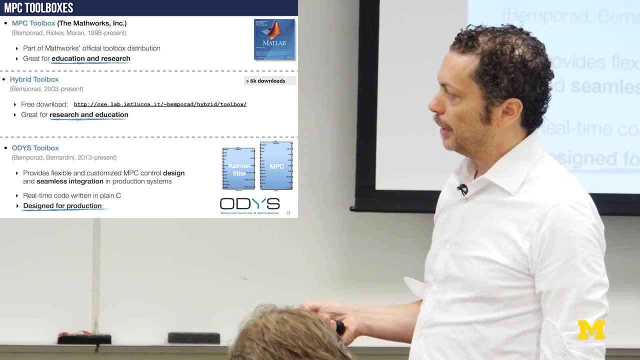 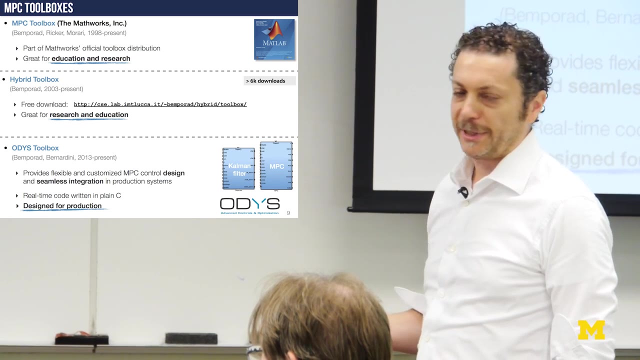 and explicit model predictive control, And lately I've been involved together with Daniele Bernardini with also recently with Jonathan Cimini, to develop a tool that has all the real time functions for MPC written in plain C And a Matlab environment around to do the design. 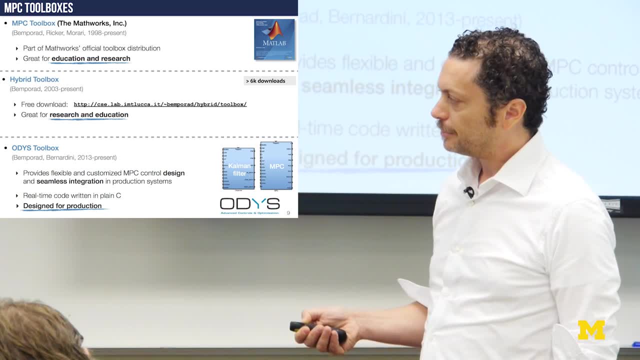 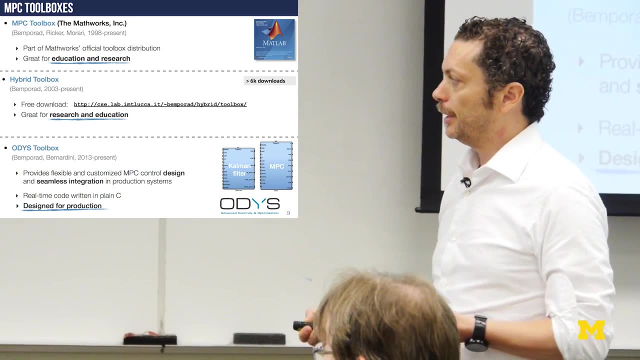 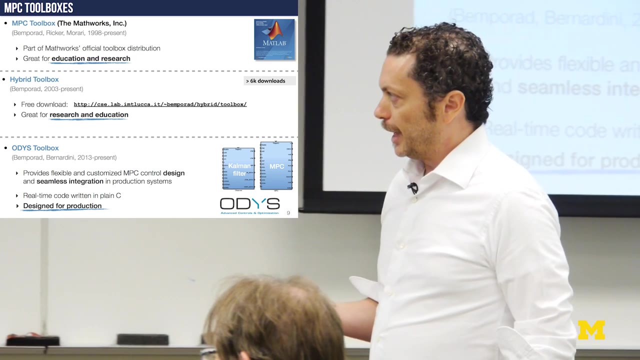 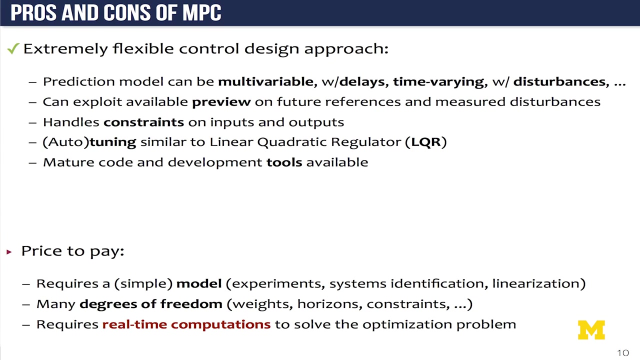 And the nice things about this tool is that it's really intended for production. So what you simulate in Matlab is the same code that actually you can deploy on the ECM of a vehicle, And so it's heavily optimized and very robust and efficient. So, pros and cons of MPC. 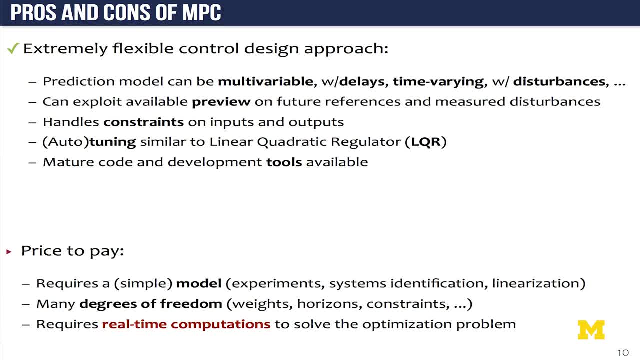 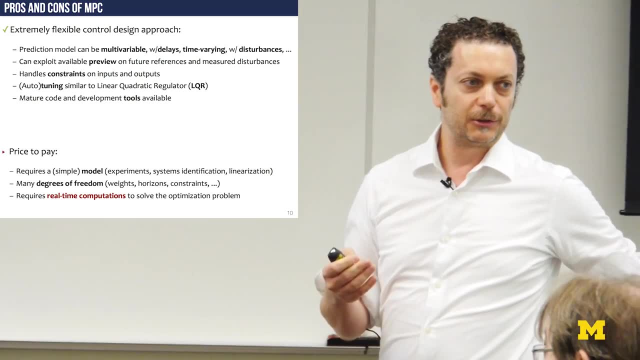 I think I gave you already the idea. It's a very flexible control strategy Because with the same control formulation you can deal with a lot of different type of dynamics. It doesn't matter how many input and output variables you have in the problem. 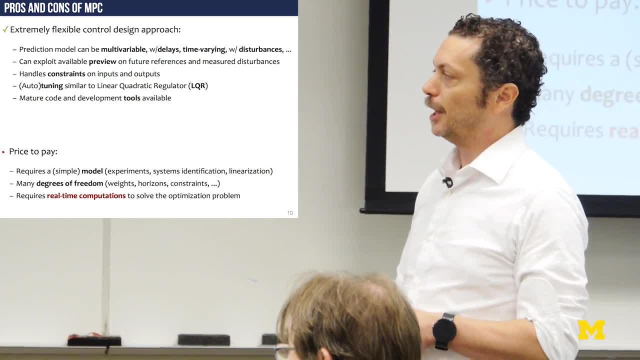 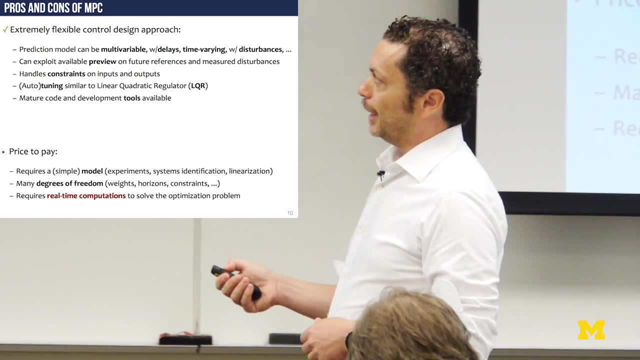 Could be single input, single output, Could be 100 input, 100 output. It's the same formulation And actually it's the same software. Of course the tuning is different. in that case You may have a little bit of a problem. 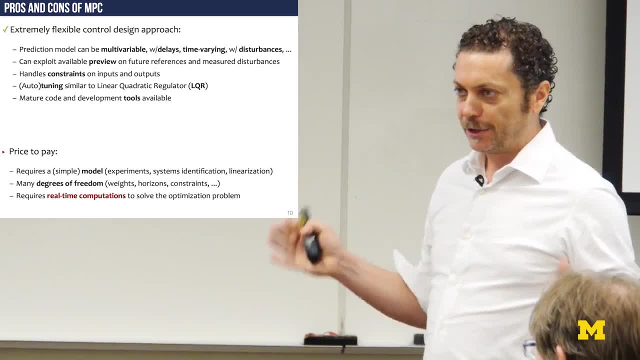 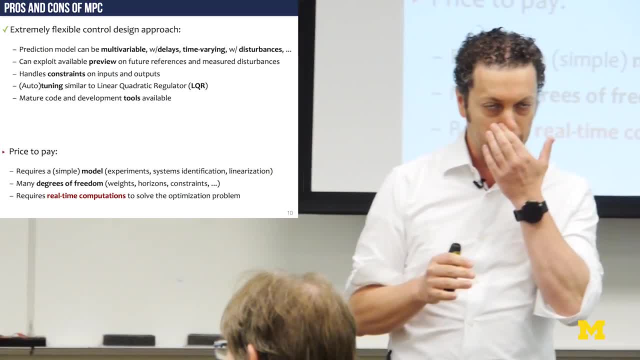 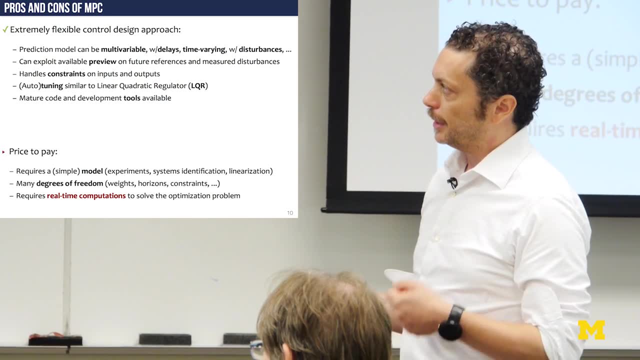 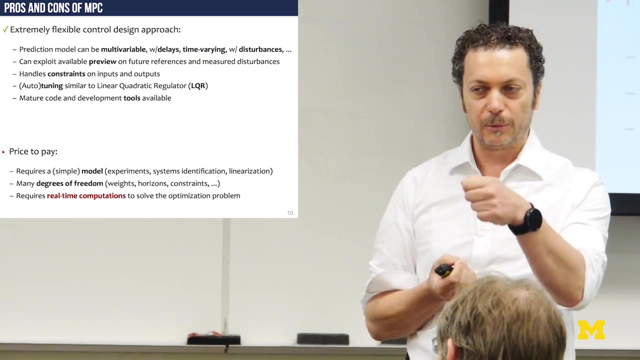 Everything can be fit in the formulation of a receding horizon optimal control problem, as I presented in the previous slide. Another nice feature of MPC, besides handling constraints, is also the ability to exploit preview. So if you know in advance what your reference signal will. 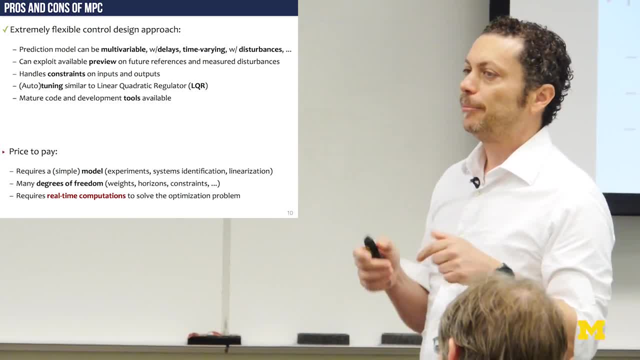 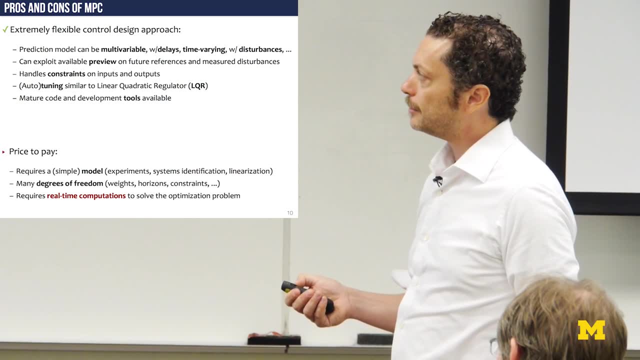 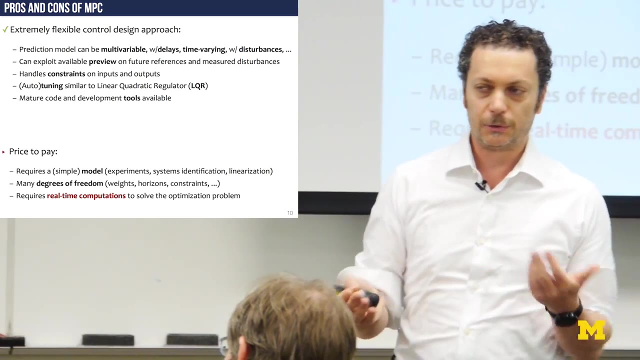 be of your measured disturbance signals will be. you can embed this information in the optimization and take advantage of this to improve your tracking. In terms of tuning, it's the cost function. Most cases it's a quadratic cost function, So you have to choose the weights. 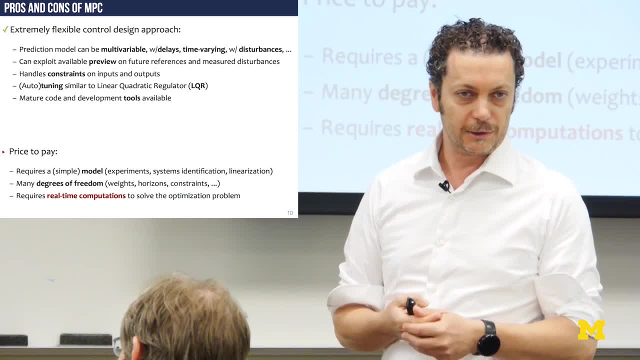 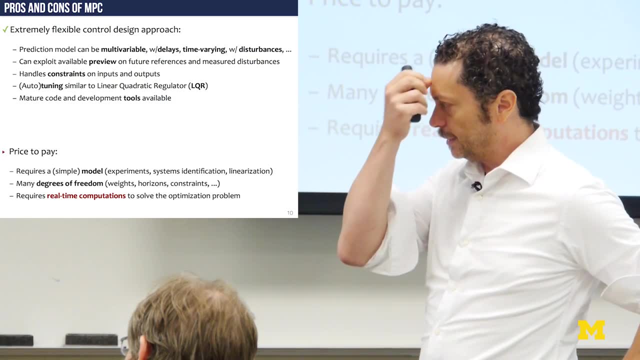 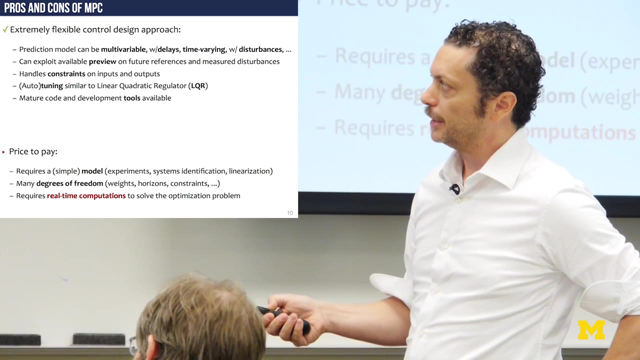 And this is the same operation that you do when you tune LQR LQG controller, So nothing different. And actually you can build auto-tuning tools based on global optimization on top of a simulation environment, so to automatically come up with a good set of weights and a good set of covariance matrices. 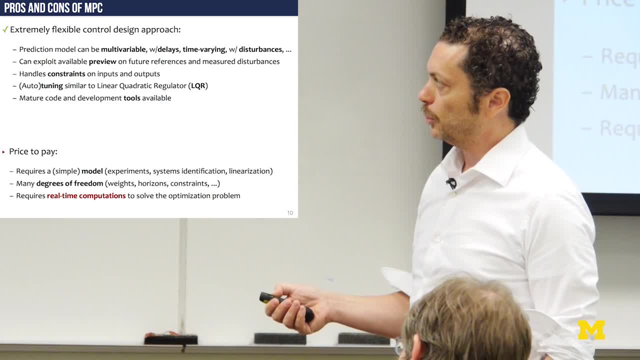 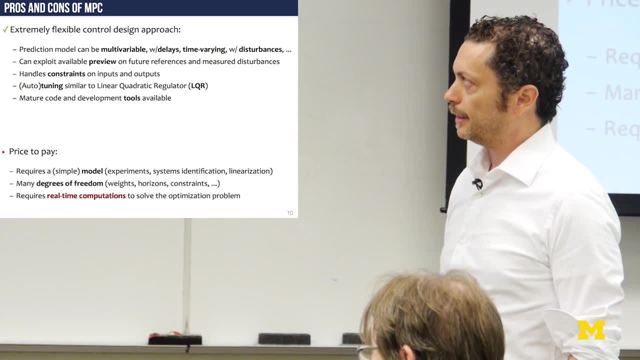 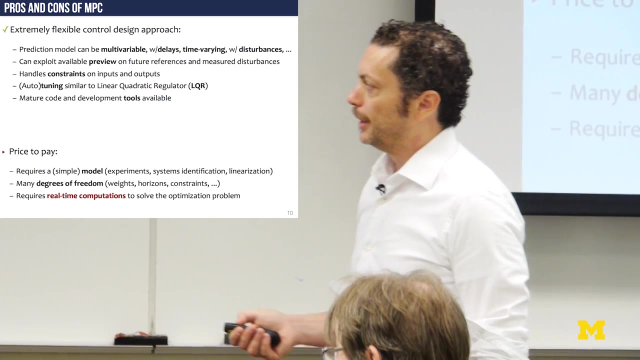 for the estimators that you use to close the loops. And the code is quite mature and the tools are quite mature, So this actually has become a technology. I would say Now, what's the price to pay? First of all, you need the model. 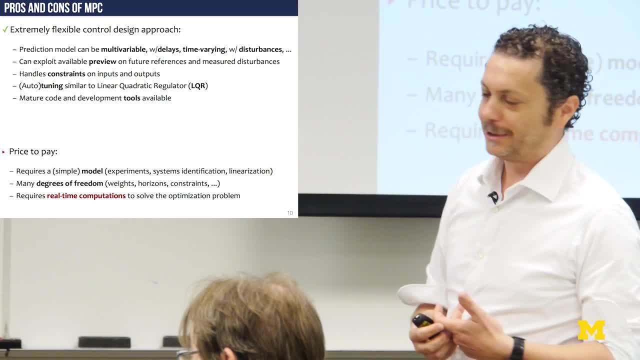 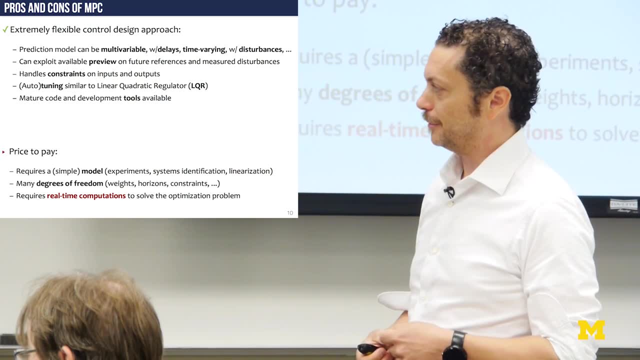 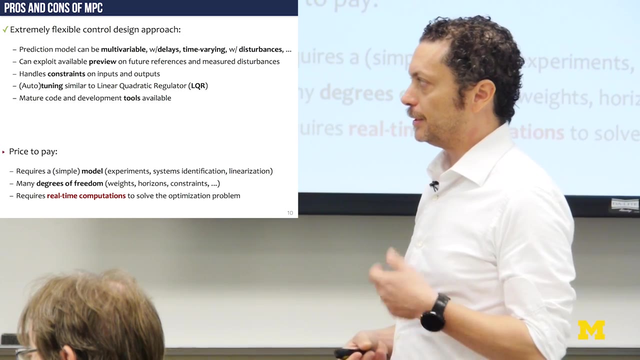 And this is as for all model-based control strategies. So you need a model, And that means that you need to spend time- And usually most of the time is spent there- to figure out what a good model for making prediction is. that involves running experiments. 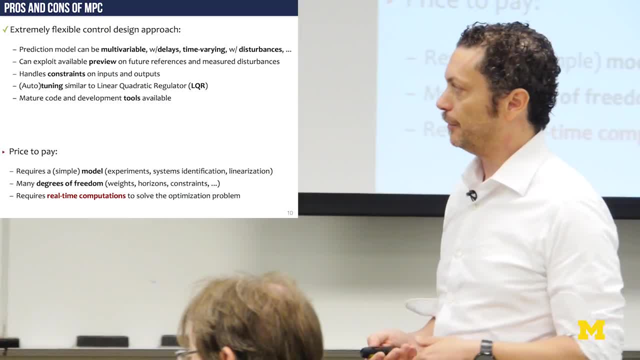 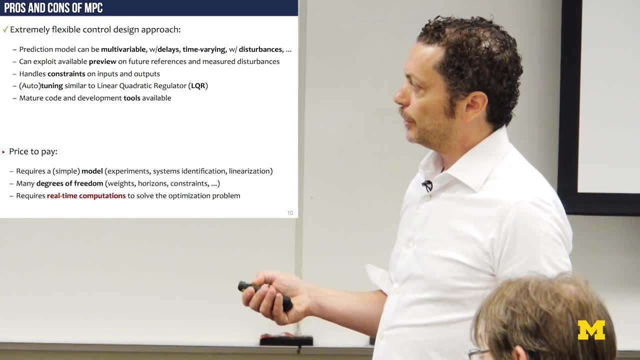 doing system identification or linearizing the linear models, And this can be very time consuming. compared to model-free techniques, You may have many degrees of freedom, the weights, But also you have to choose the constraints, the prediction horizon, So you have much more flexibility. 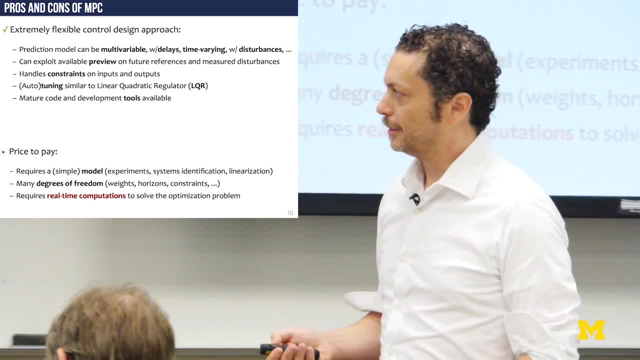 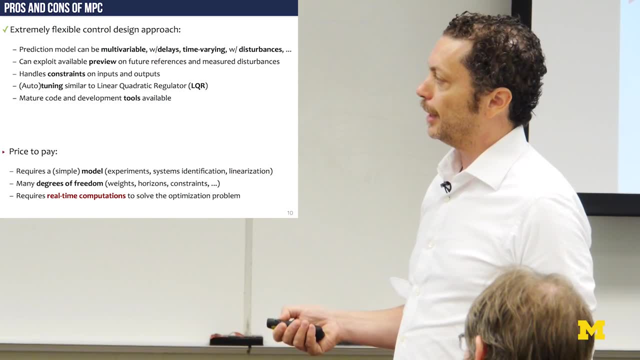 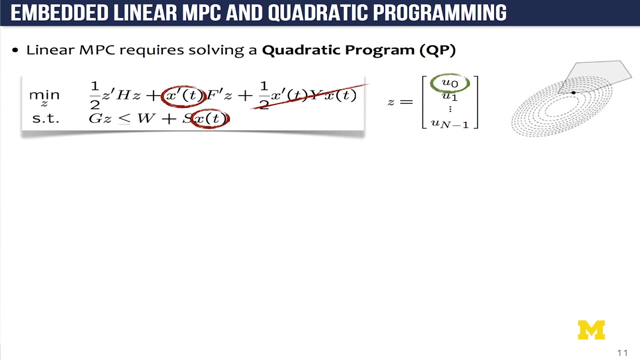 which is a good thing, but is also a bad thing from the tuning point of view. And, last but not least, is the computations that are involved to implement the control law. So you have to solve the optimal control problem in real time. 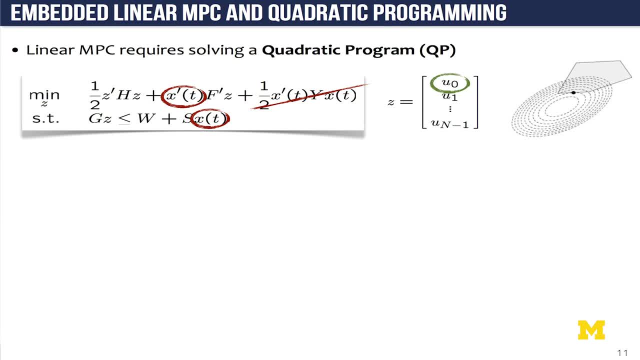 What is the optimal control problem you need to solve? If you use linear models, which is quite often the case, if not always the case, in all industrial applications, the optimal control problem can be mapped into a quadratic program. So the quadratic program, so the problem. 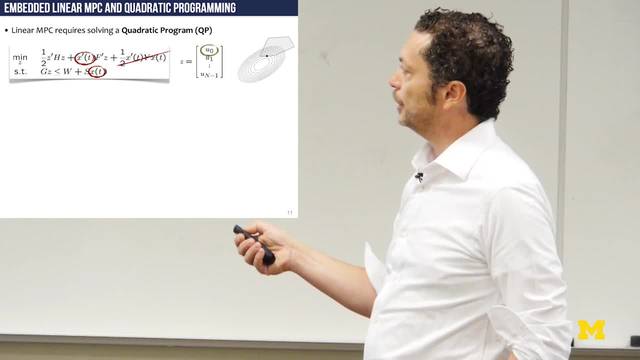 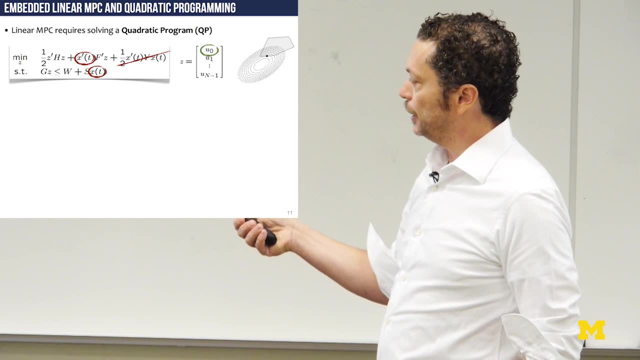 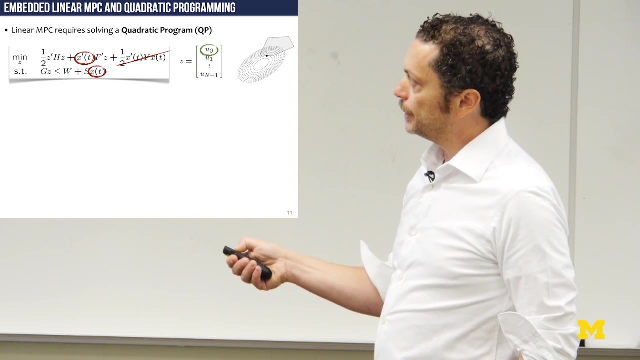 of minimizing a quadratic function subject to linear constraints that define a polyhedron where the solution should lie. Here's the optimization vector. Again, it's the sequence of future inputs you need to choose. If you use linear time invariant prediction models, the QP has this type of form, where the Hessian matrix 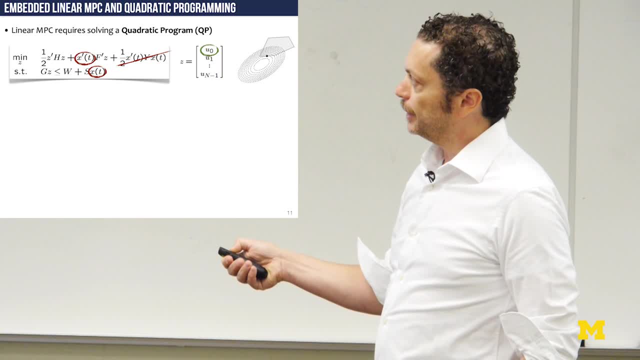 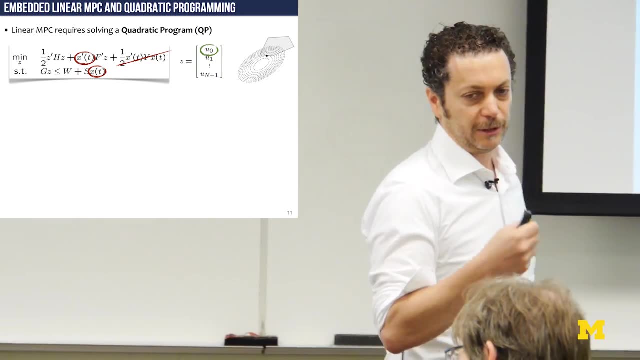 and the left-hand side of the constraints are constant matrix, But the linear term of the cost function and the right-hand side of the constraints change depending on the value of the state vector and, more generally, the value of the state vector and the reference signals. 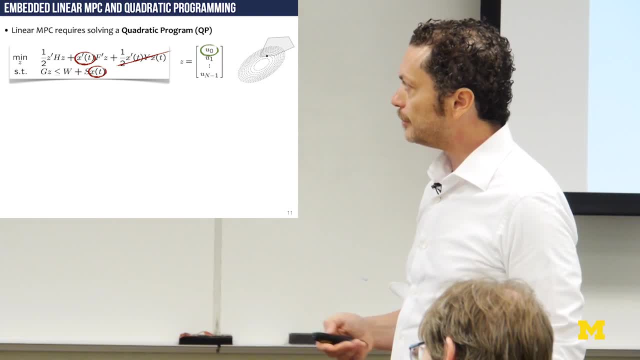 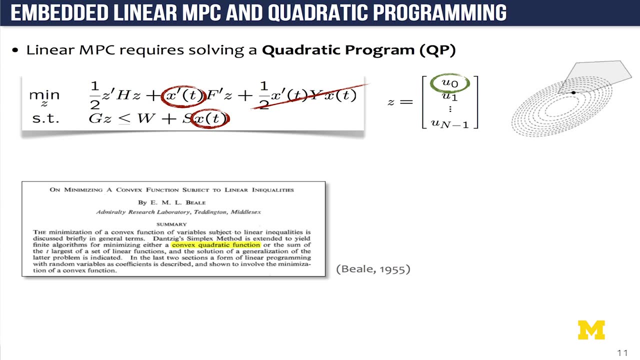 and everything that changes in real time. Now how to solve the QP. This is also a very old problem. If you look into the literature, probably one of the first papers dates back to 55. So it has a long history. 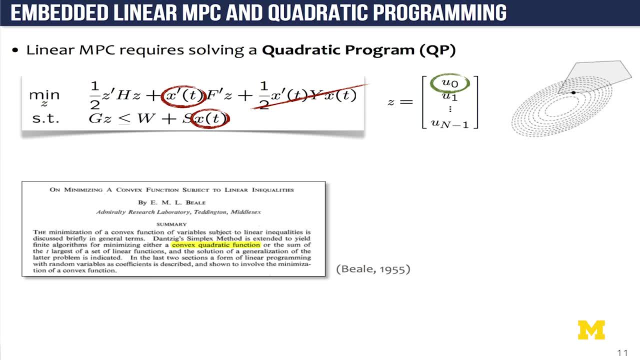 It started in management science And it's applied in tons of different applications in many different disciplines, not just in control. So today, after so many years, if you look in the literature and books, there is a very rich set of algorithms and solvers. 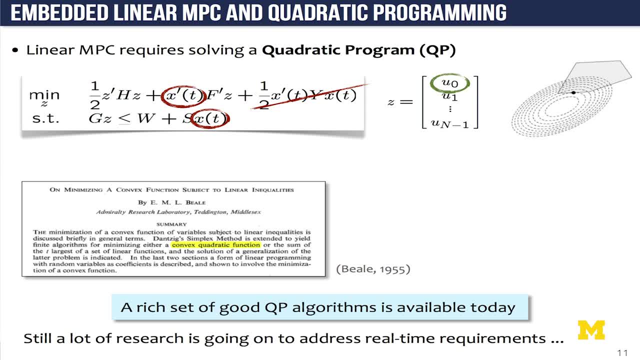 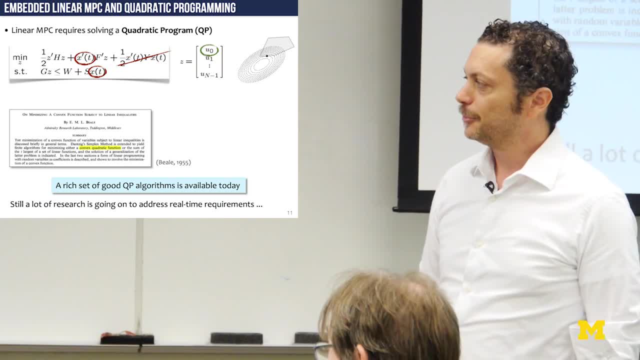 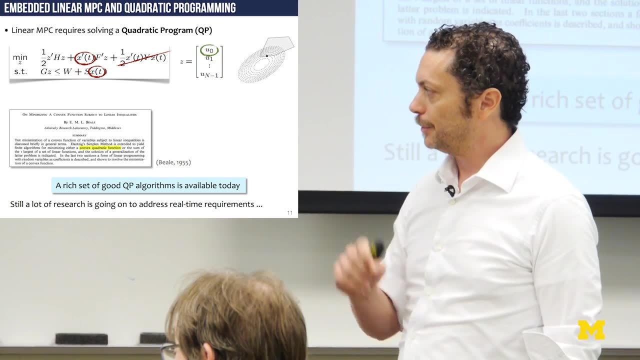 that you can choose from and use, And these actually are pretty well understood and studied And they're efficient. Still, the story's not over, because there is a lot of research going on to come up with QP solvers, And I will show you some recent things that we have been doing. 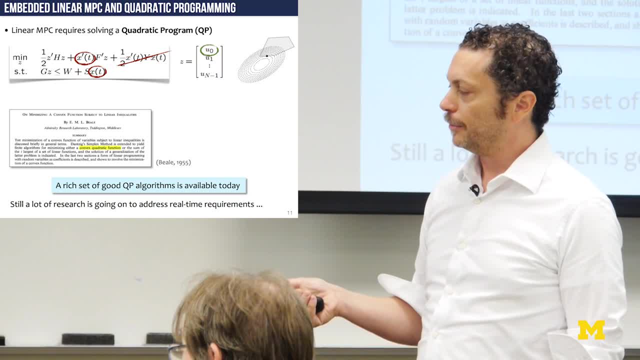 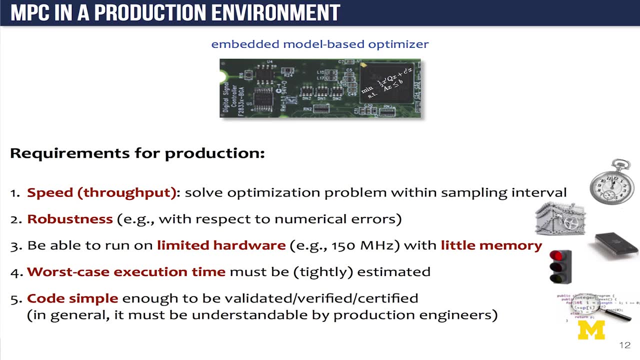 So to meet real time requirements, where, when the QP solver doesn't run just offline but must run on a platform. What are these requirements Here, I think? what, in my opinion, are the main ones? Well, speed, of course, or throughput of the controller. 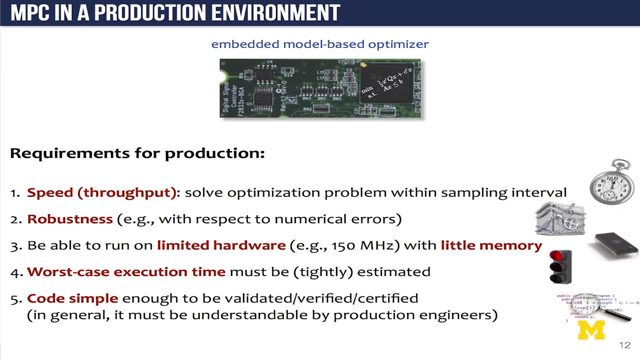 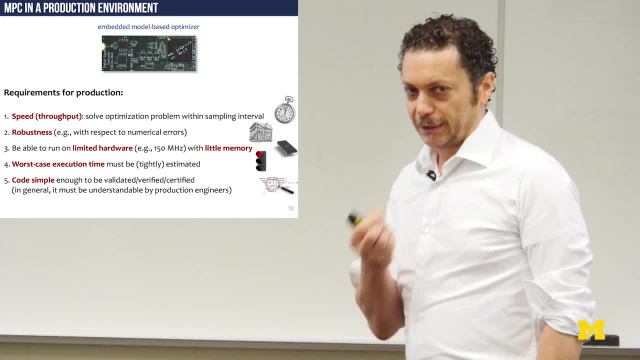 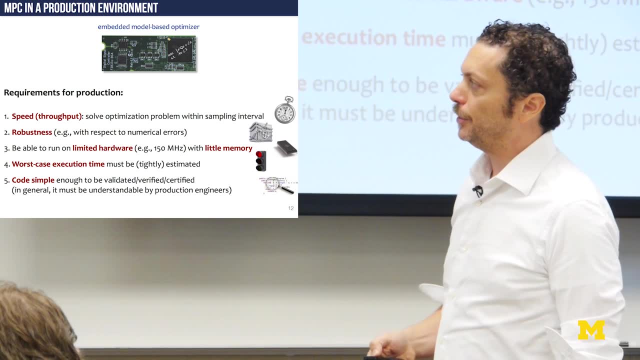 You want to make sure that your solver is fast enough to deliver solution within the sampling interval. That's minimum requirement. But also you want to have robustness, So if this has to run autonomously, say on a vehicle, in real time, without any supervision, 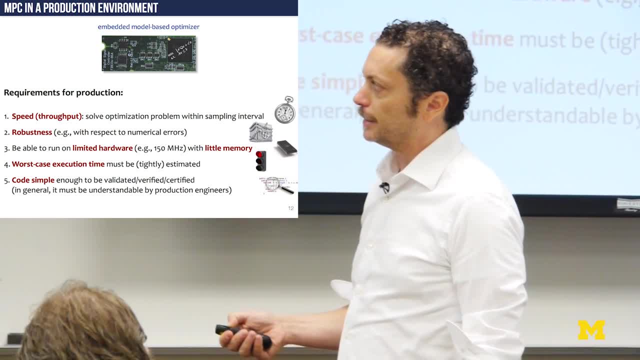 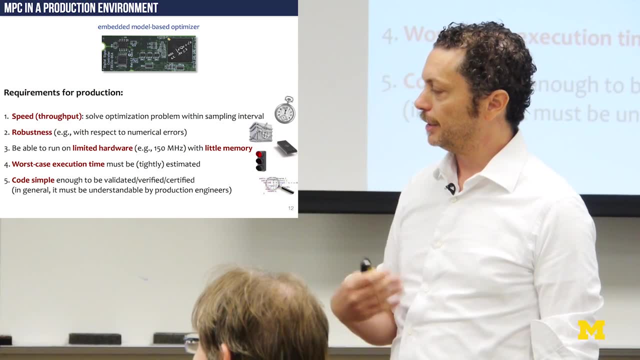 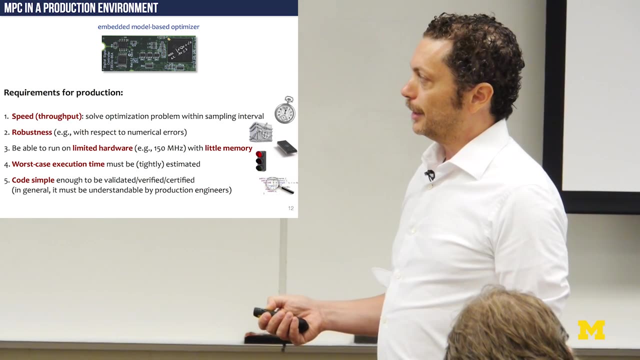 this must be robust. It doesn't have, it cannot fail, And Especially must be robust with respect to numerical errors. Most of the time the code is implemented in single procedure or even fixed point precision. Then also usually you don't have much hardware richness. 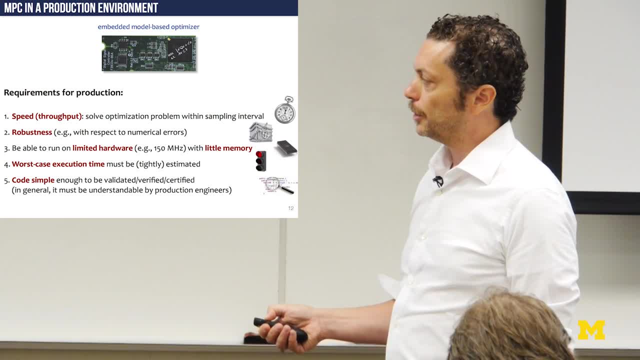 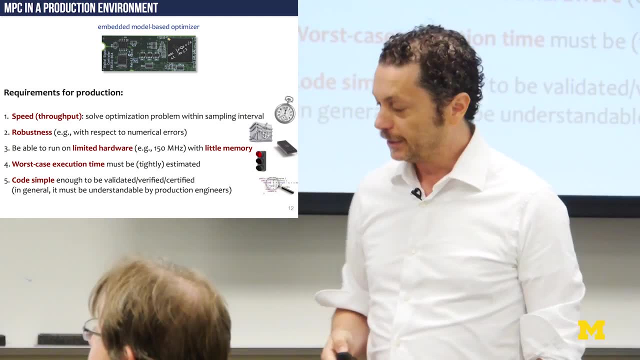 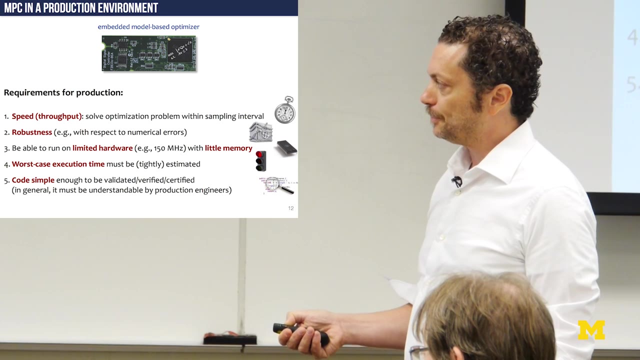 at your disposal. Many cases you have to work with CPUs which are in this order of magnitude And also with little memory- say a few tenths of kilobytes- And the other requirement is that You need to estimate what is the worst case execution time. 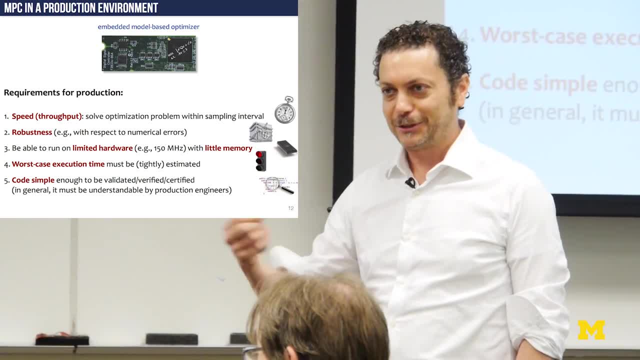 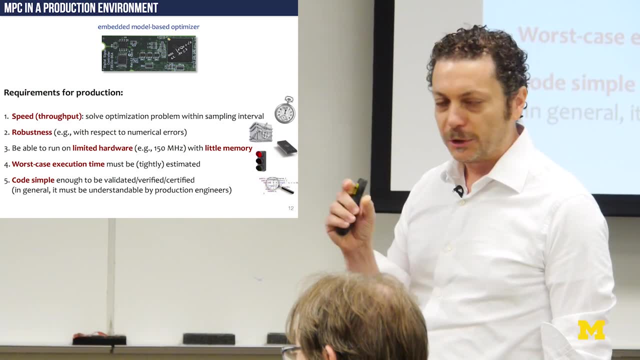 It doesn't really matter what is the average time- OK, it matters if you run simulation, So that will speed up your simulation, But to be executed in real time, what you care of is the worst case execution time, So your controller must be able to provide. 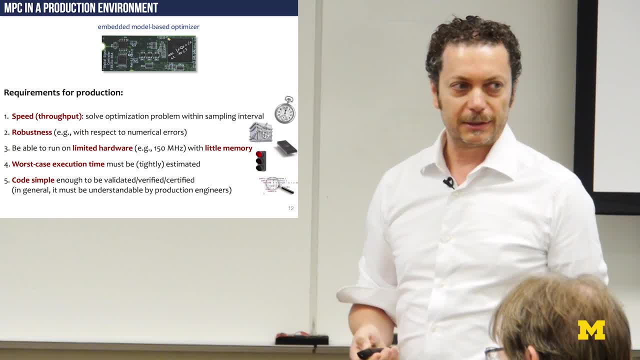 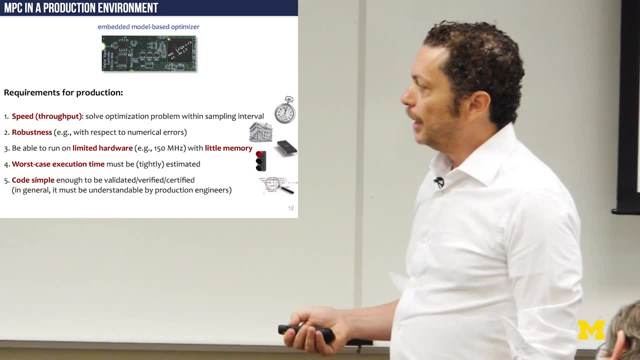 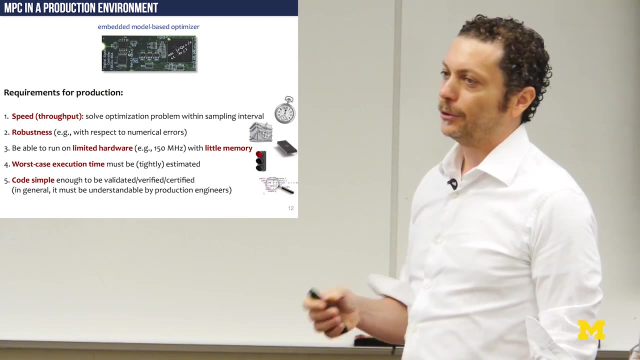 a solution within the sampling interval in the worst case. So you need to have a solver for which you are able to estimate the worst case execution time And the last. these are more. if you want an implementation or also a psychological requirement, The code should be simple. 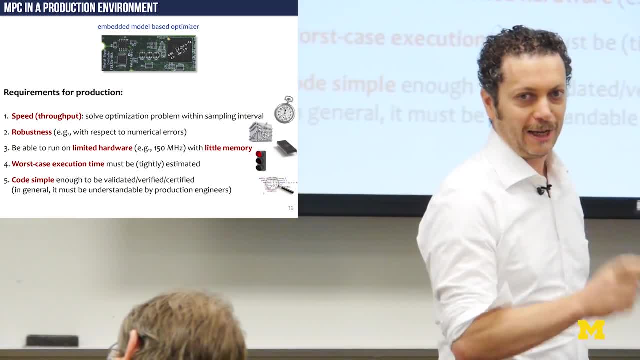 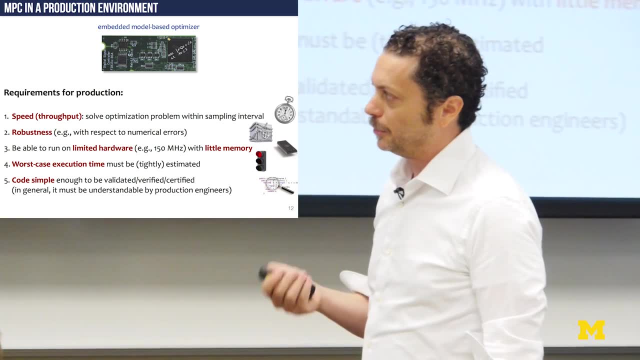 If you have very good algorithm but it's very complicated, 10,000 lines of C code, then it's hardly implementable because people will be very skeptical. And there are good reasons for that. actually, Because many cases you want to validate the code. 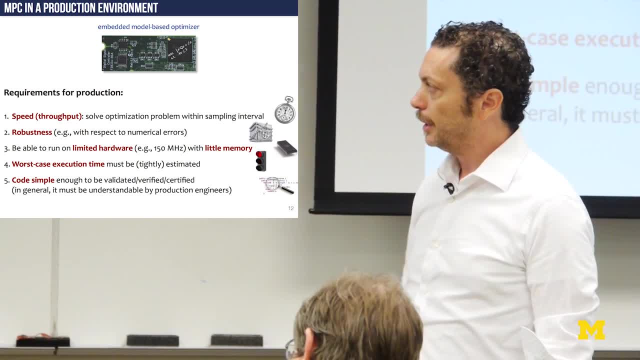 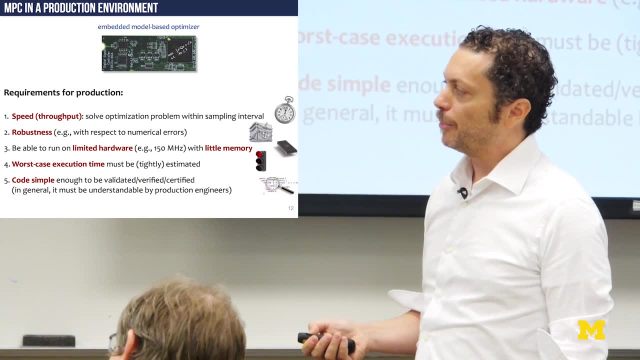 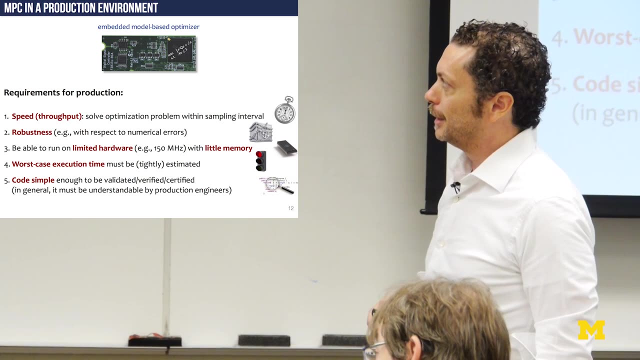 and certify the code. I mean software certification of the code- And, for example, in aerospace application, this is a very severe requirement, So you have to come up with algorithms that are relatively simple to code. OK, let's keep in mind these requirements. 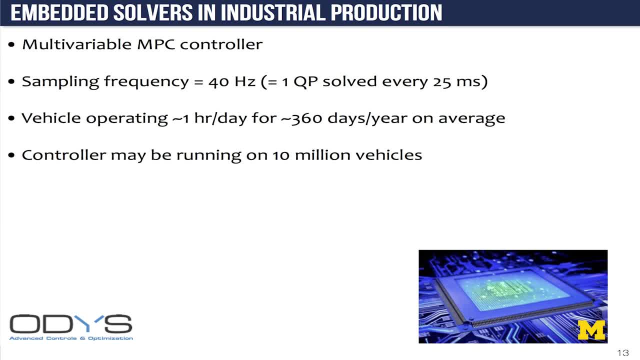 Now I want to show you some, actually an example, coming from real work we have been doing with those. I cannot tell you the details for confidentiality reasons, But just to give you an idea of the sites and the importance of this requirement. OK, 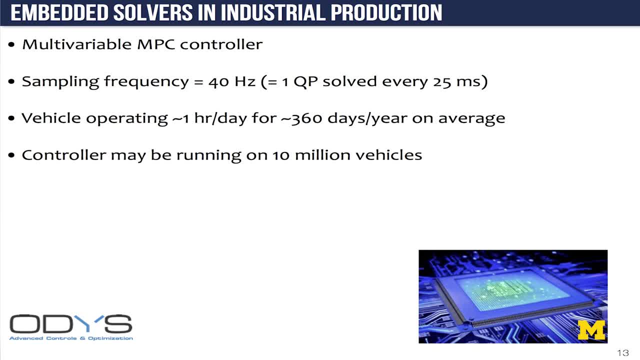 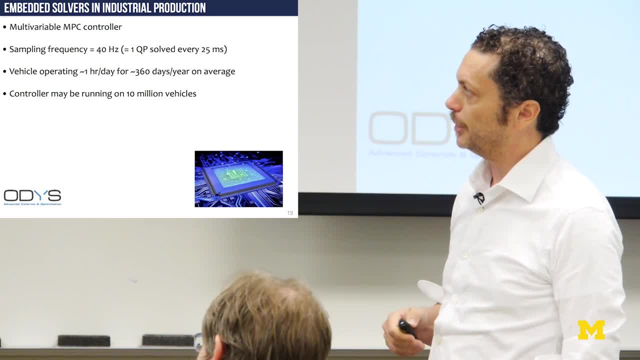 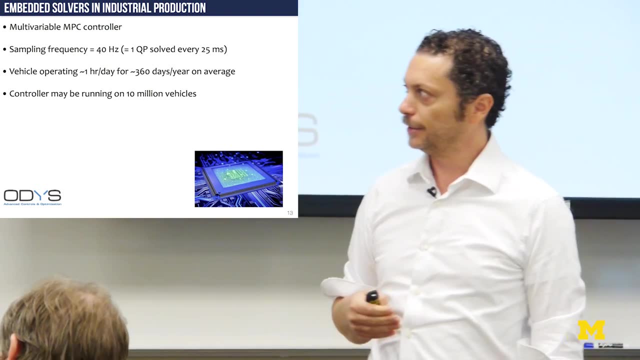 OK, So you have multivariable MPC controller that has to run every is running at 40 hertz, So you have to deliver a QP solution every 25 milliseconds And say this goes on a vehicle that operates on average one hour per day over 360 days. 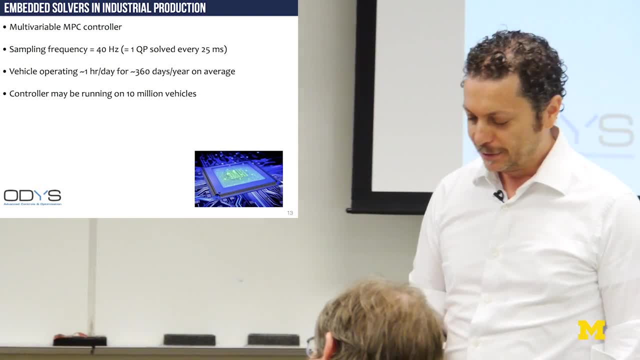 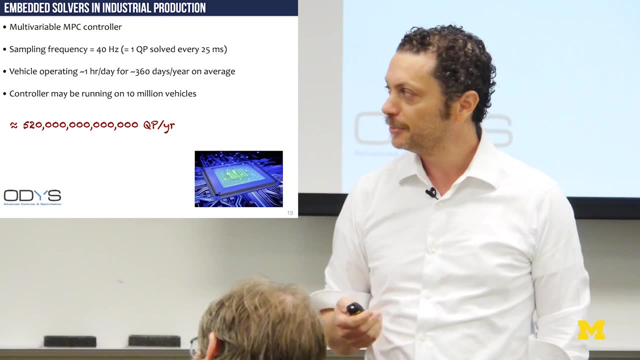 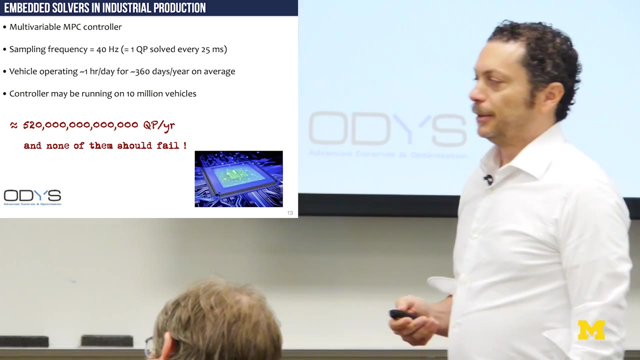 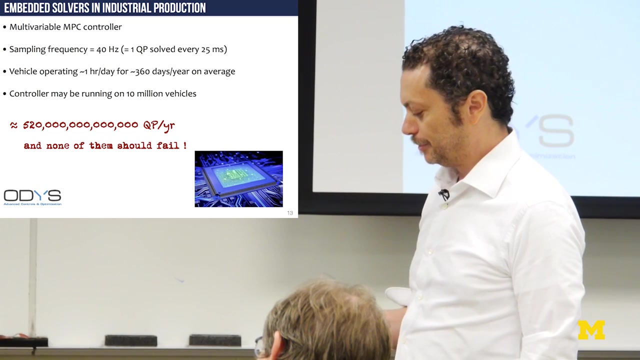 And let's say this may be running on 10 million vehicles. Now, if you do the math, this means that you have to solve half quadrillion QPs per year And no one of these QPs should fail Right. So that this is: it's able to run on a vehicle. 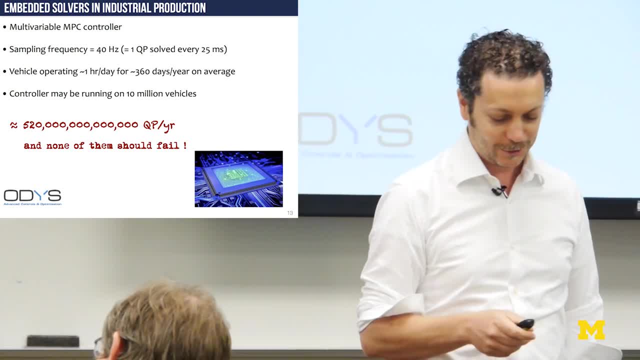 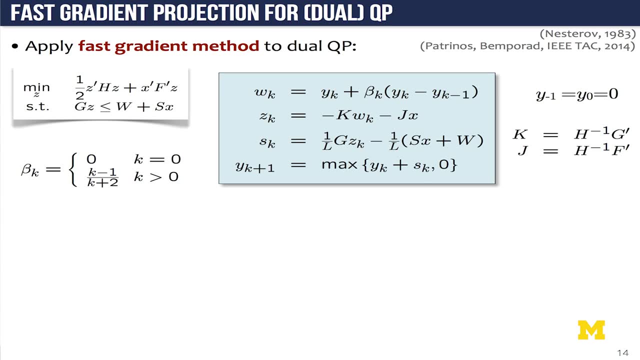 So that puts a little bit of pressure on us to develop the algorithm and write the code. I want to start with a solver that we developed together with Panagiotis Patrinos in Luca A few years ago To address these requirements that I 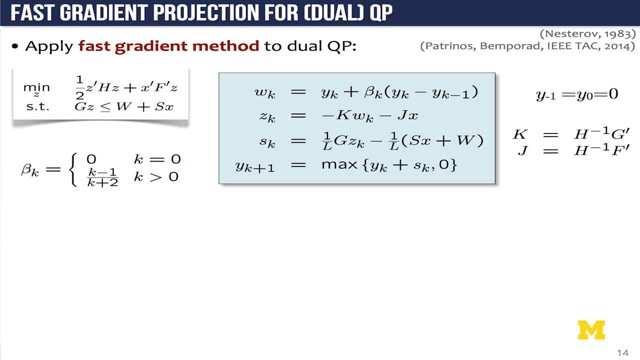 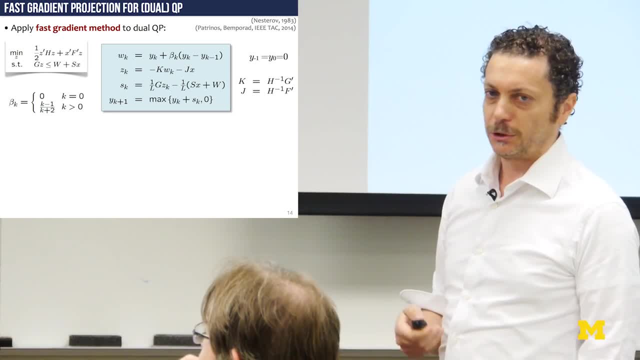 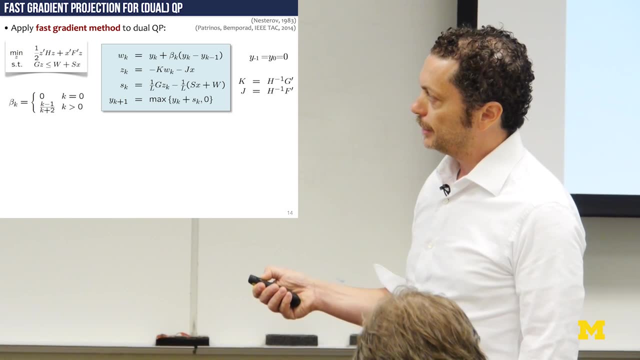 was listing in my previous slides. So to come up with a QP solver that is simple, it's fast enough and is worst case. execution time can be estimated quite well. So here is the solver. Actually, the whole solver is listed here. 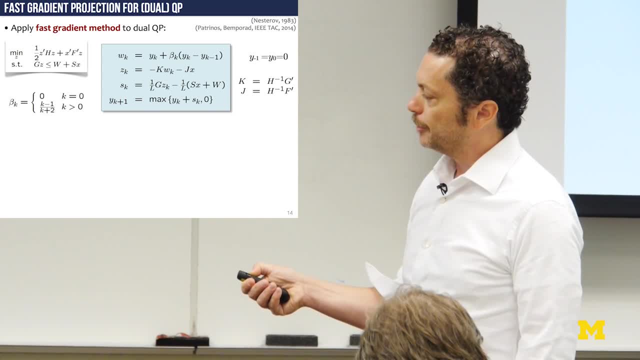 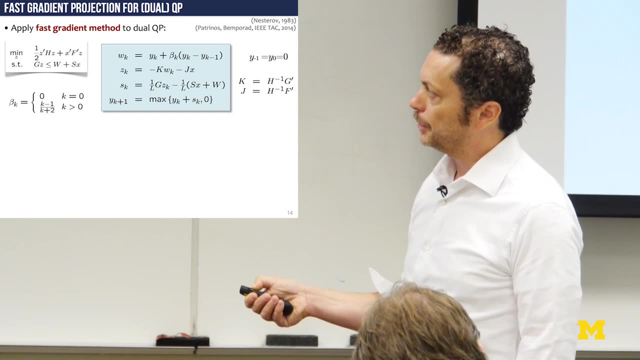 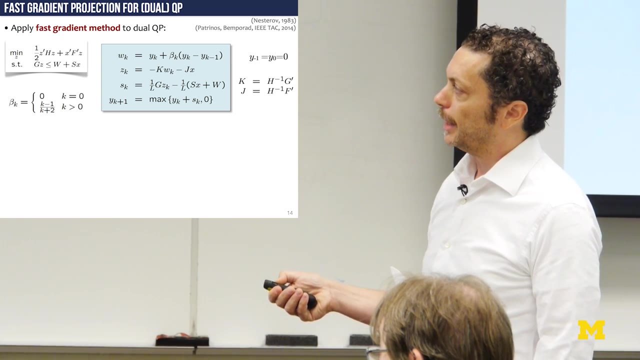 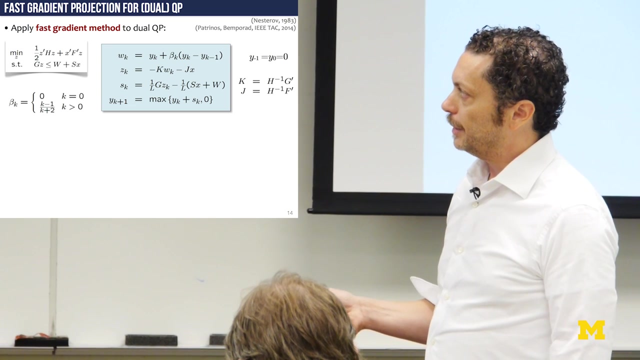 It's a bunch of Matrix, vector multiplication and max. This is an algorithm that actually is the gradient projection algorithm in its accelerated form due to Nesserov, applied and specialized for the dual of the QP problem that you need to solve. So very, very simple algorithm. 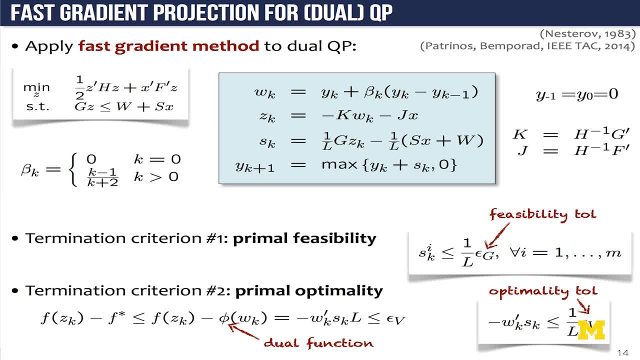 Also, checking when you should terminate the iterations is also quite simple. You have to look at these variables, whether they are within a certain feasibility tolerance. in terms of feasibility And in terms of optimality, you can estimate the distance from the optimum by looking at the duality gap. 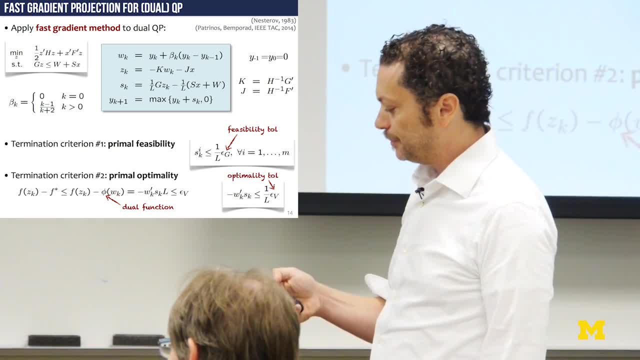 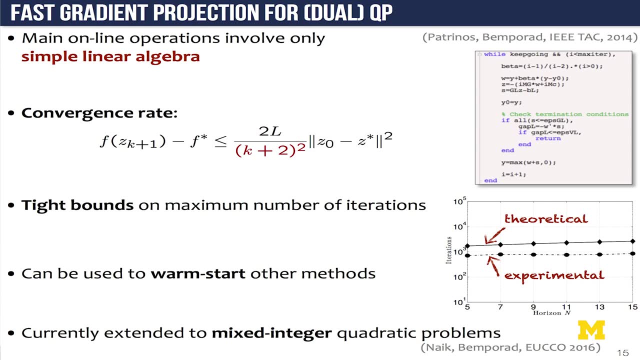 And this can be also easily computed by a scalar product. So this is actually the code written in embedded MATLAB that solves the QP. So extremely simple. And the convergence rate: it's a first order method, It's not too fast. It has a convergence rate of 1 over k squared. 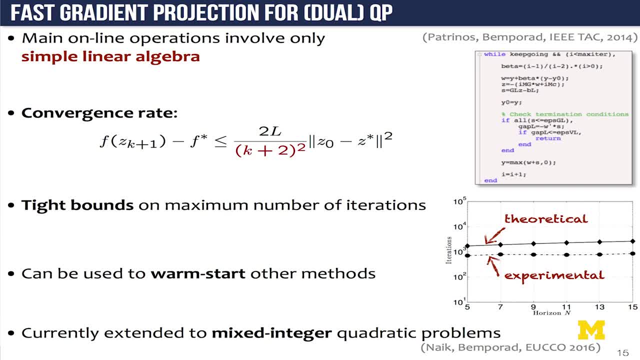 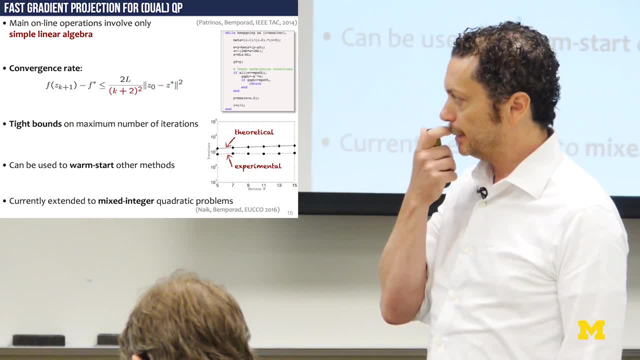 The good thing about this algorithm is that you can estimate the worst case execution time by deriving theoretical bounds, which turn out to be quite tight in many cases. So if your bounds, if your theoretical bounds are good enough for your application, you are all set. 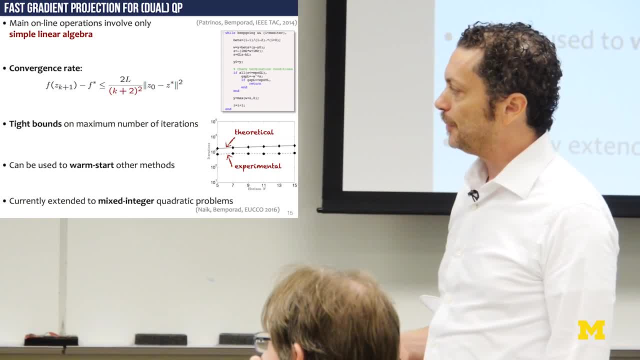 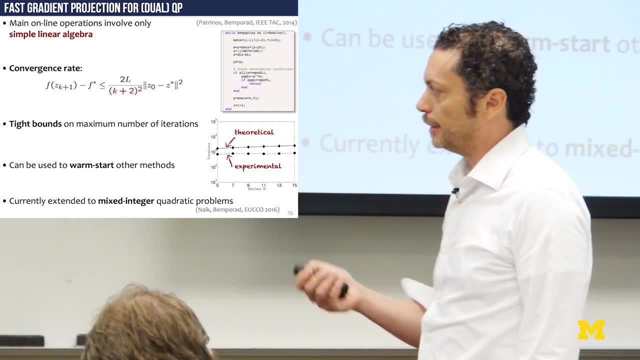 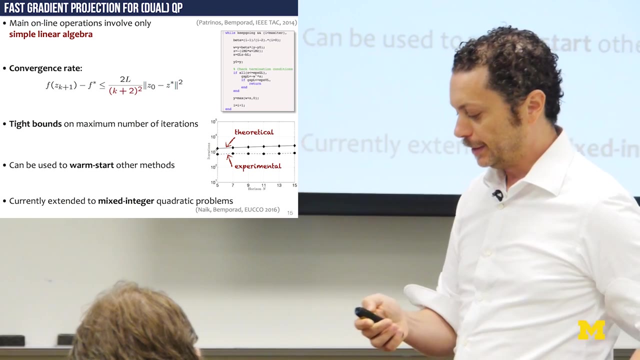 You can implement this even in the production system And we are currently extending this solver Solver to solve mixed integer quadratic programs, together with my student behind me, using the same algorithm but within a branch and bound setting, exploiting more or less smartly the bounds. 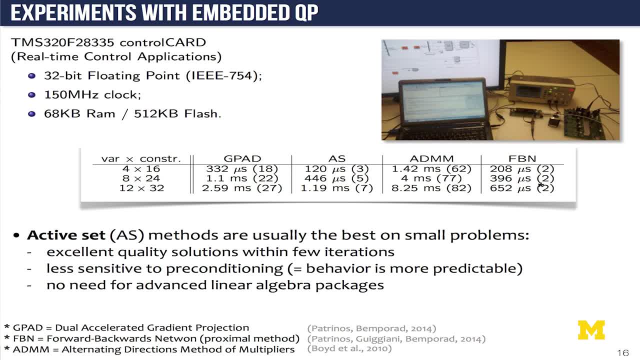 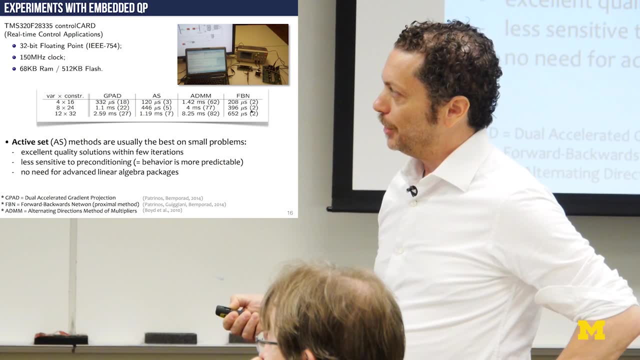 This is to give you some numbers of solving QP problems on a platform that actually Jonathan was- you right, Jonathan- who worked out this. This is the size of the QP, So small QPs- that's typically what you have in small MPC application- fast MPC. 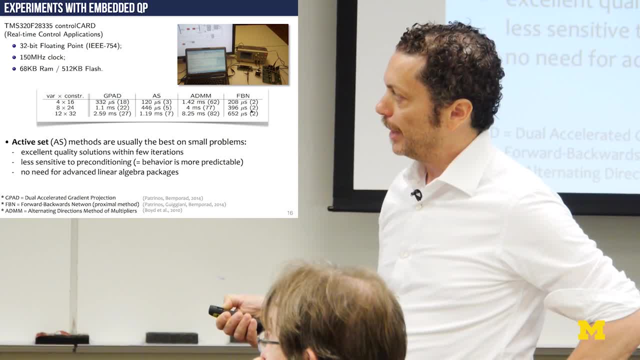 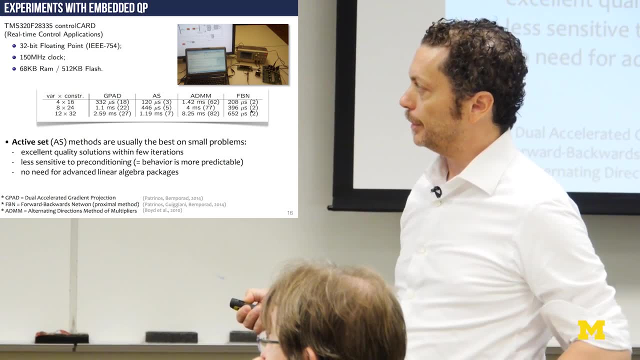 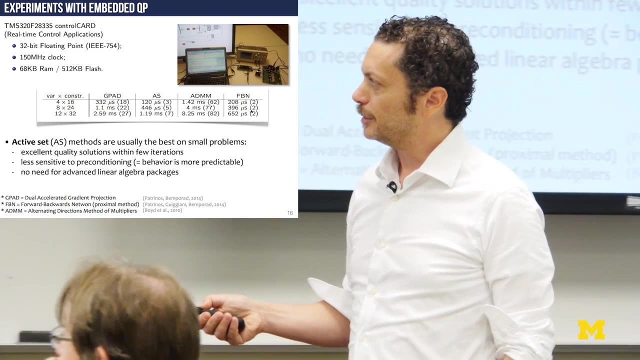 applications using different solver. the gradient projection method on the dual, an active set method. ADMM is also another popular simple solver that can be used in application, although the worst case execution time with ADMM is more critical. So you have to estimate, even if you do proper scaling. 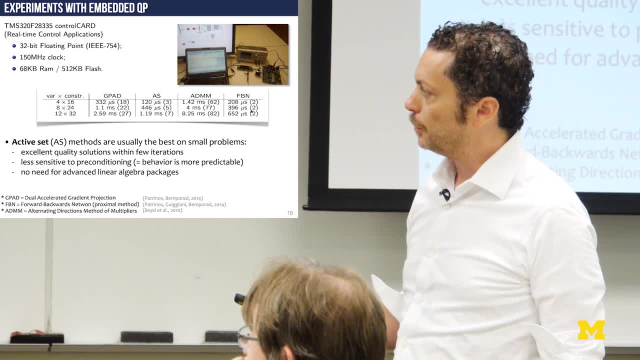 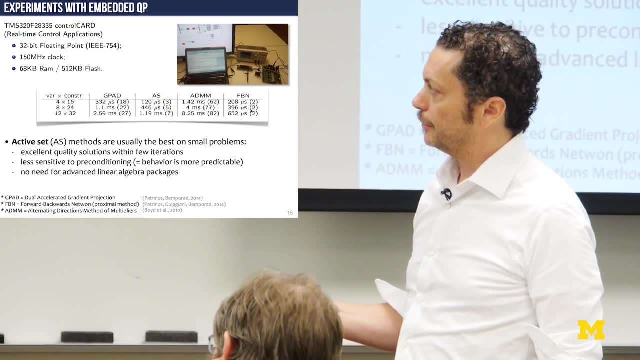 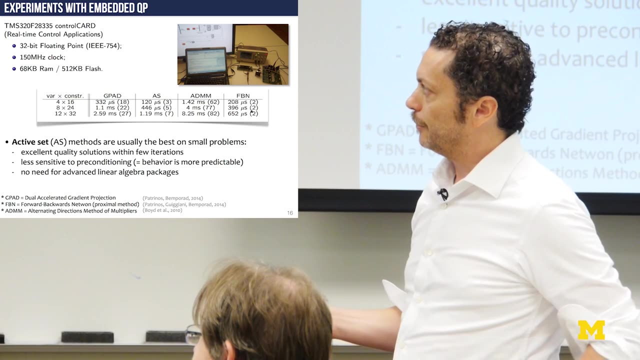 of the problem matrix And for backward Newton method, it's another method that was developed by Panos Patrinos and Alberto Guigiani and myself back in Luca, which is a Newton method applied on the envelope function associated with the problem. So this is the rightfully the order of magnitude. 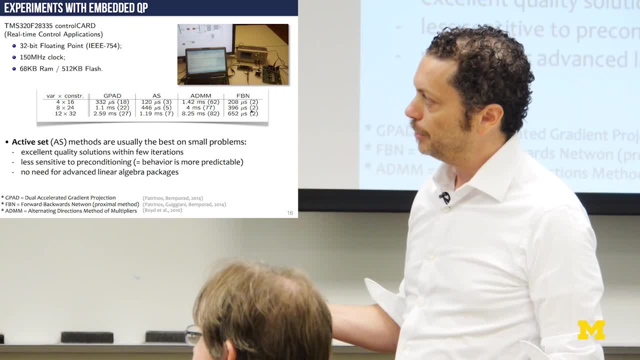 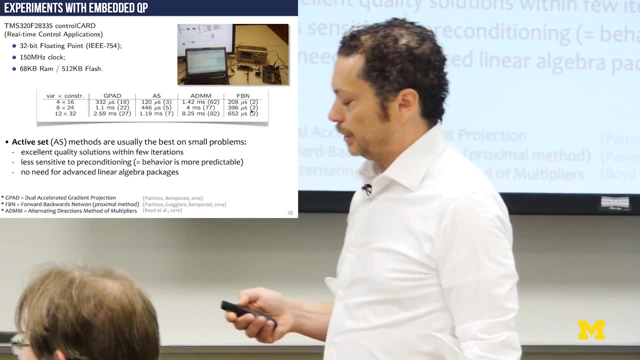 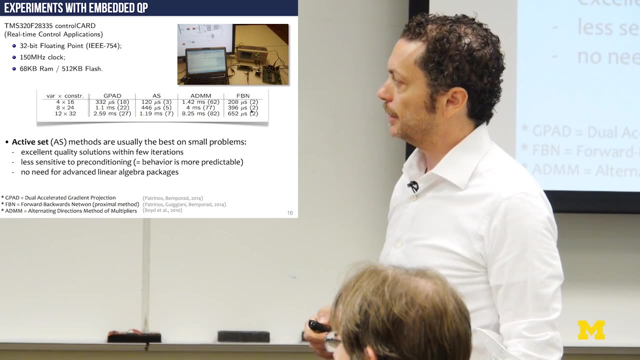 So you can solve on this platform And this QP size in about, say, in the order of 1 millisecond. So just to give you such an estimate, And these are comparable active set actually turn out to be for this type of small scale, dense problem. 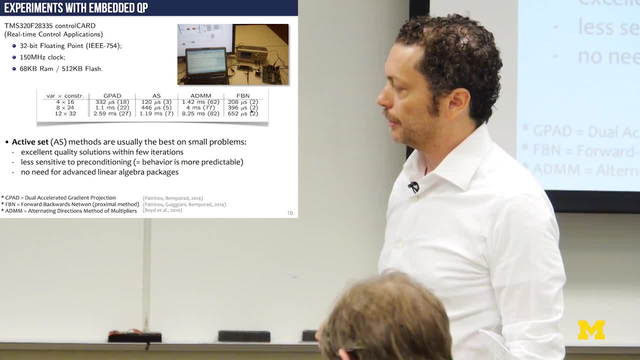 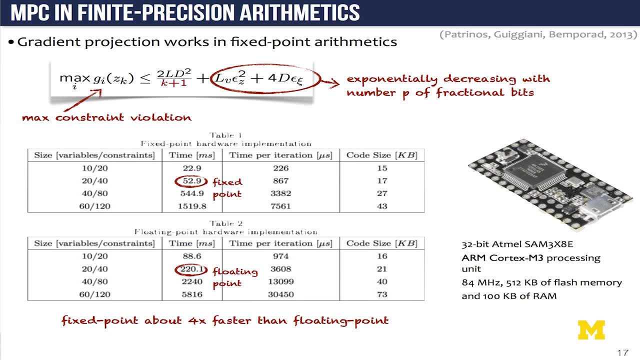 probably the most adequate ones, But these other are also good candidates for applications And these are other tests that Alberto Guigiani and did in the past. We looked at fixed point implementations of the non-accelerated version of the dual QP solver. 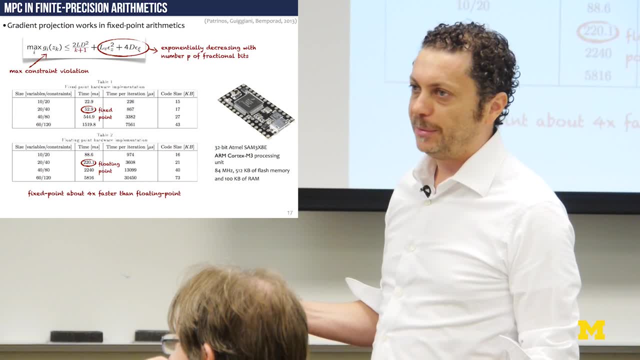 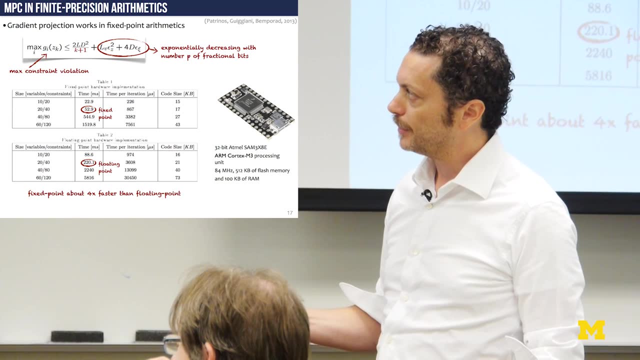 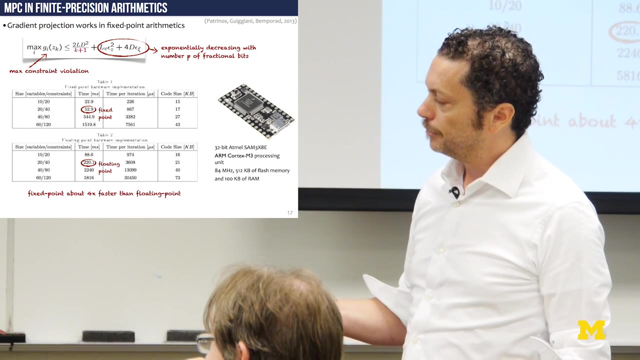 We actually could derive bounds on the number of bits you need to have in order to meet a certain precision in terms of satisfaction of the constraints, And we have a similar result for optimality. And this bound here goes down exponentially with the number of bits and tells you: 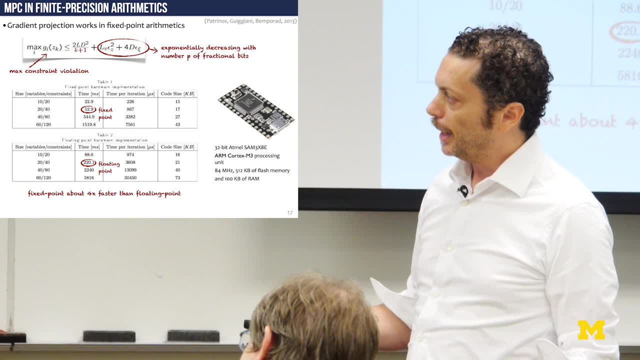 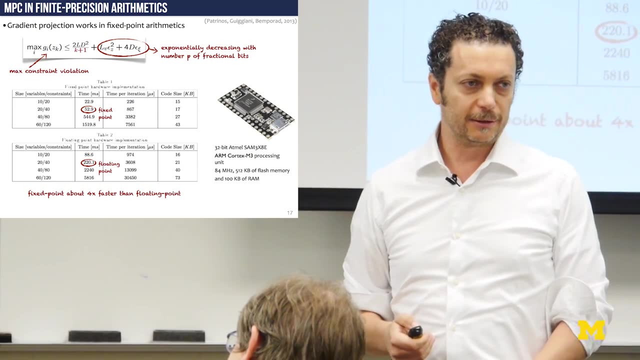 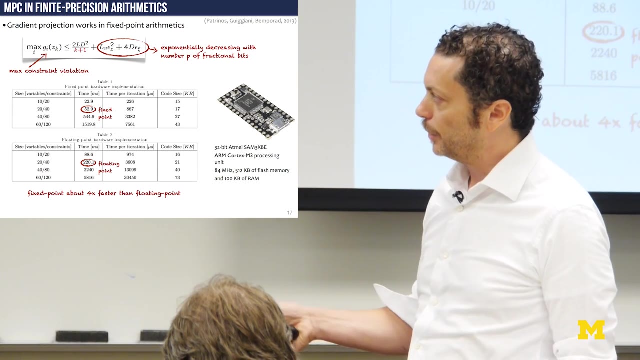 how many bits you need to have a certain precision. And if you implement the solver in fixed point arithmetics, this is roughly four times faster than the same algorithm implemented in floating point on the same platform, where the platform here is an arm, Cortex. 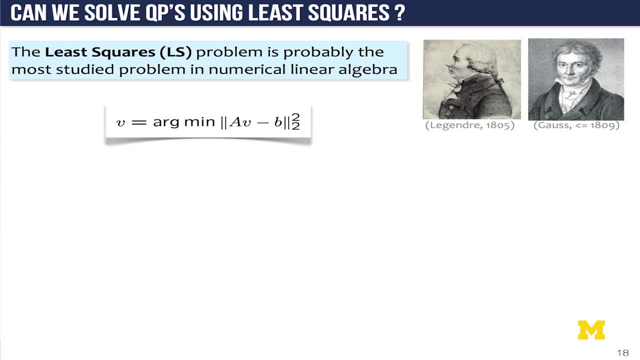 M3. And you can see that this is a very, very good result. And you can see that this is a very, very good result. All right, That brings us to another approach I've been working on recently, which is driven by the idea of using least squares to solve QP. 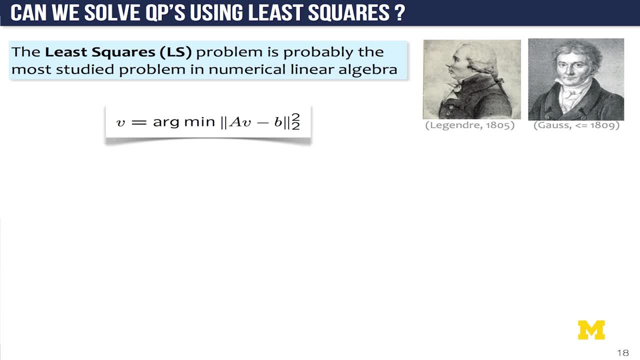 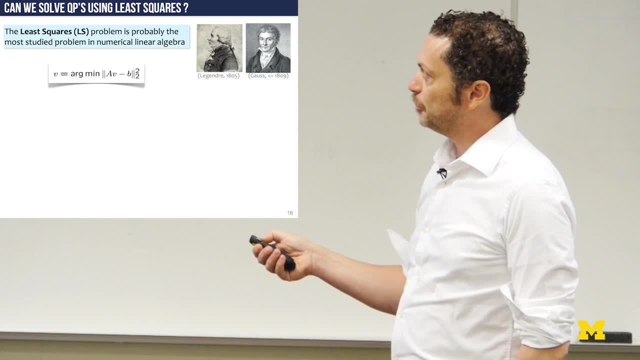 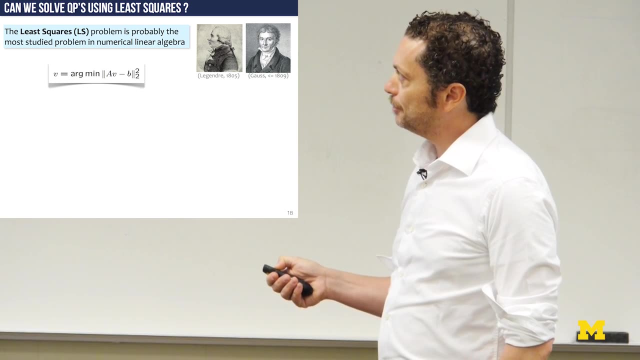 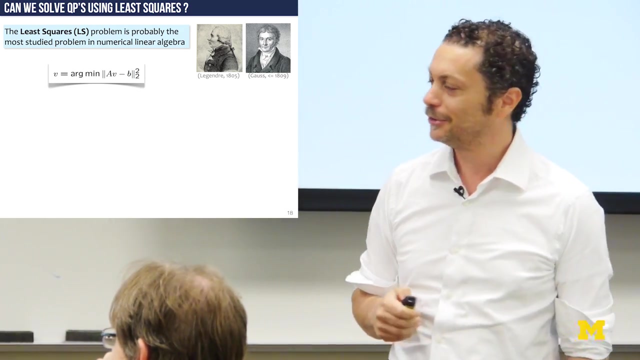 problems. So why least squares? Least squares are probably the most studied problem in numerical linear algebra. The idea dates back to the The beginning of the 1800 years. Not sure whether it was Legendre or Gauss. always this dispute is which one was the first. 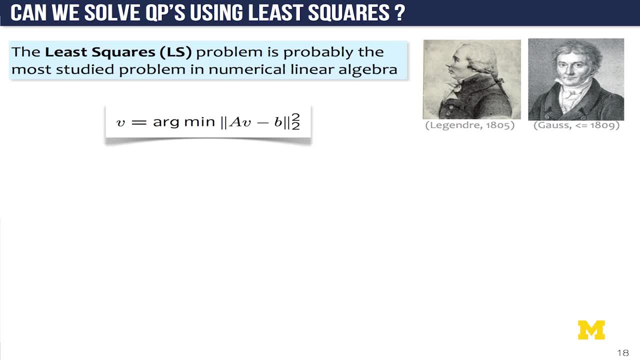 The problem is simply to minimize the norm of a, V minus B, where A and B are given. A is a given matrix, B is a given vector. The problem is so important that MATLAB has a comment that is just one character: the backslash. 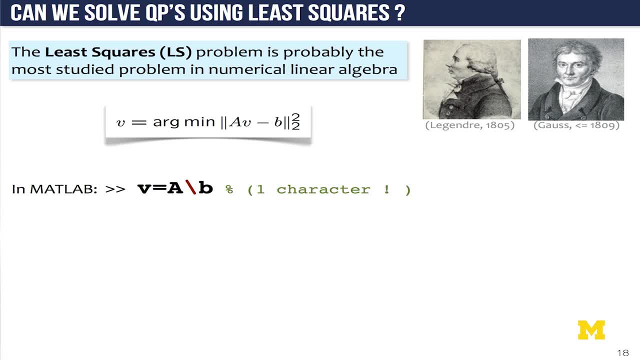 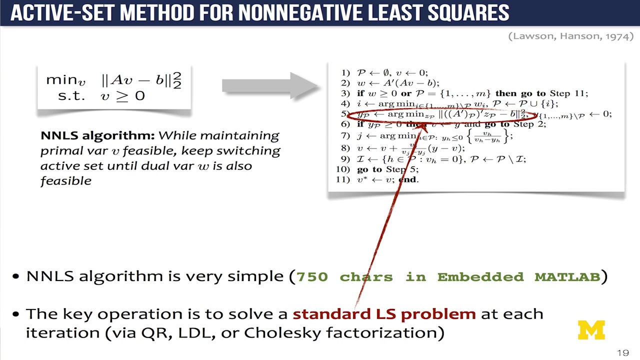 to solve the least squares problem And in particular I'm looking at non-negative least squares problems, where you want the variables to be non-negative. Why this class of problems? There is a nice book from the 70s. 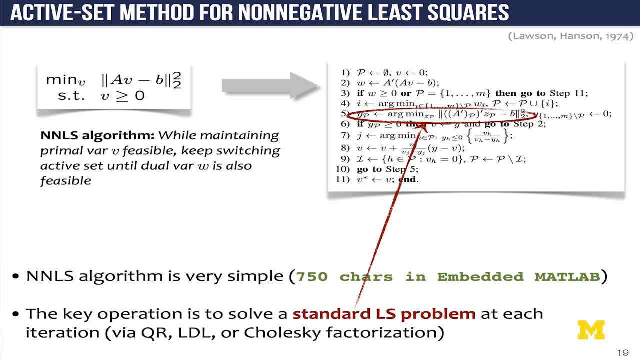 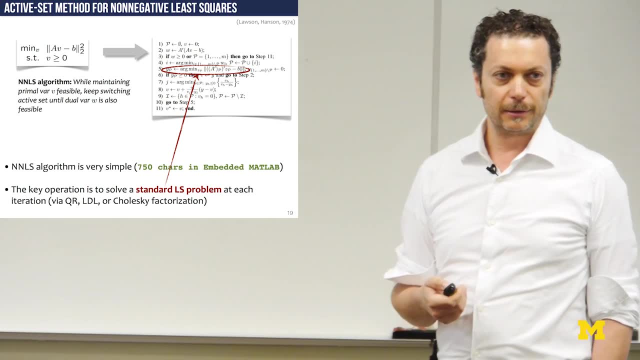 by Lawson and Hanson that analyze least squares, And there is a chapter also on non-negative least squares where they give an algorithm that is quite simple and quite efficient and is very well understood from the numerical viewpoint. So they also give a lot of insight. 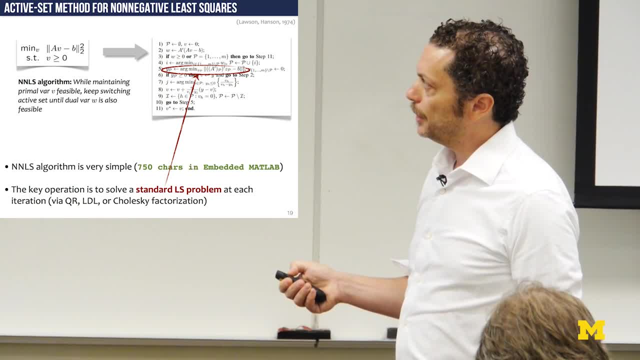 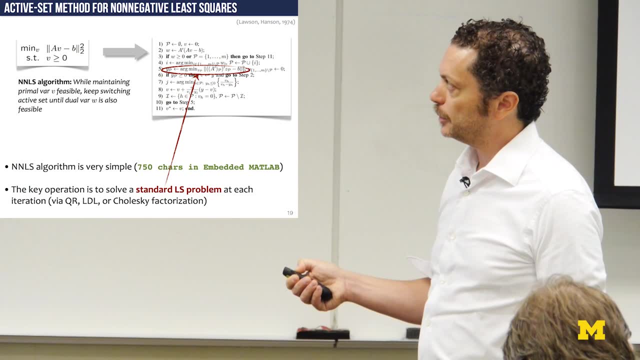 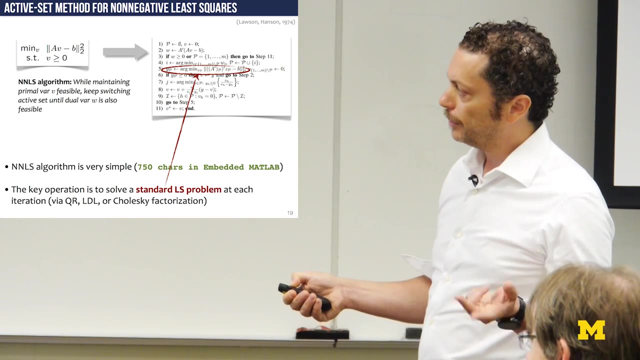 on how to implement this. The algorithm is an active set method that, at each iteration, solves a standard least squares problem And it keeps changing the active set, which is the non-zero V variables, until the dual vector of the problem becomes non-negative. 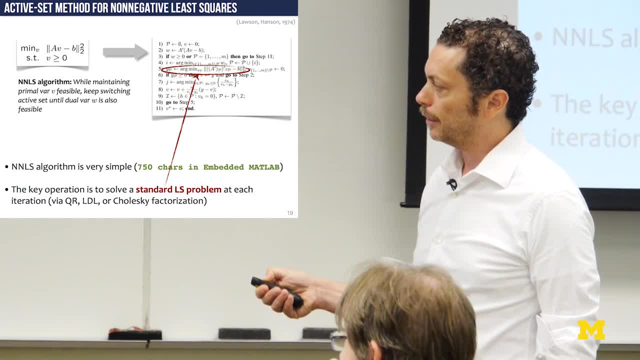 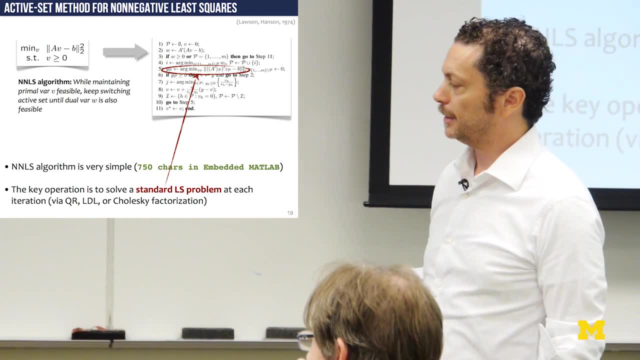 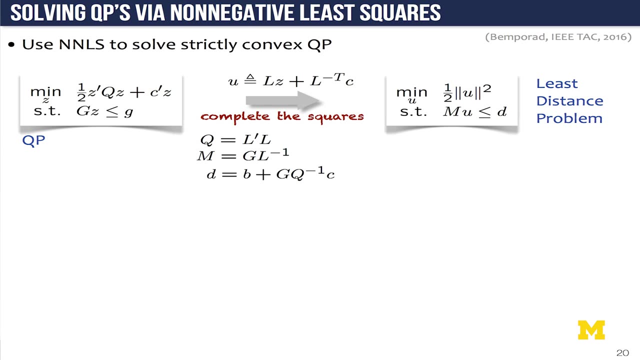 So the core of this algorithm is actually least squares solver that you can solve by QR factorization, LDL, Cholesky, recursive, non-recursive or whatever, So you can use this for your preferred method: How to solve QP's using non-negative least squares. 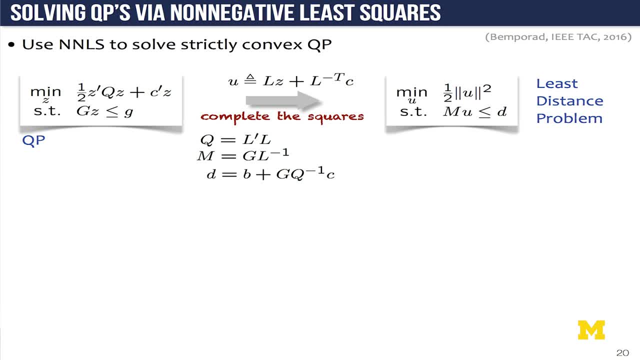 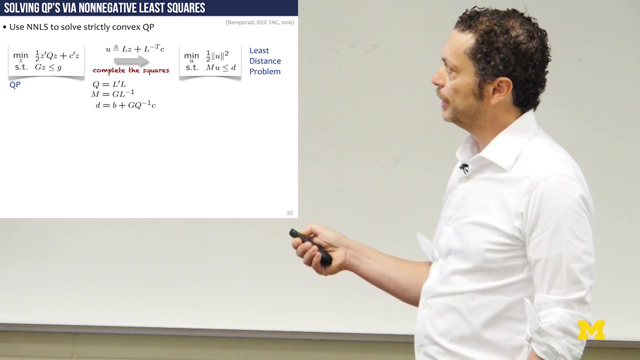 The idea is actually pretty simple. So you start with a QP formulation, You complete the squares by computing the Cholesky factor of the primal Hessian matrix Q and do a change of coordinates and reformulate the QP as a least distance problem. subject: 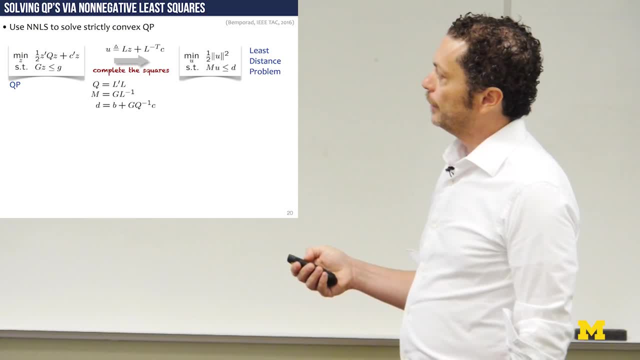 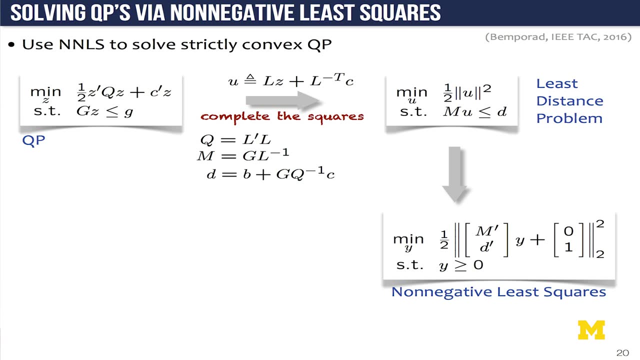 to polyhedral constraints And once you have done this simple transformation, you can solve this equivalent problem. So this: M is the constraint matrix, time, the inverse Cholesky factor and D is the linear cost of the dual problem. So you solve this non-negative least squares problem. 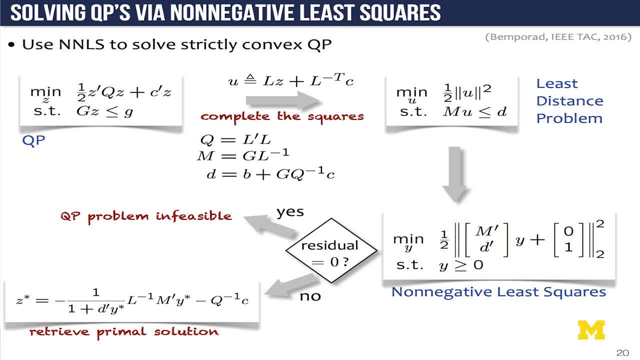 with respect to vector y, And then you look at the result. If the result is 0, then the QP problem is infeasible, Or otherwise. if the result is 0, then the QP problem is infeasible. 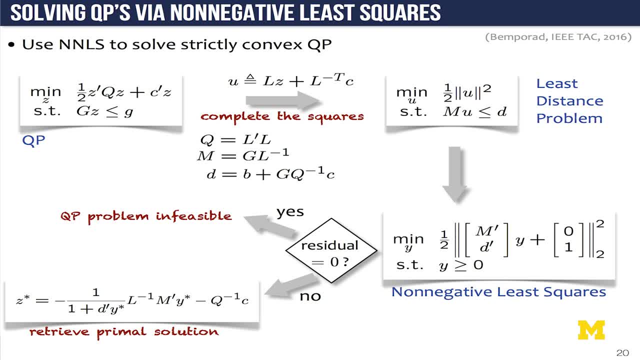 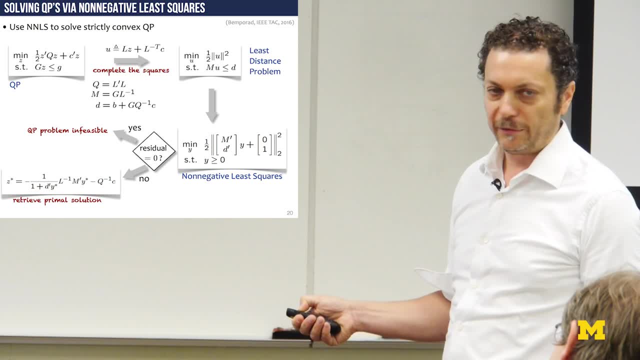 If the result is not 0, then you will retrieve the solution of the QP from this vector, y. Note that this is not the dual problem, So y is not the dual vector In this case, if the QP is infeasible. 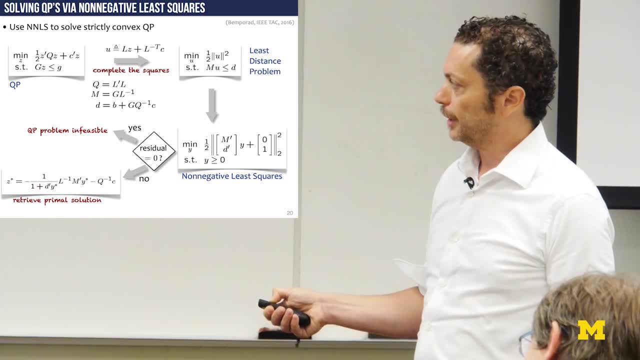 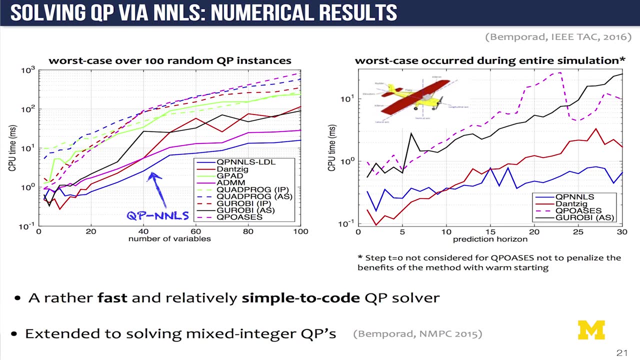 the dual vector will go to minus infinity. So it's similar but it's not exactly the dual problem. And here are some numerical results. So comparing this solver based on the result, the non-negative least squares and recursive LDL factorization to solve the least squares problem. 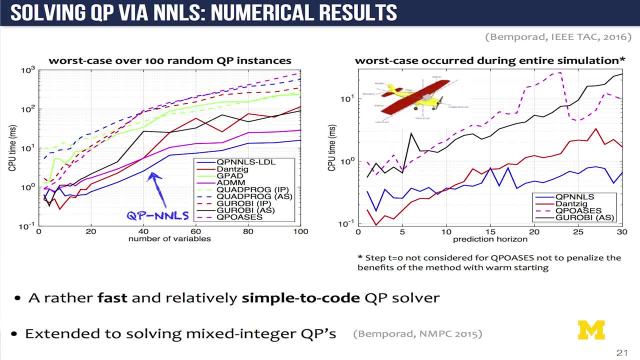 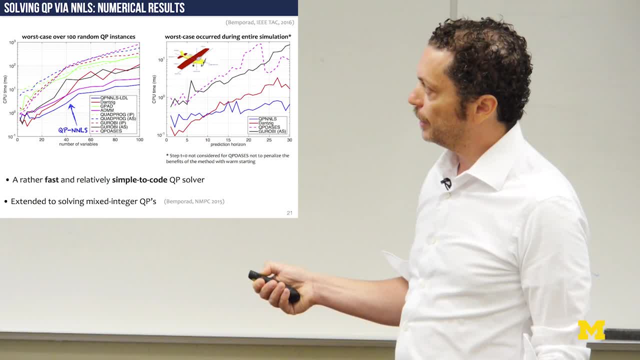 it's quite competitive with other active set methods. Also, we have ADMM. The gradient projection method is here, is the green one, QP Oasis is the one here, Gouraud being quadprog, Gouraud is a commercial one. 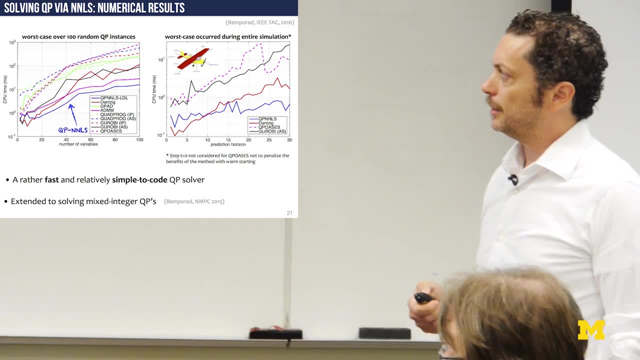 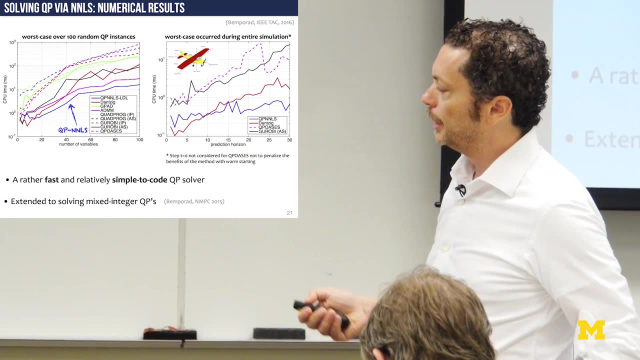 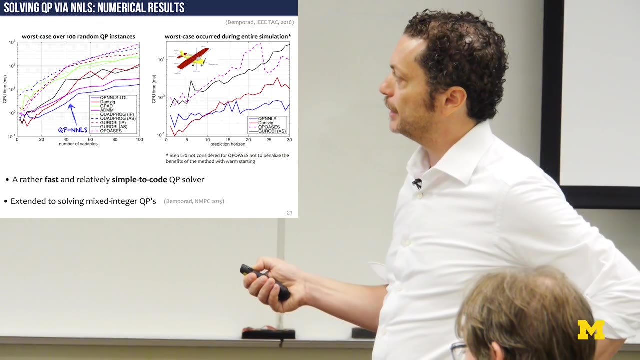 Quadprog is the one in MATLAB, So it's actually quite fast and also not too difficult to implement, Thank you. And here is an MPC application. This is to control the altitude of an aircraft. Two inputs, two outputs. The system is open loop, unstable. 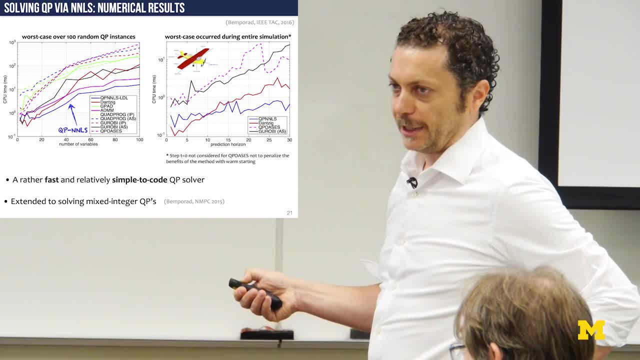 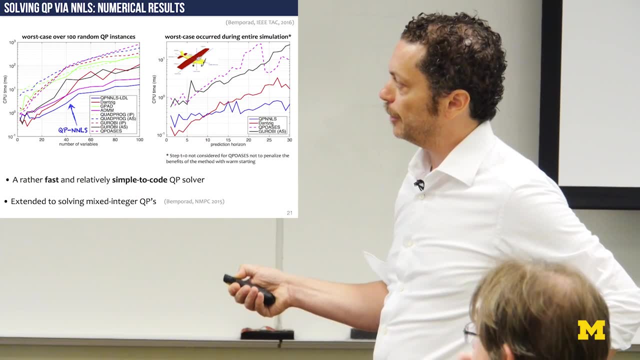 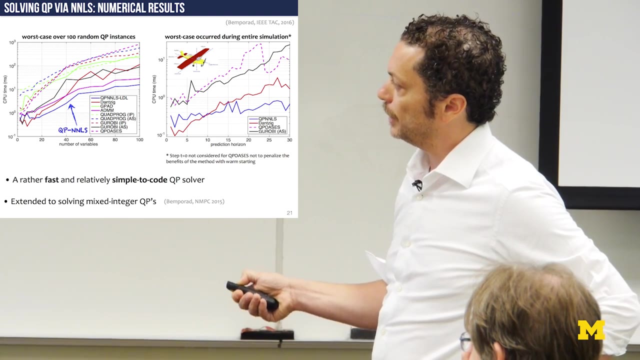 And here is the complexity: CPU time in the worst case. Except the first step, which I don't count because QP Oasis is quite bad on the first step, It takes advantage of warm start during the following steps. This is the worst case. execution time. 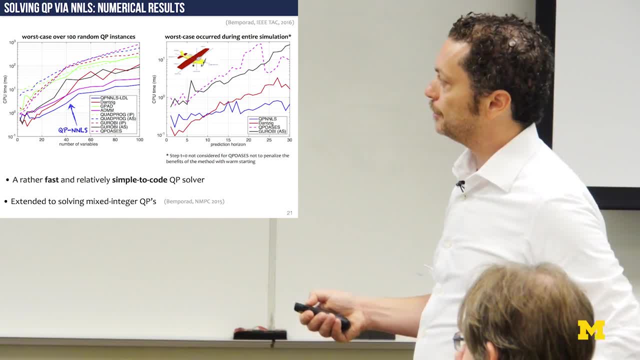 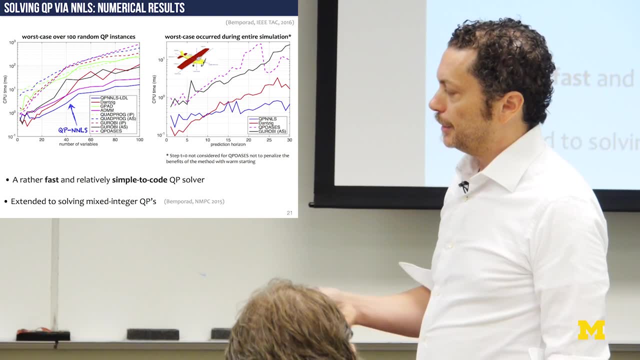 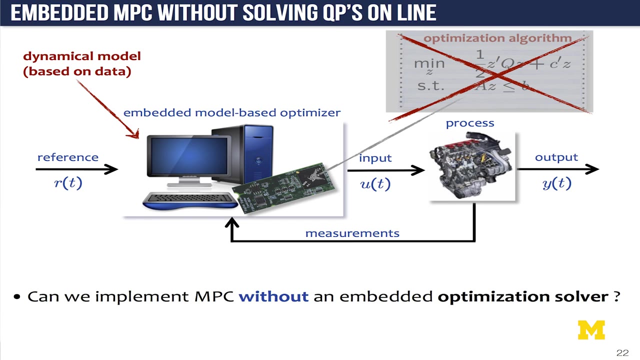 as a function of the prediction horizon, That is, as a function of the problem complexity. This can also be extended to mixed integer QPs. I presented this last year in the nonlinear MPC control conference. So now next question. We have QPs, good QPs. 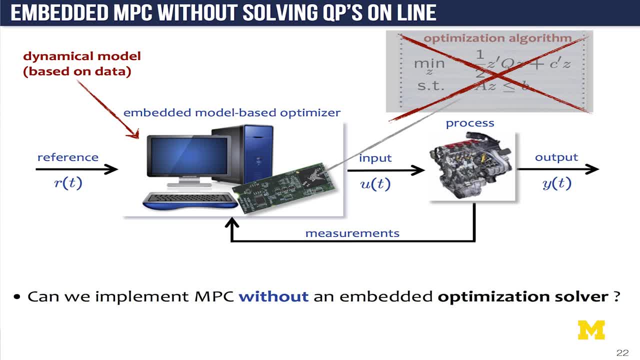 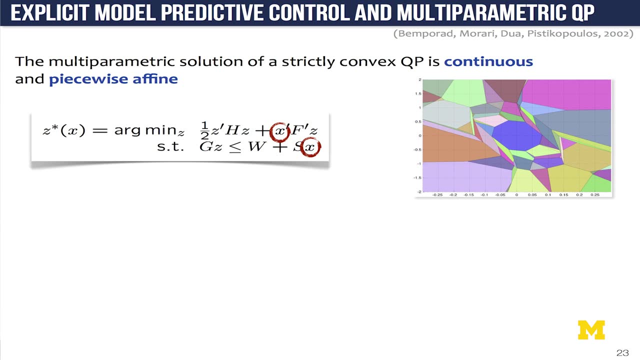 But can we solve MPC problems without QPs? Let's say you don't want to implement a solver for different reasons. OK, So you can solve these problems online. Can you still use MPC? Well, the answer is yes, And this was studied now, about 15 years ago. 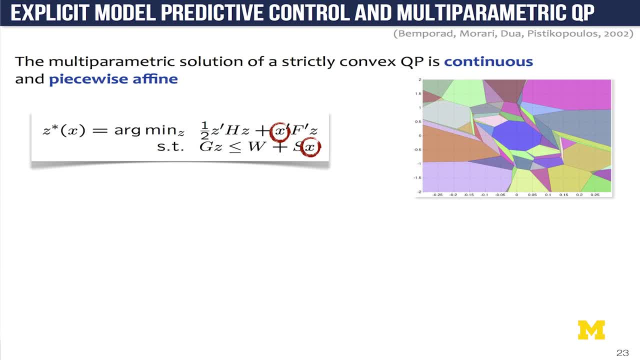 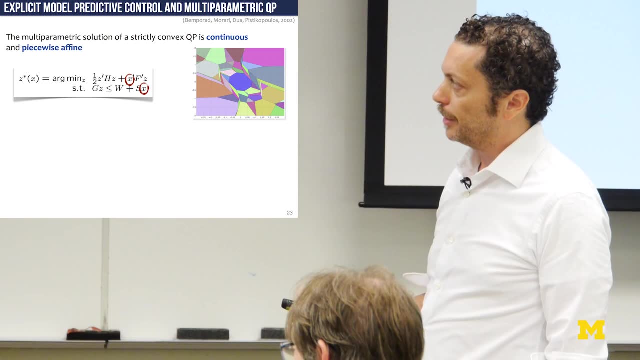 In a paper we wrote where we show that if you look at the QP as a parametric quadratic programming problem where the parameter vector is the state, the state and reference vector, you can solve this problem offline and get the solution as a function of x. 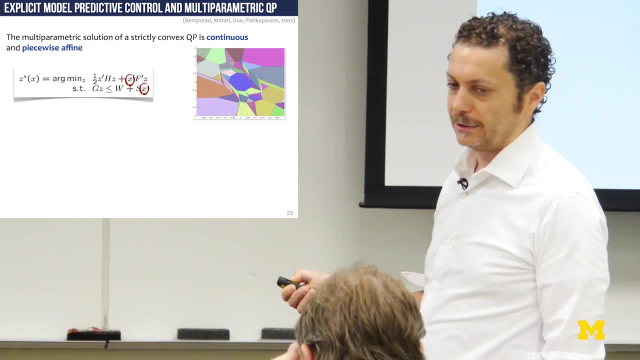 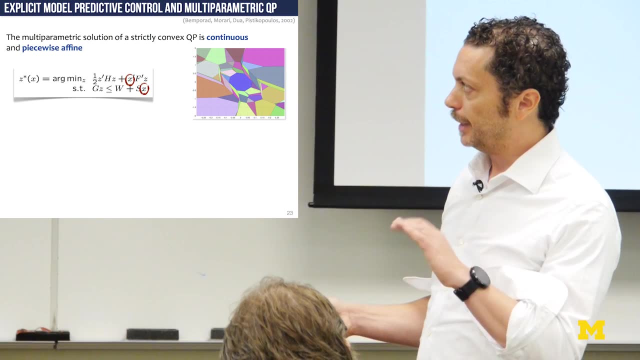 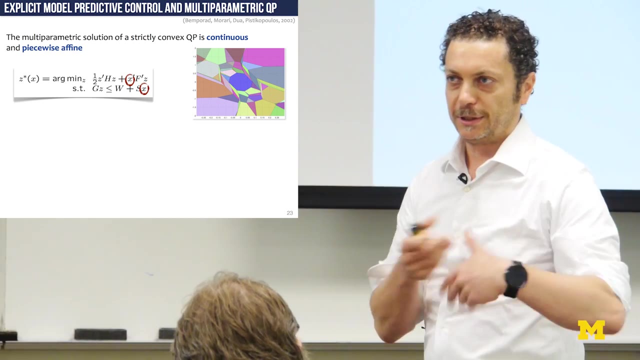 And this solution? it's piecewise, affine and continuous, So actually you don't have to grid the state space to find the solution at different points. The algorithm gives you the solution in the exact solution if you were working in infinite precision arithmetics. 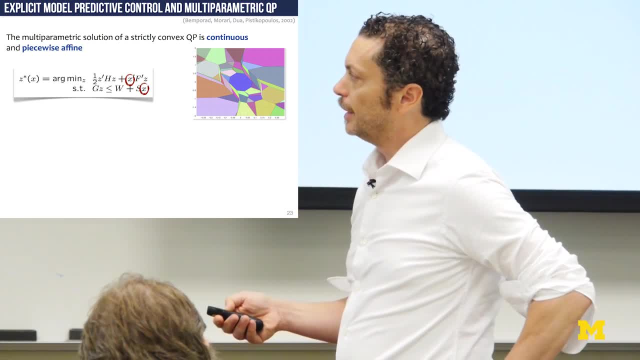 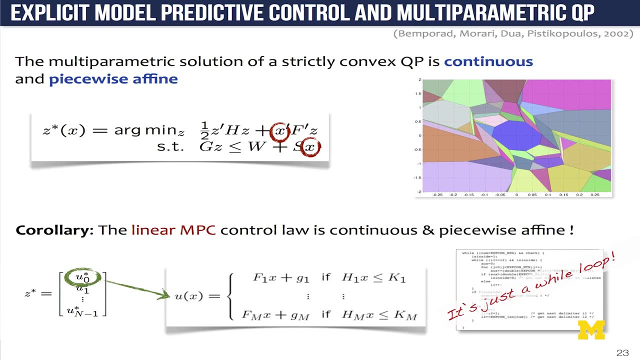 It gives you the explicit form of the solution, And this is very nice. You know that the solution is continuous. So the controller that you are implementing, which is the first sample of the solution, it is a continuous controller, So it's a continuous function of the state vector, which 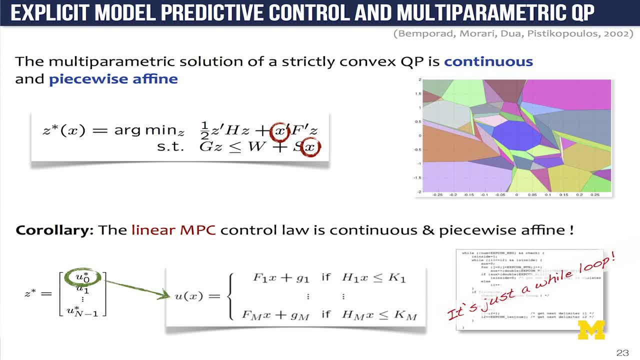 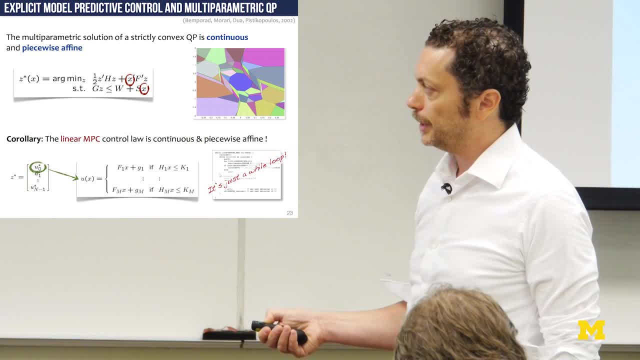 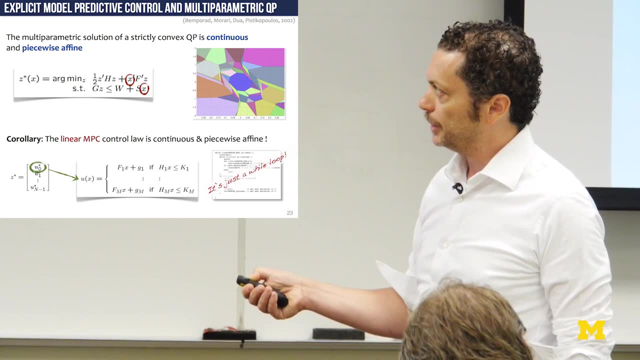 is good for robustness reasons. But the main thing is that this controller is piecewise affine controller. So the solution is a lookup table of linear controllers where, online, you have to see where your state vector is In which partition And then pick up the right gain. 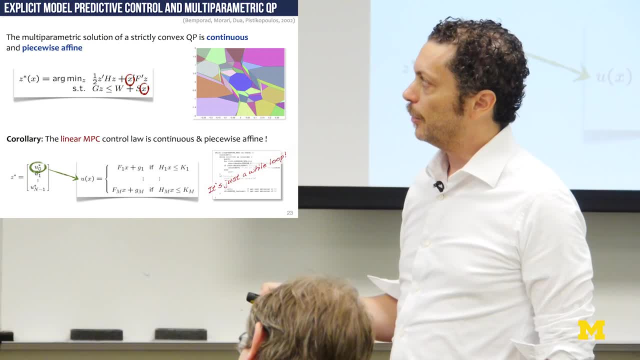 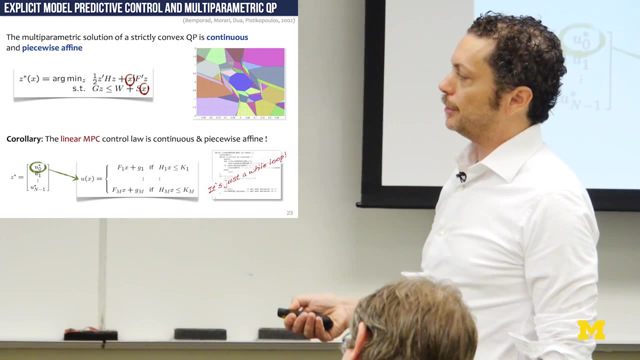 So it's nothing else as a gain schedule, where the scheduling is driven by the partition that you get automatically from the solver. So, again, the implementation of this then becomes quite trivial. It's a wide loop in the simplest form, A wide loop over all the region, until you. 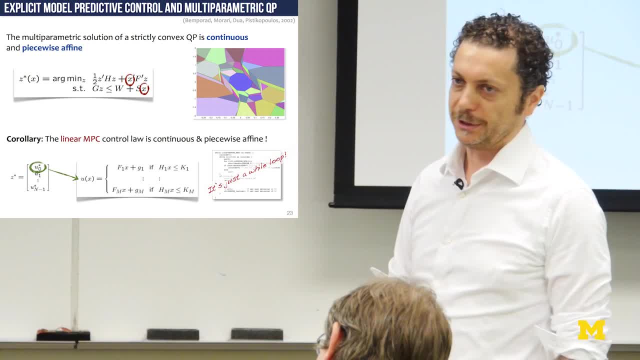 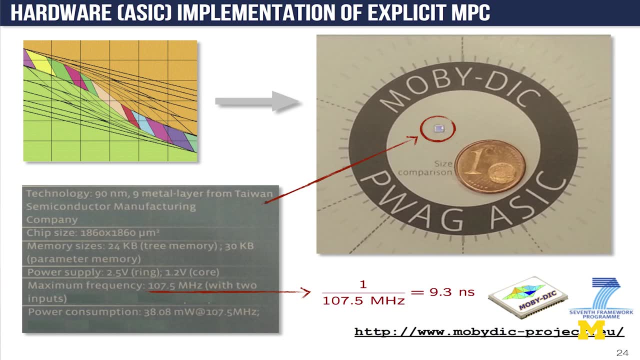 find the one where you are And then you compute a linear feedback law. This is also interesting for implementation. These are some experiments we did within the European project, together with a group in electronics at the University of Sevilla in Spain and a group of electronics in Genova. 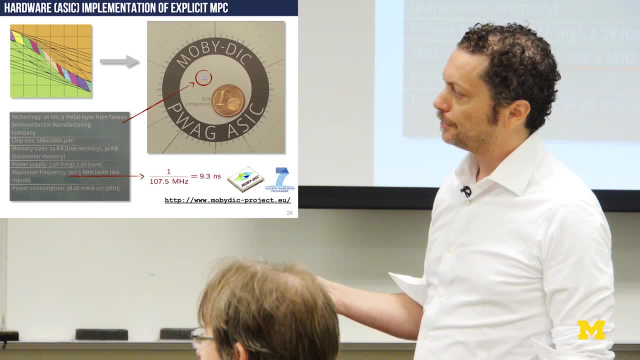 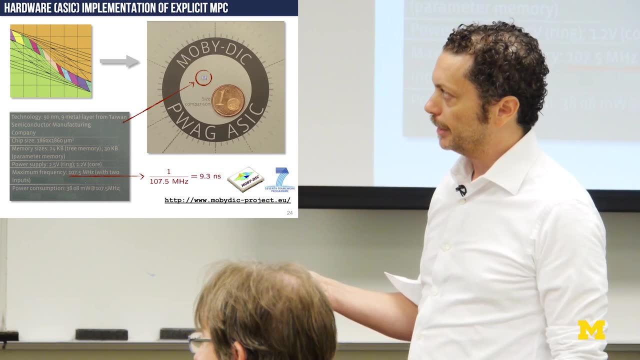 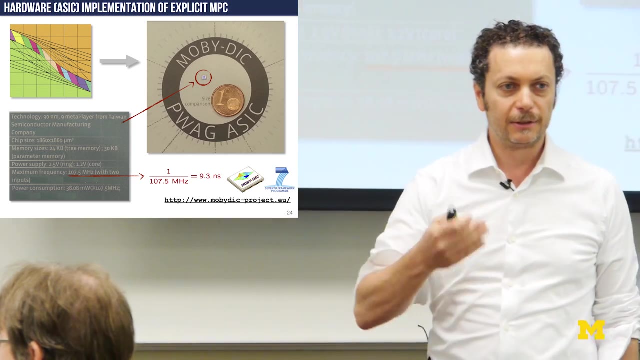 Taking an explicit control, MPC control law and then embed these first in an FPGA and then on ASIC and the bar in the circuit and test the speed you can have on this circuit And it turns out that in About 10 nanoseconds you can compute an MPC law. 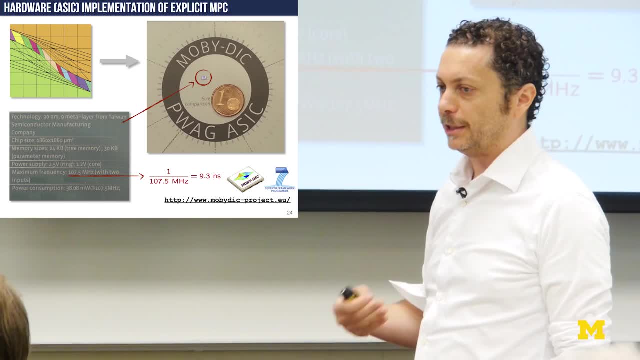 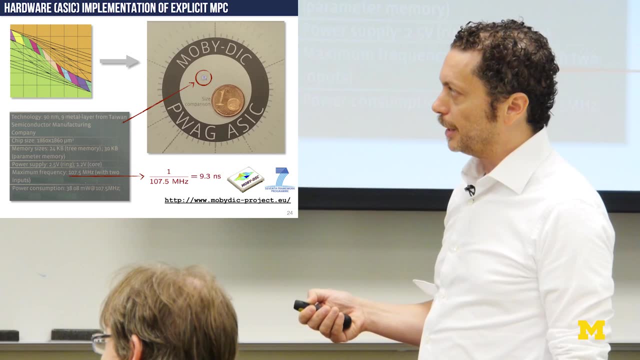 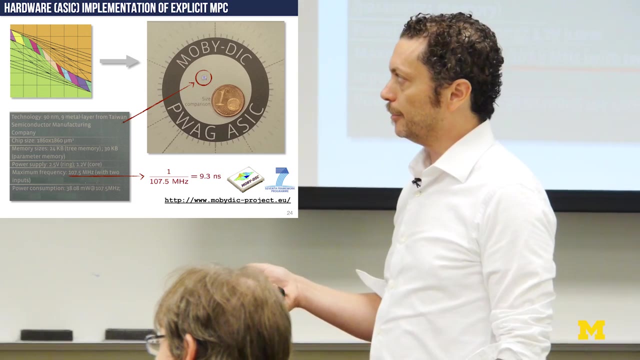 So that gives you an idea of how fast you could run an MPC controller, For example in a power electronics application where the sampling time is very small, that you could still run MPC control laws for such fast system if the control law is implemented in explicit form on a chip. 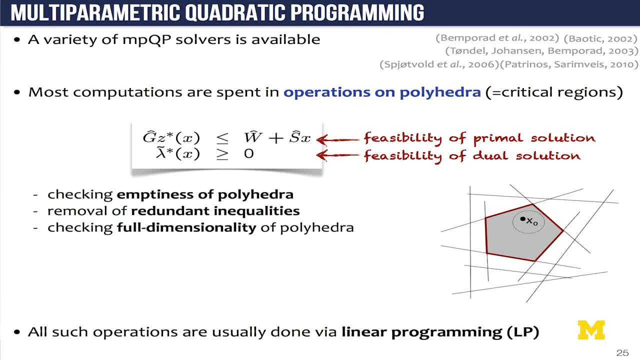 Now To solve the multi-parametric QP problem. there have been different approaches developed mainly between the year 2000 and 2010 by different groups. They are very much related to each other, Namely, they all look at the conditions. 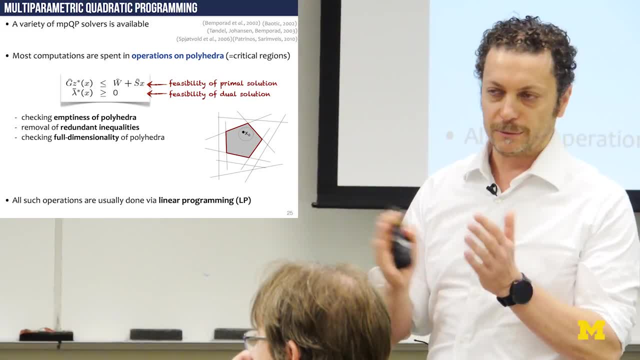 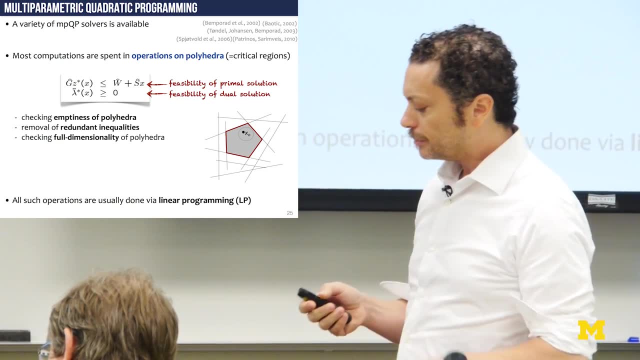 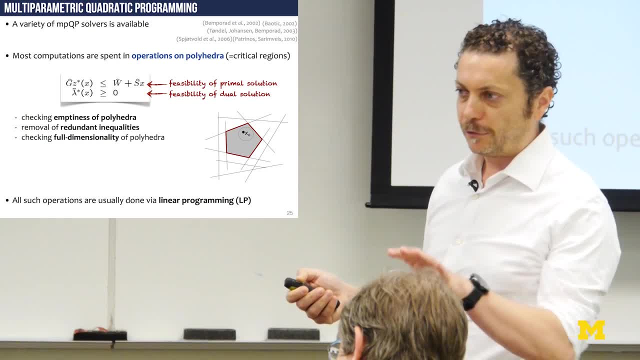 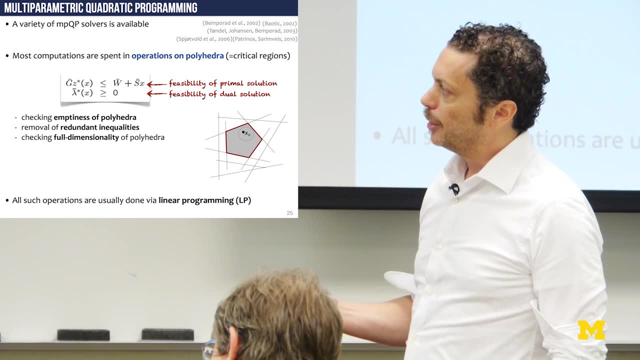 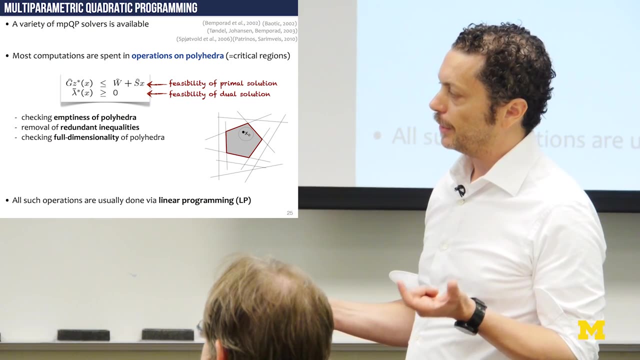 Most of the time for these algorithms, these are offline algorithms to solve the problem in explicit form. most of the time is spent on checking feasibility of polyhedra. Namely, you find from the KKT condition what the optimizer for the primal problem and dual problem. 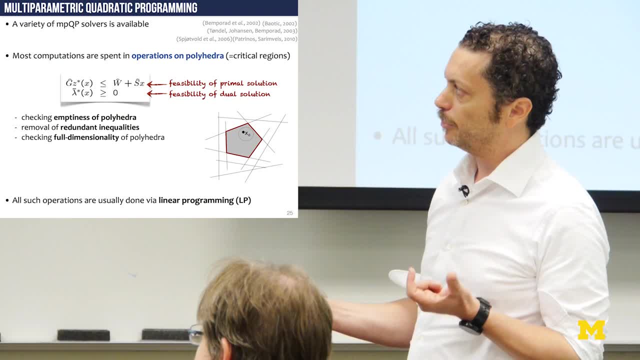 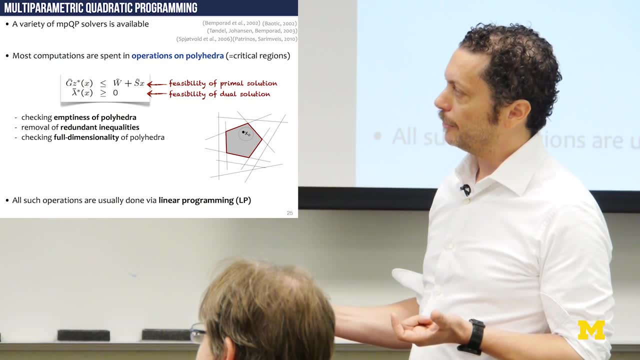 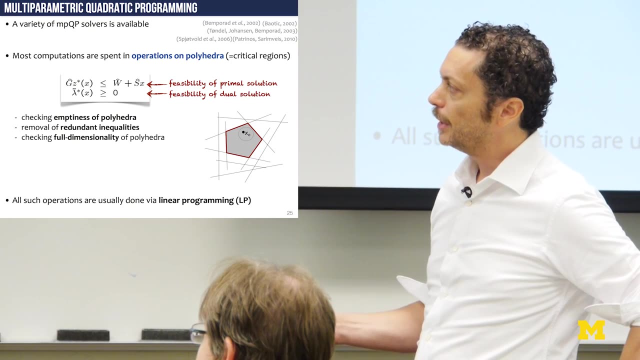 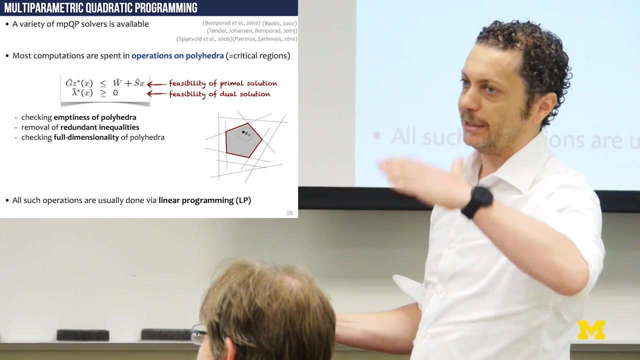 is as a function of x, And then you impose that both are feasible. So this creates linear inequalities with respect to x, and so you have to get rid of redundant hyperplanes in this linear set of inequalities, and this is traditionally done through linear programming, by taking each hyperplane and maximizing. 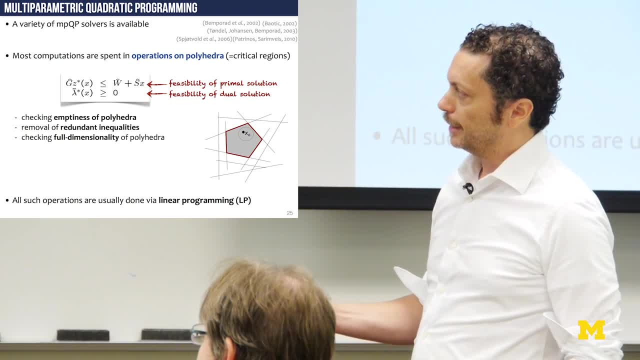 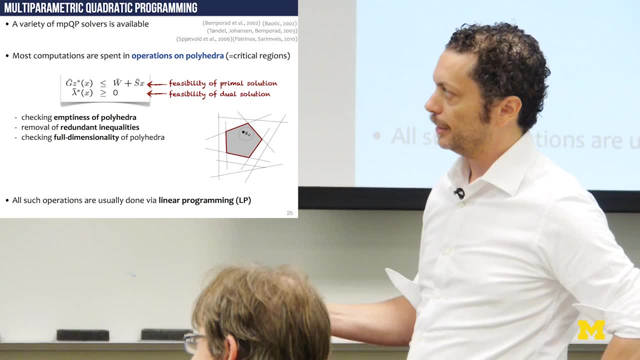 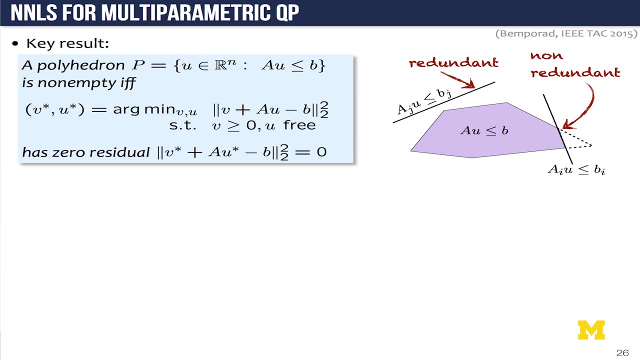 the hyperplane and see if the optimum is subject to the remaining constraint and see if, at optimality, you are on the hyperplane or you are on a on the lower value. when I was asked, Matt works to implement explicit MPC in the toolbox, we couldn't have an LP solver to solve the multi parametric QP. 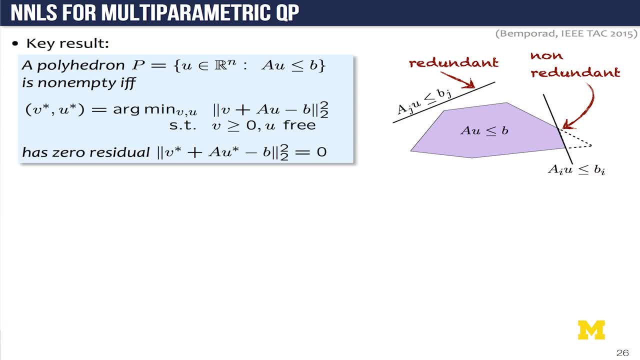 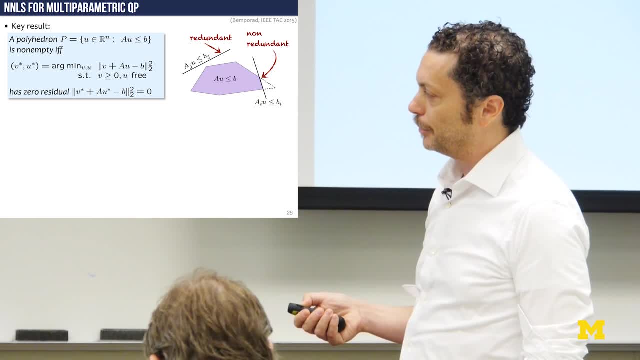 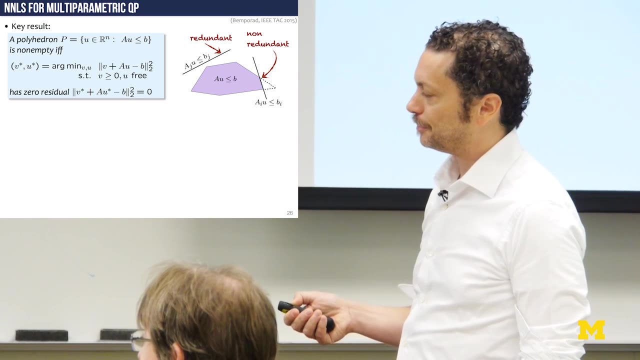 so we had to come up to a different solution, and that triggered some action, actually some interesting research for how to perform several polyhedron computations without LPs, but using again non-negative least squares, And the result is actually quite simple If you look at the polyhedron, if you 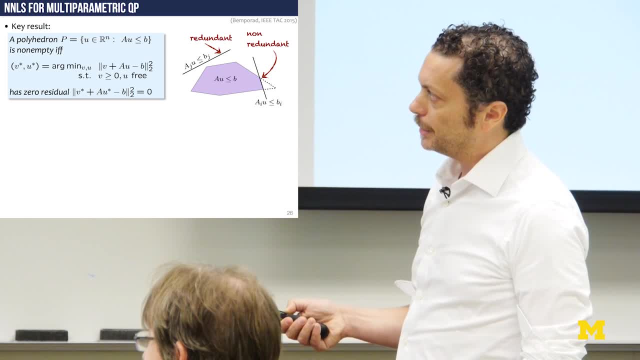 want to test whether this is feasible or not. you can solve this non-negative least squares problem, where some of the variables are non-negative, some are free, and look at the residual. If the residual is 0, then you have found the feasible vector. 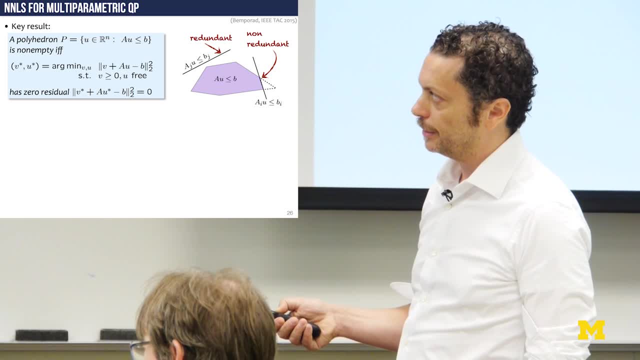 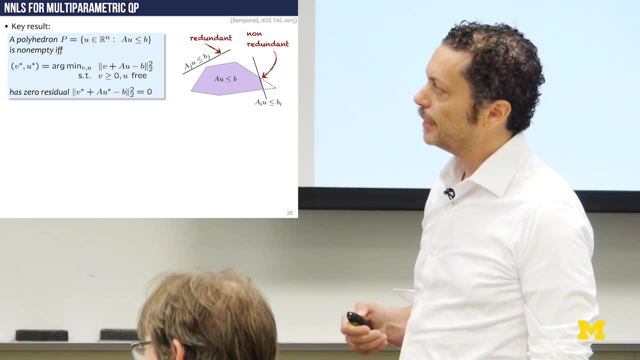 u, because au minus b will be negative or equal to 0. So it will be a feasible point. Or if the residual is non-zero, so it's greater than 0, then you can prove also the other way around that the polyhedron is infeasible. 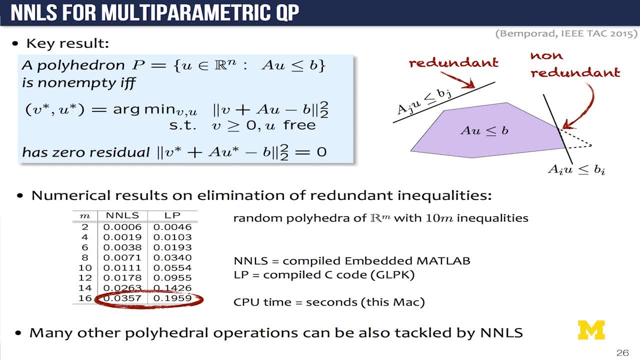 And then you can use this to test redundancy of hyperplanes using different approaches. One which is quite efficient is to take lower dimensional polyhedra, where you consider each possible facet. say, this hyperplane, this would be not redundant, This hyperplane, this would be an empty facet. 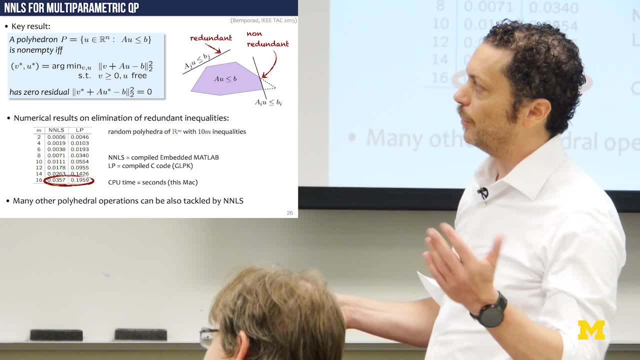 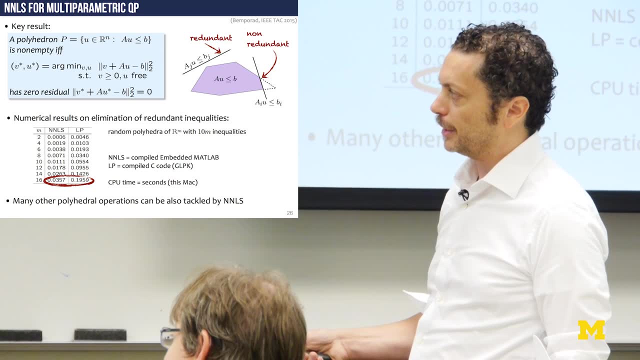 in the polyhedron And then use this approach to discover whether the facet is empty or not, And actually it turns out that this is quite faster- about one order of magnitude faster than using LP, And actually these results are a bit 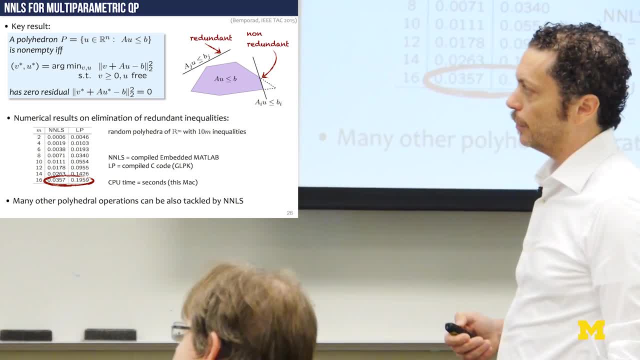 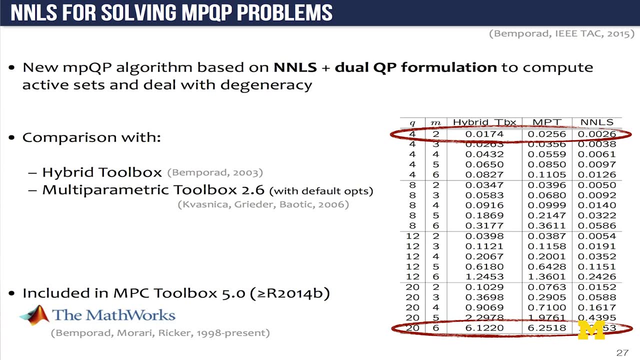 contained through the public domain GLPK code for solving LPs, which is written in C, And it's actually quite efficient. And so, in the end, by also formulating the parametric QP problem in its dual form and then solving the dual form, 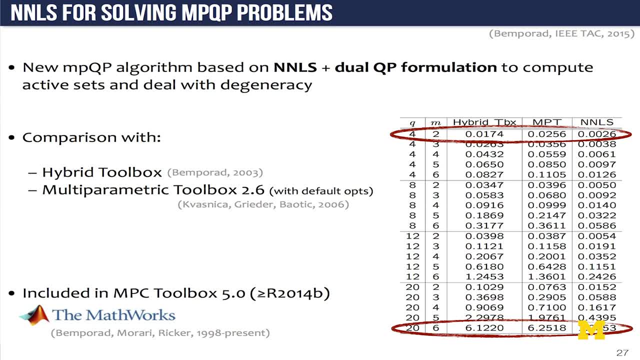 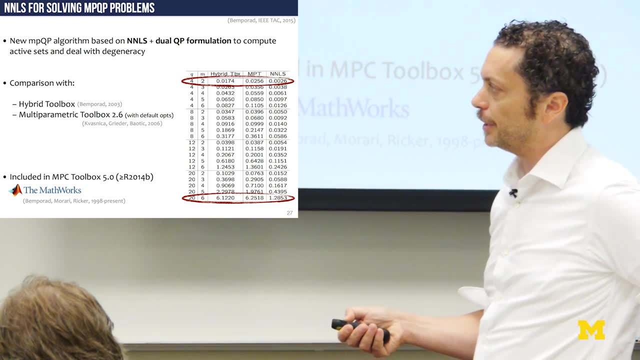 directly in a parametric way, then this is the solver that is described in this paper. This is implemented now in the MPC toolbox And it's actually faster Than other ones- the ones they had in the hybrid toolbox and the one developed in the group in Zurich. 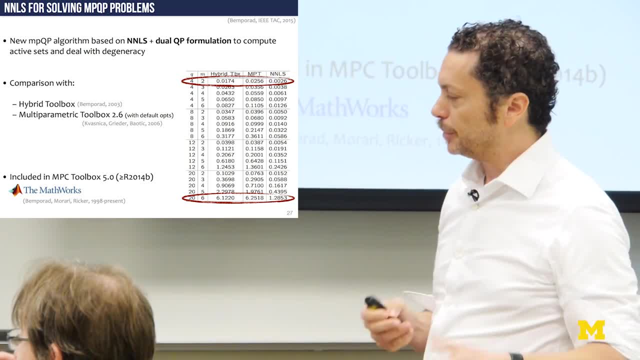 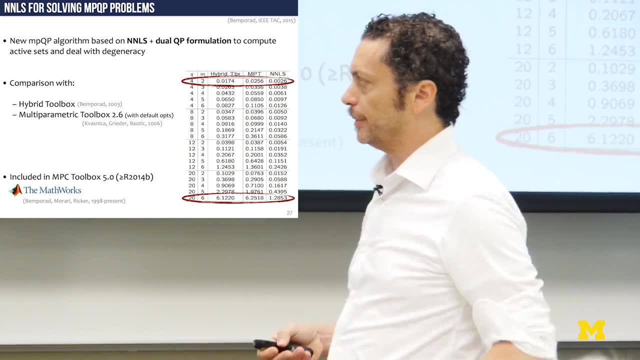 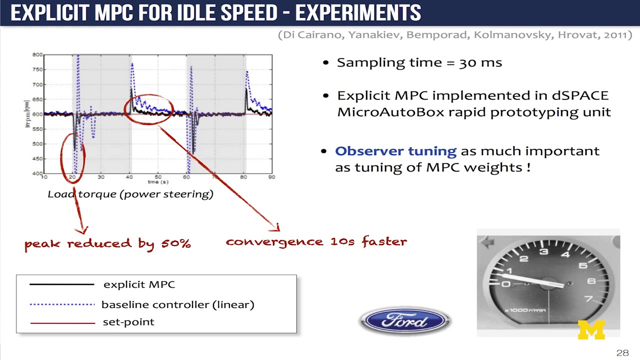 the multi-parametric toolbox. Of course this depends also on the problem and the type of options you choose, But I would say roughly all the solvers have the same order of magnitude for solving a given parametric problem, And this is an application that we worked out. 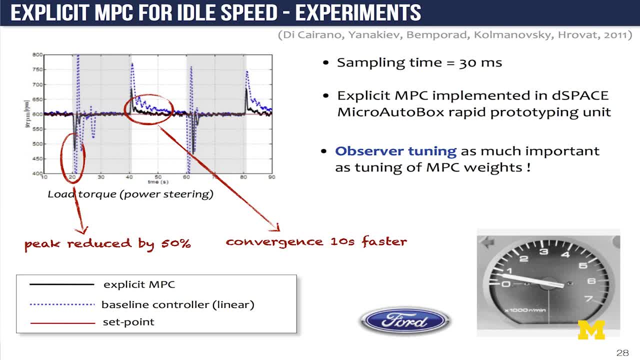 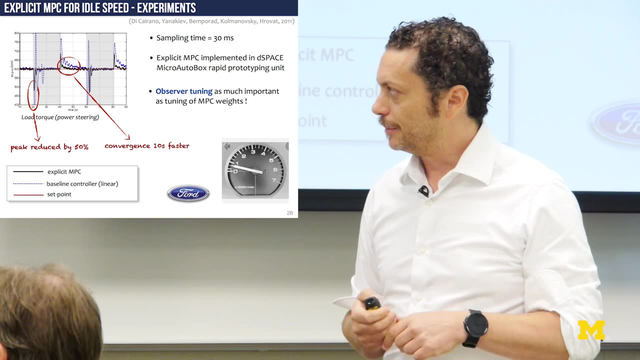 with Ilya Navarro, Stefano Di Cagliano and Diana Yanakev some years ago using explicit MPC to control the RPM on the engine when it's in idle- So probably the most classical control problem of idle speed control, And that we worked on using MPC and then explicit MPC. 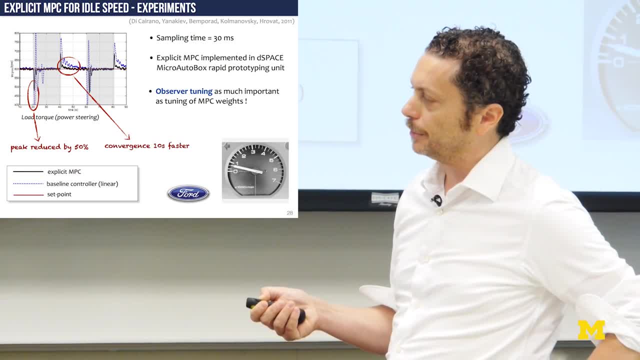 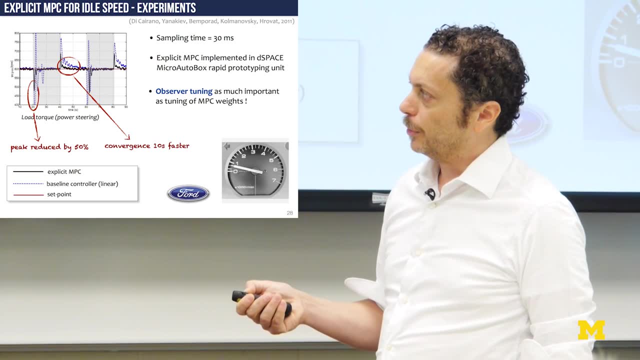 Feature of this product is a simple problem, but it has constraints on the torque you can generate and also on the RPM, The minimum RPM that you can tolerate during idle. So you want to prevent these negative peaks in RPM And the system also has delays. 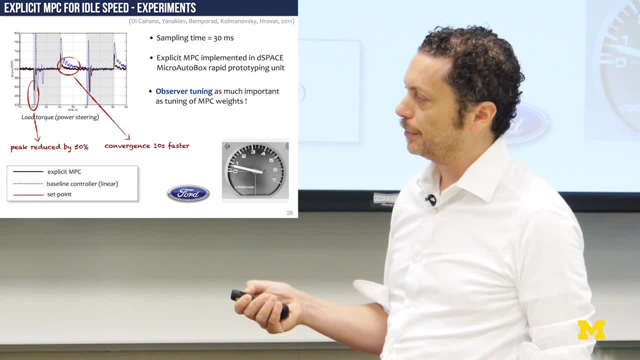 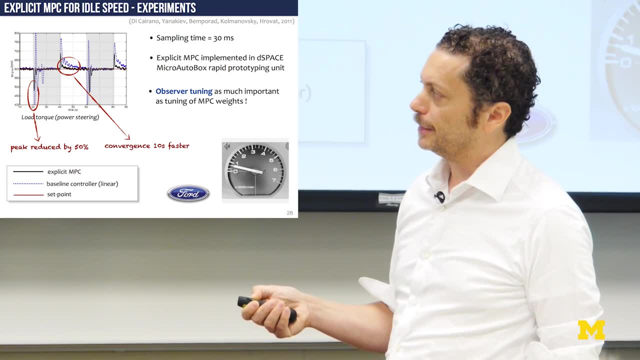 So we derived simple linear models with delay as prediction models And then designing MPC controller in explicit form and run some tests. And this is a comparison of performance. The blue one was a baseline controller, Linear controller available at Ford at that time, And the black one is the MPC controller. 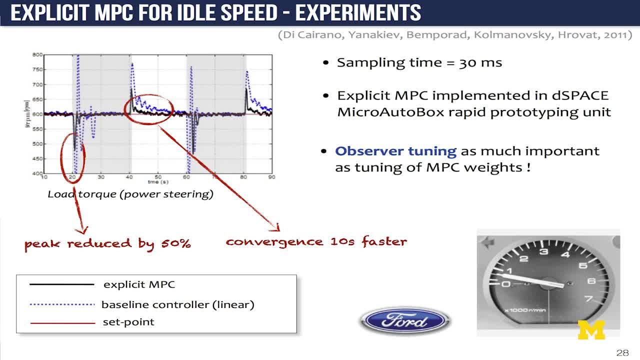 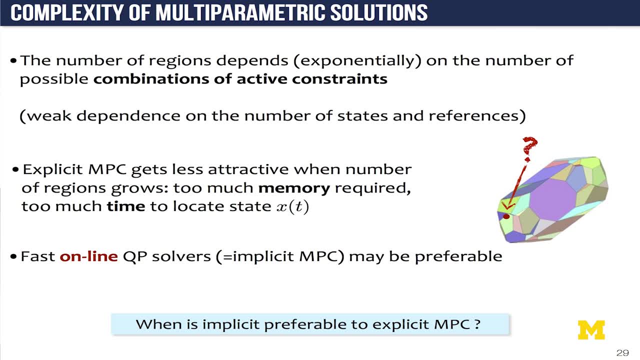 So you have convergence, which is faster, and also the peaks are reduced. So it's a good controller. So about the complexity of explicit MPC, Explicit MPC unfortunately is not the solution to all MPC problems. And why is this? Because the number of regions can grow quite a lot. 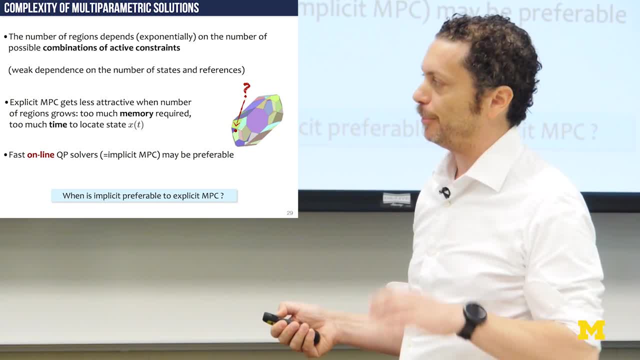 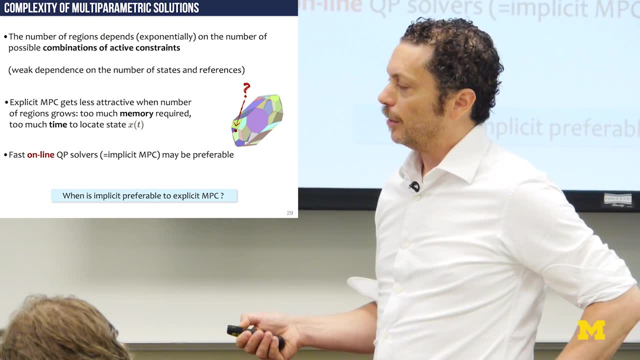 as the number of constraints that you have in the problem. It doesn't depend that much on the number of states and references, But it mainly depends- and actually in the worst case depends exponentially- on the number of constraints that you have in the problem. 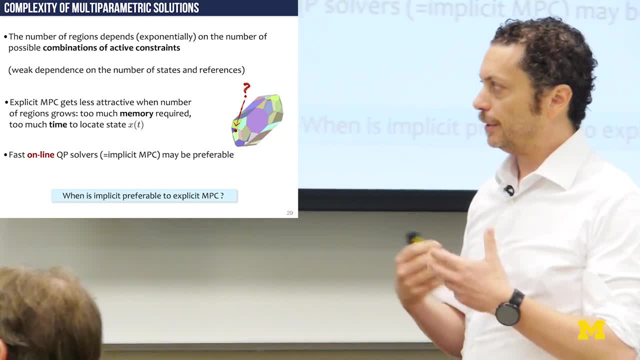 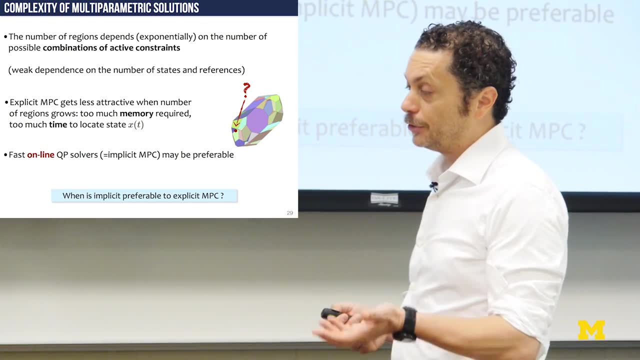 So this partition may become very large, with thousands of regions, And then at that point it becomes questionable whether this is more efficient than actually solving a QP online, which- let me call this an implicit MPC, where the control law is implicitly functional. 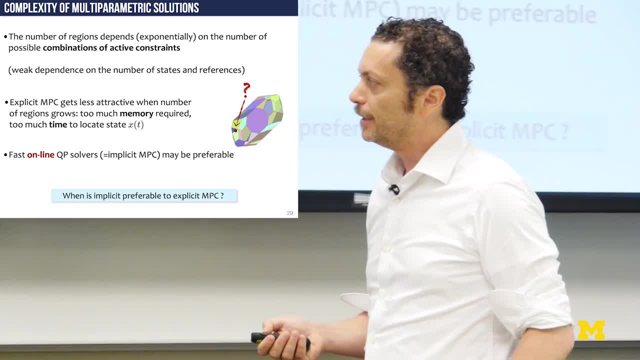 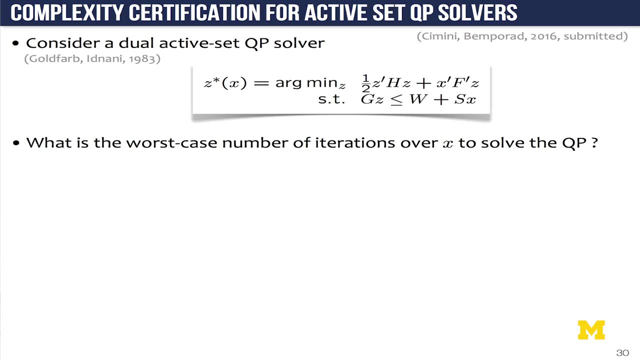 It's an implicit function defined by the solver. So when is implicit preferable to explicit? Not clear, It wasn't clear. We did a work recently with Jonathan Cimini on trying to understand and answer this question, but actually trying to understand what is the worst case: execution time for a dual active. 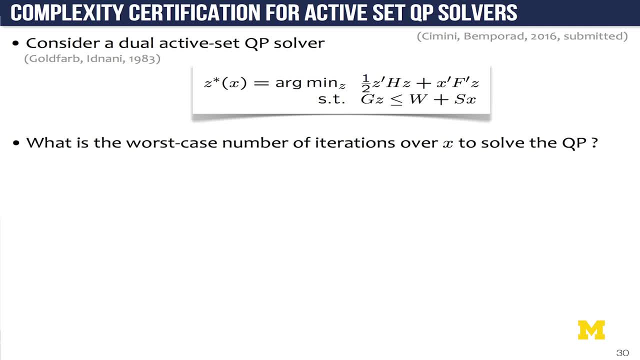 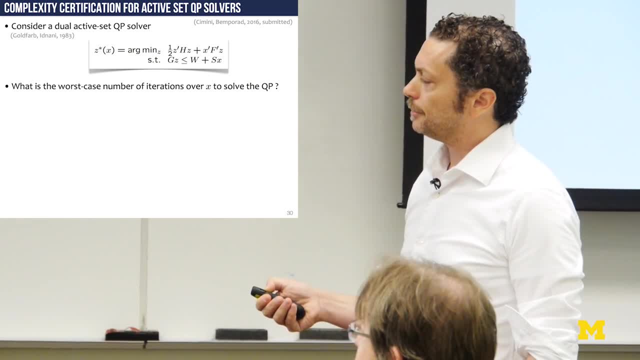 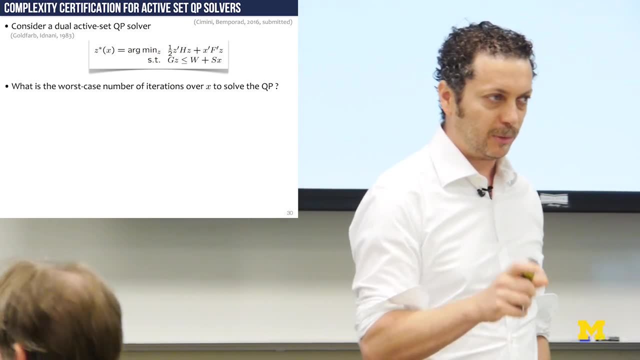 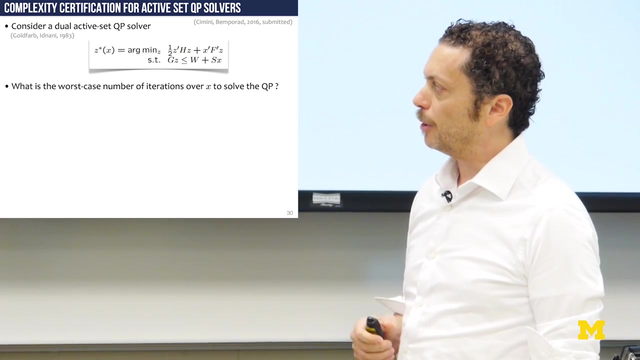 set solver. In particular, we considered the active set solver of Goldfarb and And we wanted to compute the worst case number of iterations this solver can take so that when we implement this solver we know exactly what is the worst case number of flops. 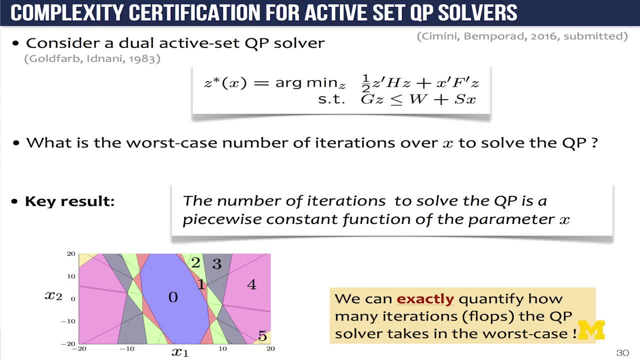 and what is the worst case, memory allocation. And we came up with a result Which is quite interesting. It turns out that the number of iterations to solve the QP is a piecewise constant function of the parameter vector x, Meaning that offline you can start an algorithm. 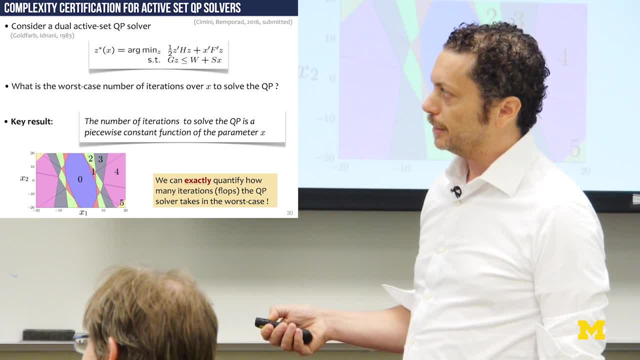 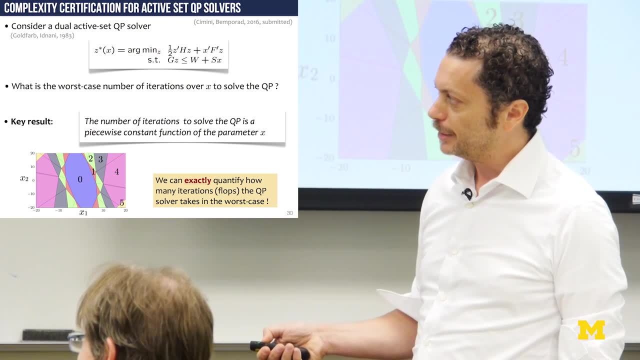 which is similar to the multi-parametric solver to subdivide the parameter space And at the end you get a partition which actually you don't care of. What you care is the largest number, this case 5.. So this proves it's a certification. 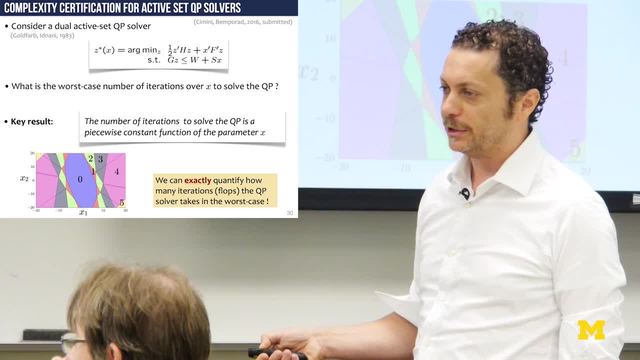 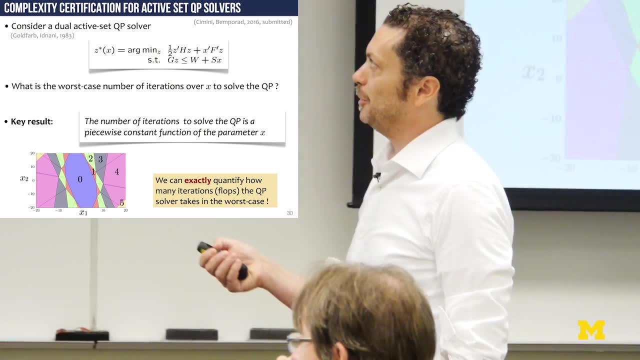 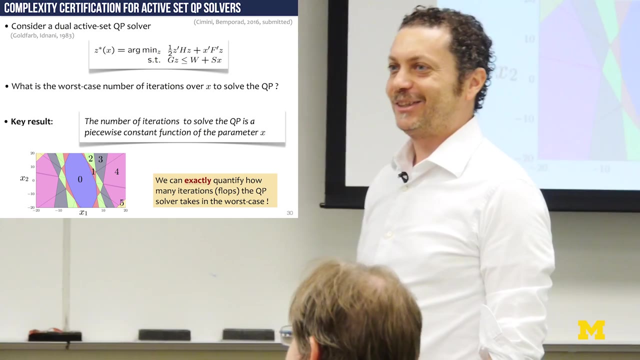 that the QP solver to solve this problem will never take more than five iterations to get the exact solution. So this was a submitted paper. We don't know yet the outcomes, But we are nonetheless. even the outcome would be negative. We are very proud of this result because it's very useful. 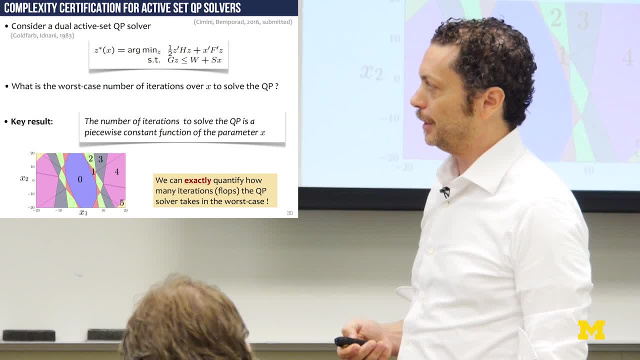 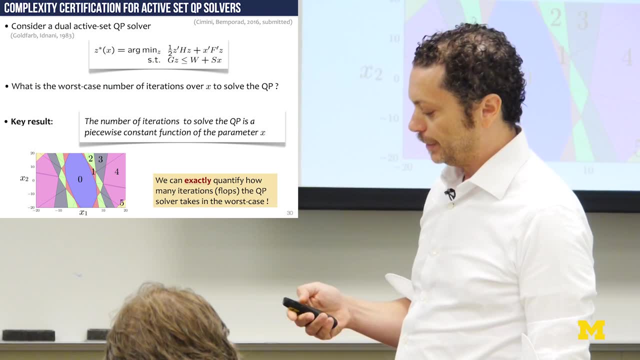 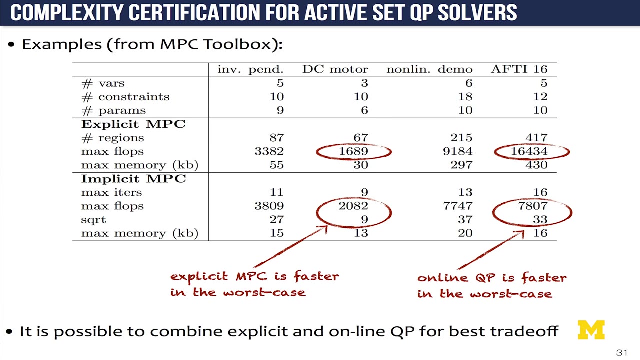 It's very nice, The theory behind it is also very useful in practice, And so, when you have this result available, you can compare explicit MPC versus implicit based on this solver. And these are some examples. So these are four demos taken from the MPC toolbox. 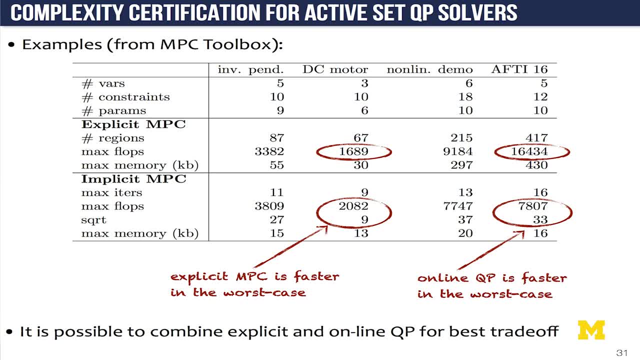 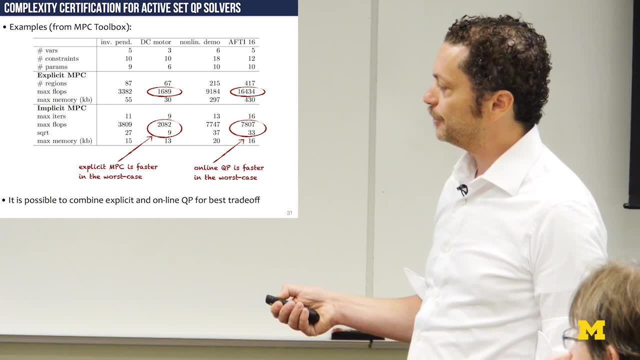 You can see, for example, in this demo which is a servo for a DC motor. here the worst case number of flops: it's smaller if you compute the explicit form than if you compute the solver online In the worst case. OK. 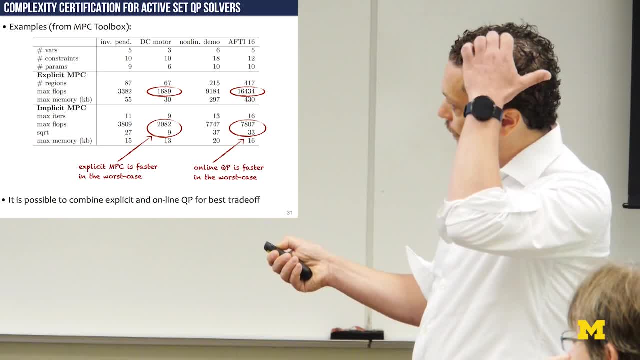 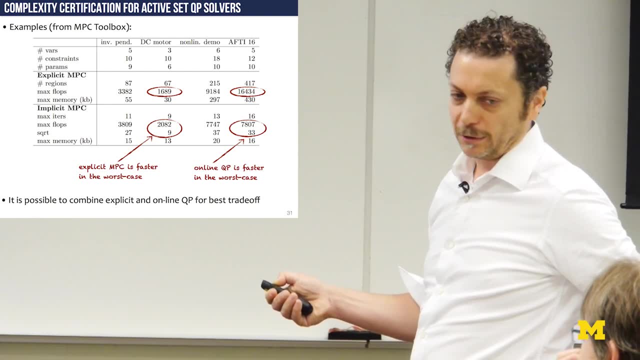 On the other hand, if you take the aircraft control problem I was mentioning before, in this case you end up doing more flops- in the worst case with explicit- than if you solve the QP online, And not to talk about memory occupancy. 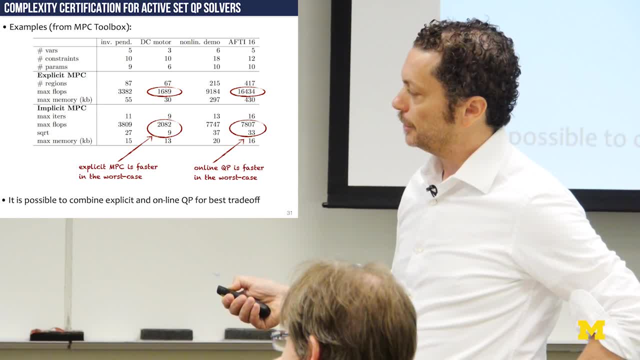 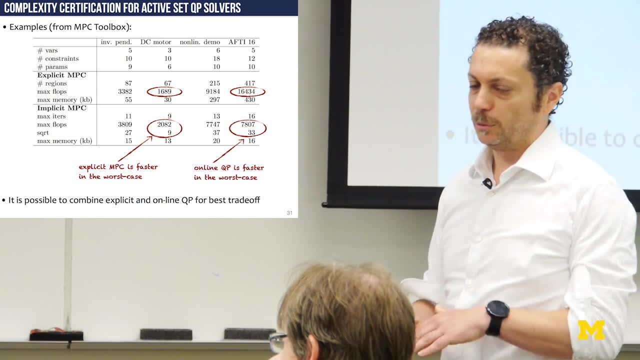 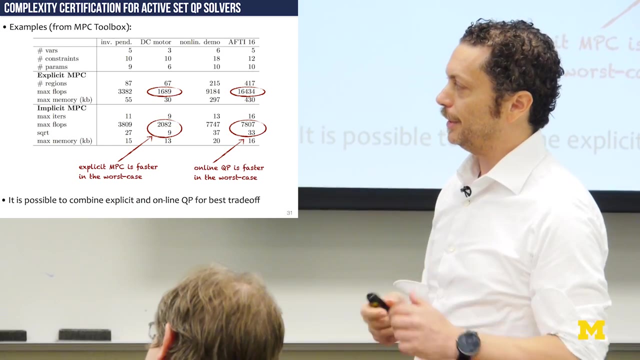 because here you have for more than 400 region. it takes 430 kilobytes to store the partition, while it takes 16 kilobytes to store the QP and the code. And actually you can do also more interesting things combining explicit and implicit solvers. 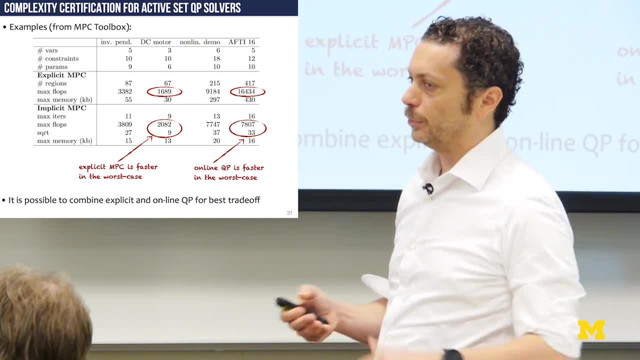 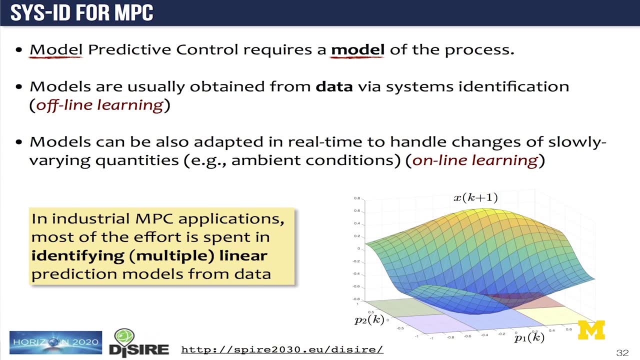 so to get this further down by doing sort of semi-explicit solver configurations? OK, I don't know, Ida, how much time do I have? Well, I think we have 10 minutes, 10 minutes or 10, 15 minutes. 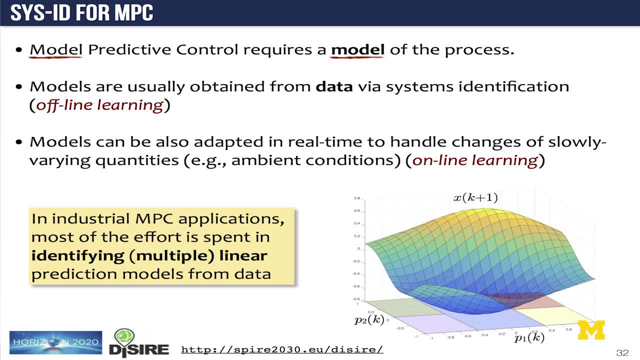 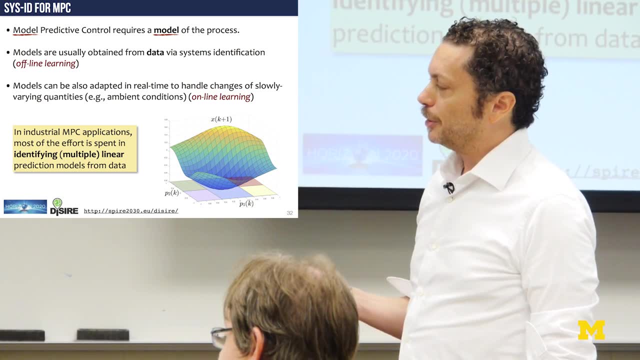 OK, good, good. So the last part of my presentation. I would like to touch a problem related to system identification for MPC, And actually not only for MPC, but this is mainly driven by MPC. So, as I was mentioning before, when 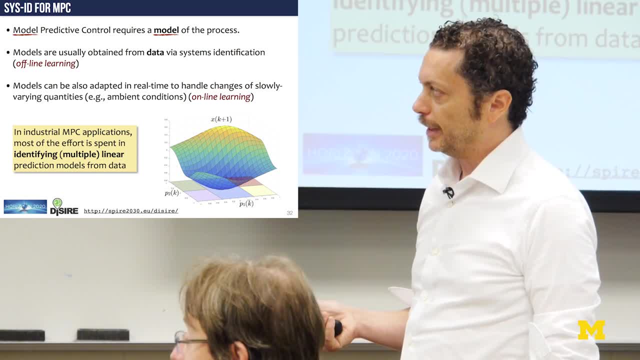 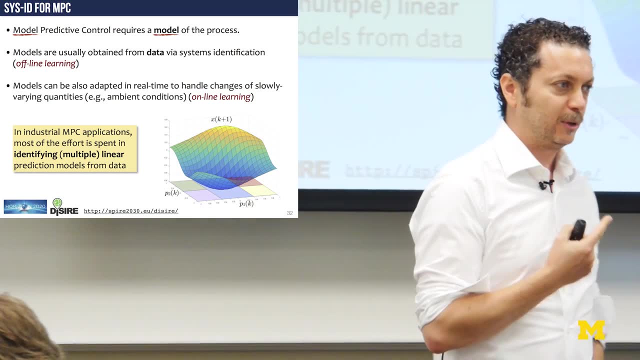 you work on real application. really, most of the time is spent on getting models and, in particular, getting linear models, And in most cases, not just one linear model but multiple linear models, Because the system you are dealing with is, in most, 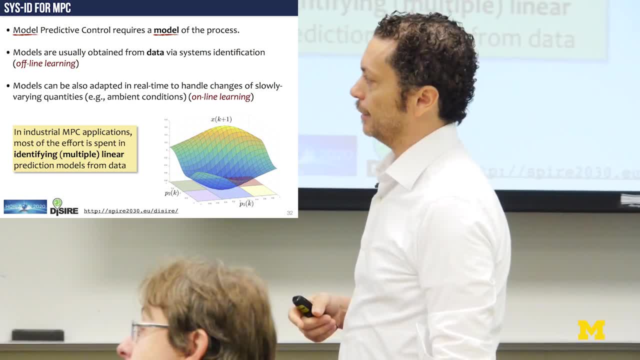 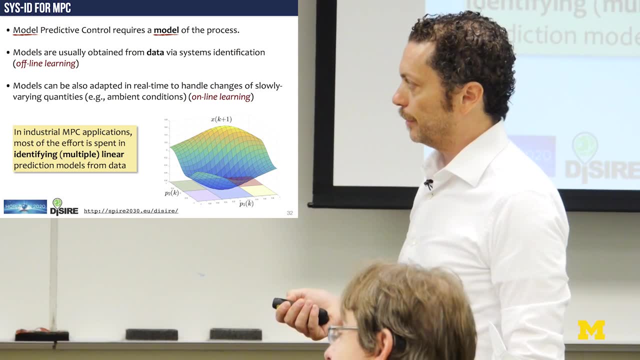 of the cases non-linear. So one linear model is usually not enough to have a good model representation. So it will not be a good prediction model if you close an MPC loop, So you have to come up with multiple linear models. That means you have to figure out. 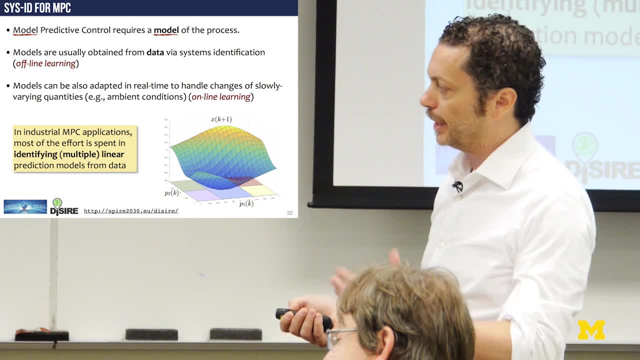 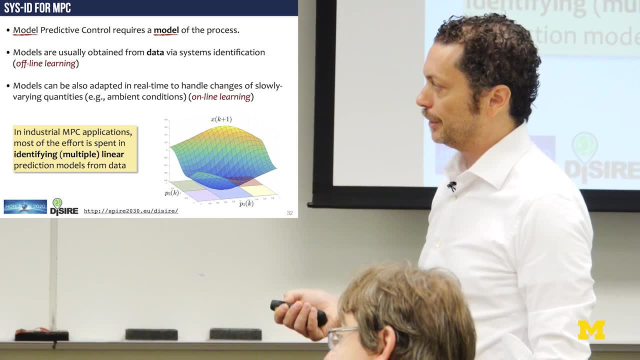 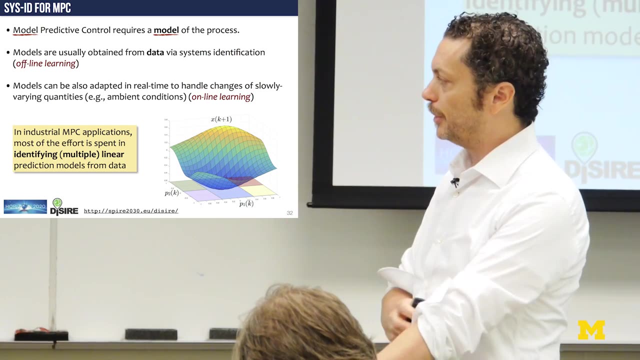 how to split certain space of parameters- which would be external parameter or states or both- into different regions and in each region which is the right linear model, And actually this can be very time-consuming if you start guessing what should be a reasonable partition. 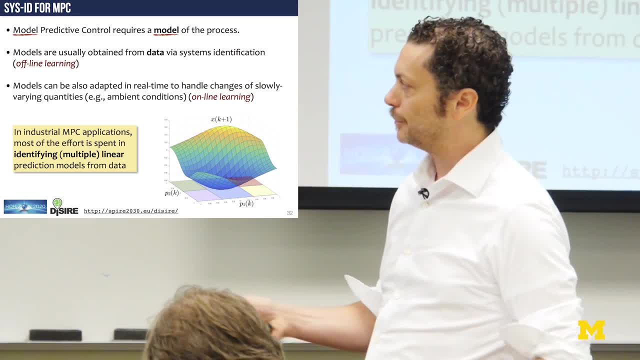 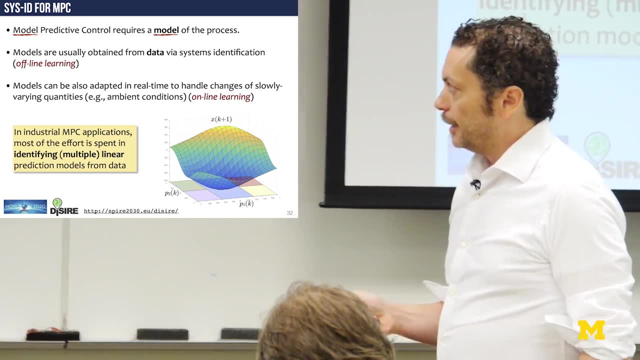 get the linear models, do model validation and then say, hm, no, that's not good, Let's get this blue region a little bit narrower and add the new one. So this can be really, really time-consuming. So this triggered some research that we did recently. 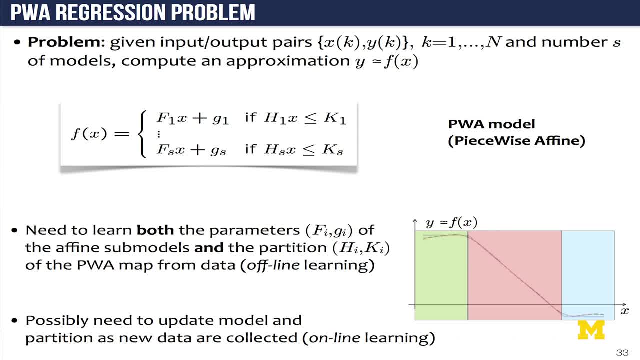 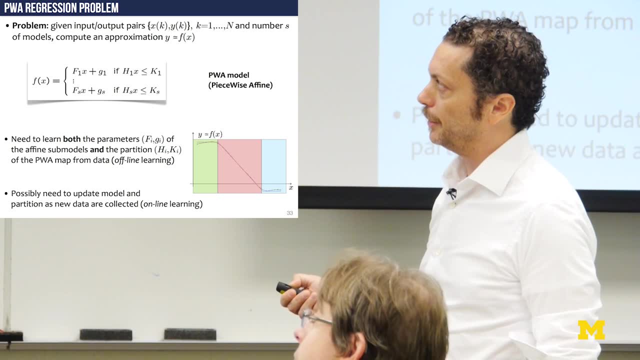 And it's a very interesting study on trying to get linear models and region at the same time. And you can cast this problem as a problem of piecewise-affine regression, Namely, you have to fit a piecewise-affine function on the data. 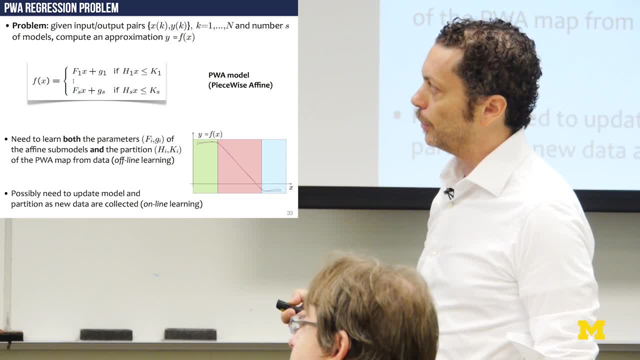 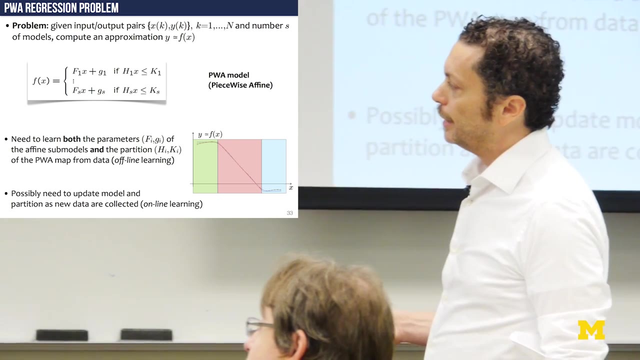 So let's say you have data points x and y. This is what you collect from experiments. You want to find the function f, which is f of x, so that f of x gives you a value that is similar to what you have measured. 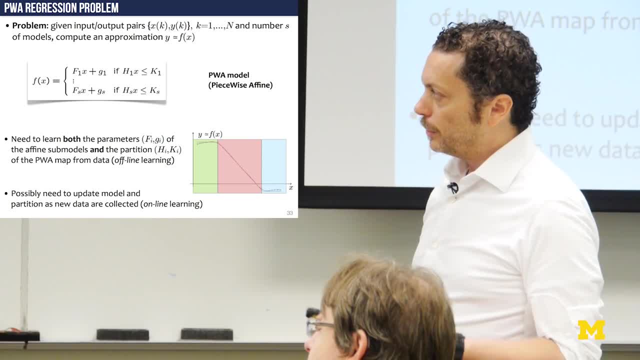 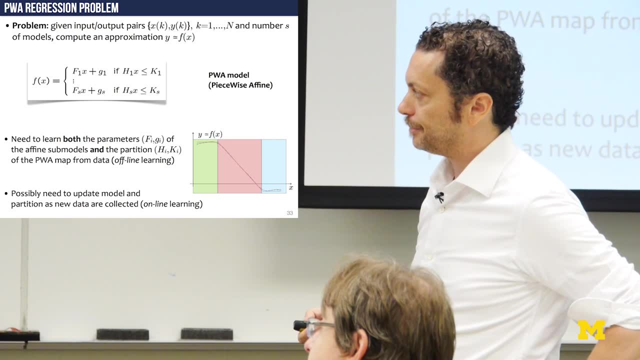 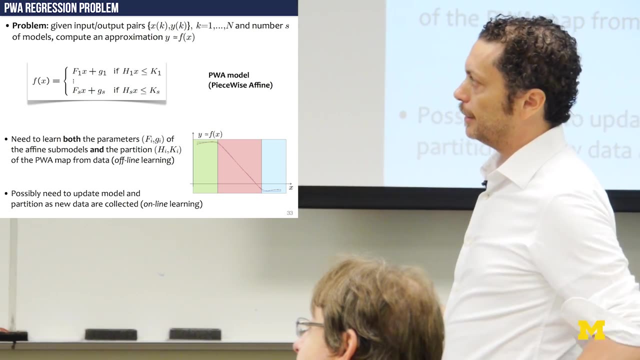 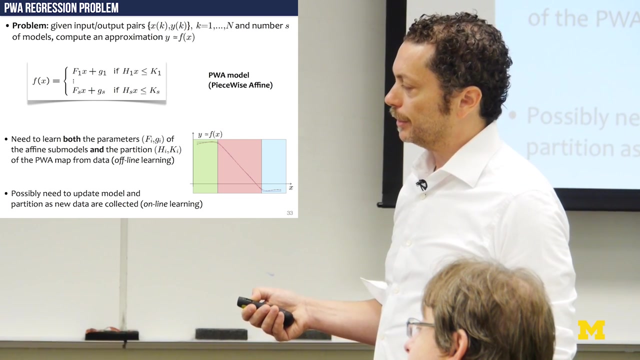 And you want to do this simultaneously. So you want to determine both the gains and the regions as one identification problem, And also you may want to do this offline, beforehand, on data collected And let's say in a batch way. But also you may want to update the piecewise-affine model. 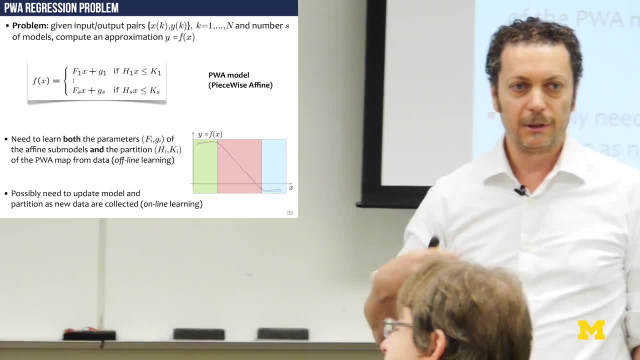 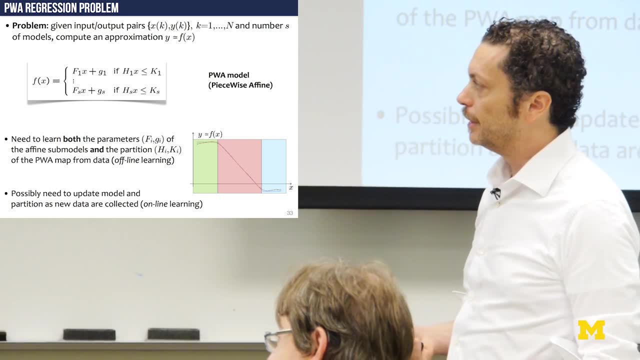 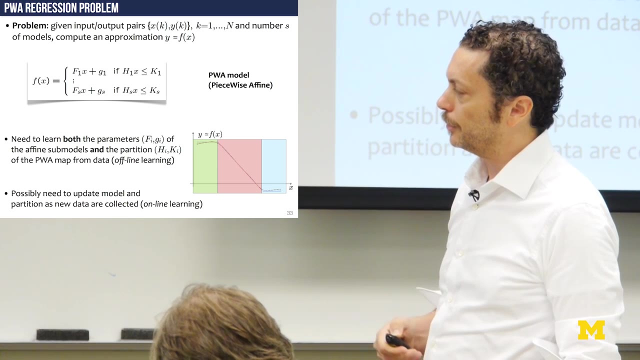 in real time if you want to do adaptive control using multiple linear models, as you have new data coming from the process while it's running. So how to address this problem? There have been already approaches to this problem, not in a recursive form, but in a batch form. 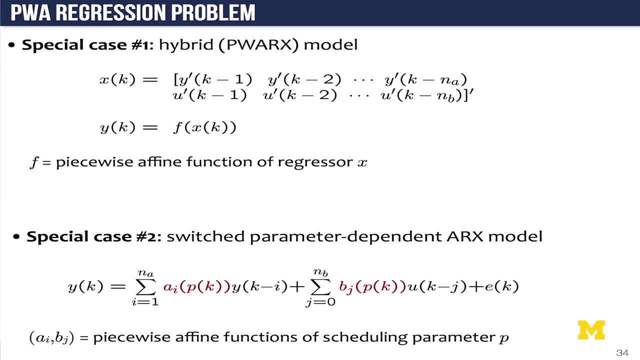 by several people in the past. A special case for system identification, in particular of piecewise-affine regression, is when x is a collection of past input and outputs And this will give a piecewise-affine autoregressive model or a linear parameter-varying model. 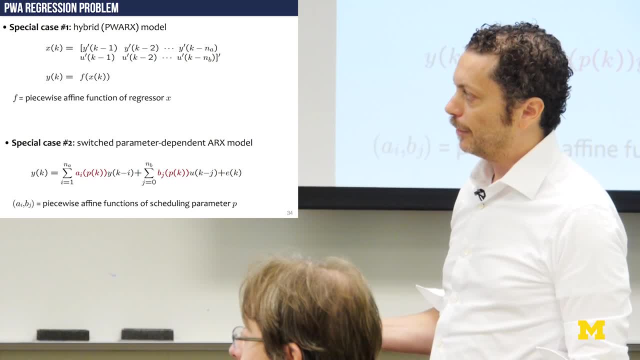 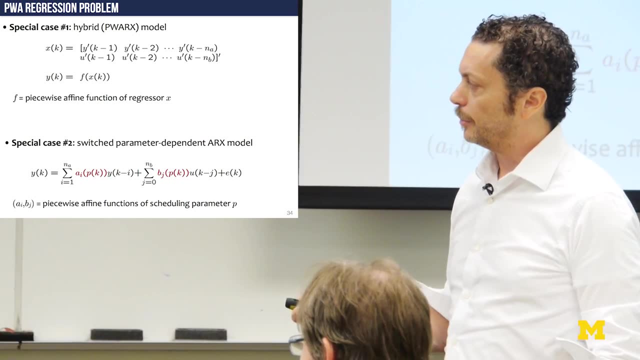 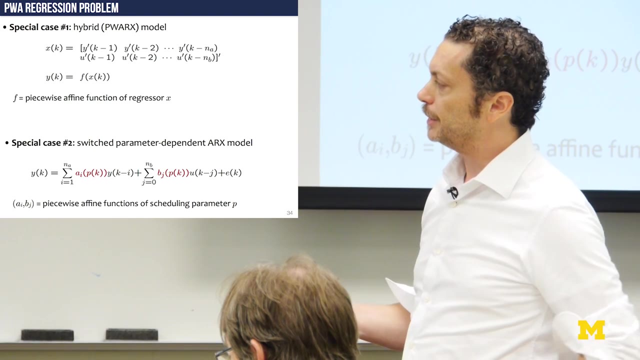 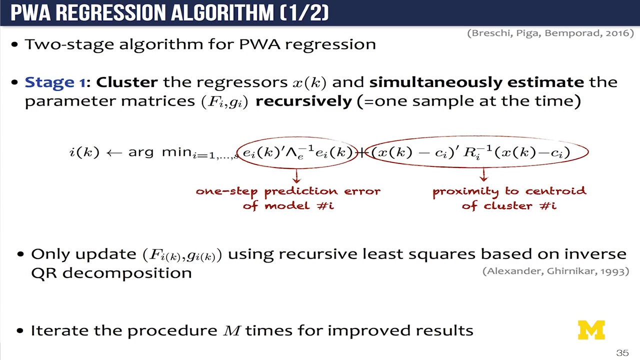 in which the parameters affect the coefficient in a piecewise linear way. So both these models are actually quite powerful models to represent nonlinear systems and especially if you have discontinuities And these can be cast as a piecewise-affine regression problem in this form. 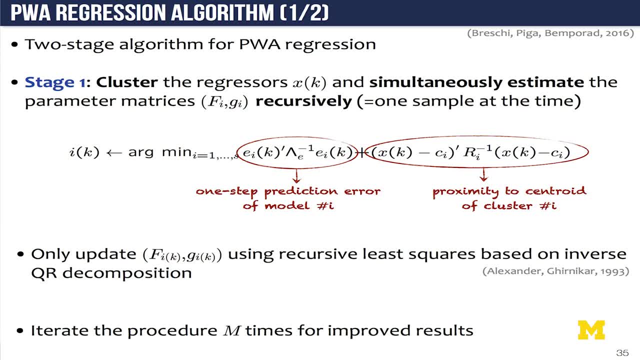 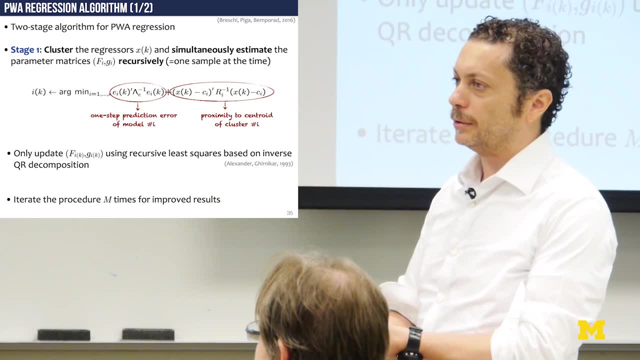 Now, the approach we came up recently together with Valentina Boesky and Daniel Piga and Luca is a two-stage algorithm. It can be both recursive or batch, And the idea is the following: Is to use recursively squares on the multiple linear models. 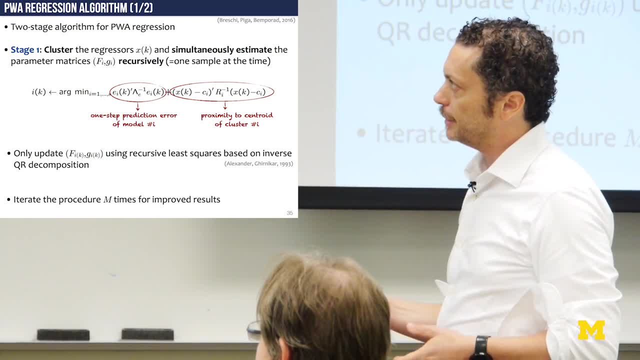 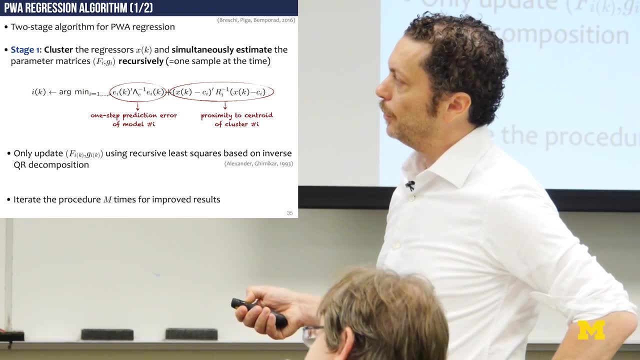 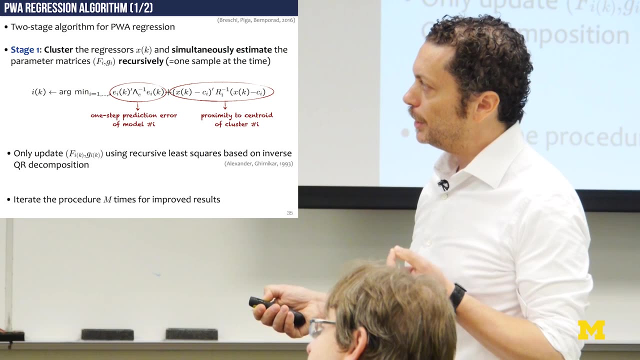 and take one data at a time. So you have a certain data set of x and y's. You take one data at a time And for each data you look which is the model that gives you the least prediction error and which is the proximity of the data point. 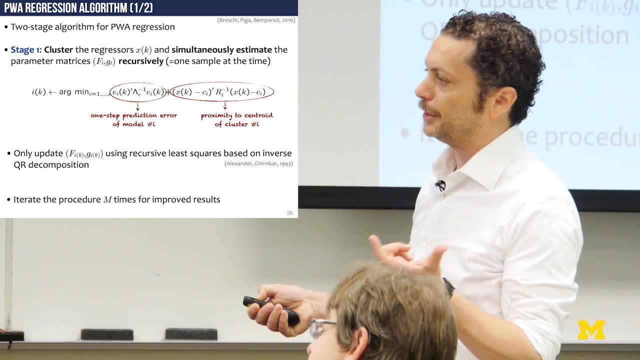 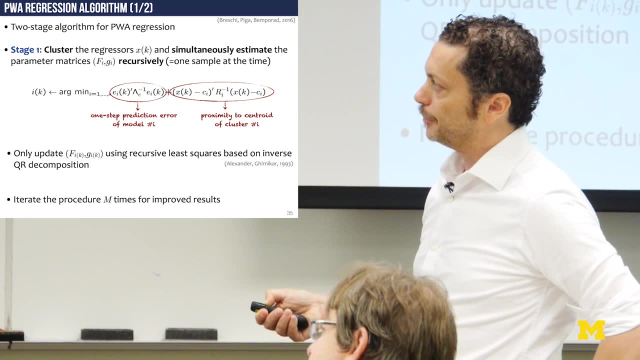 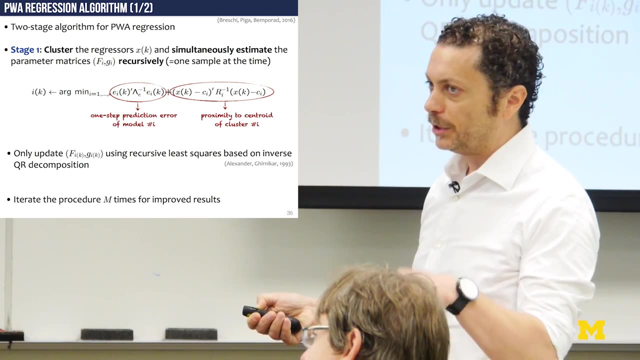 to the set of other data that you have already created, OK, Collected and assigned to a certain mode. And then you minimize this figure here And this will be the mode that you assign to the current data point. And you keep doing this for all points. 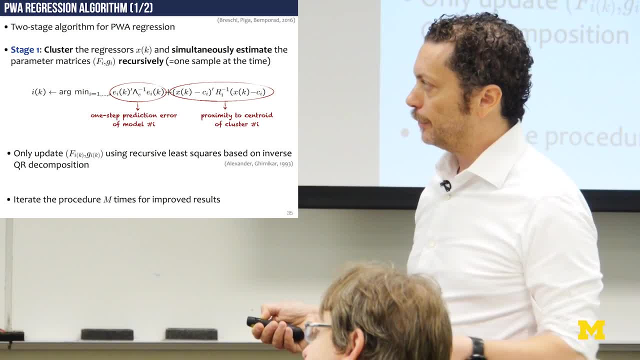 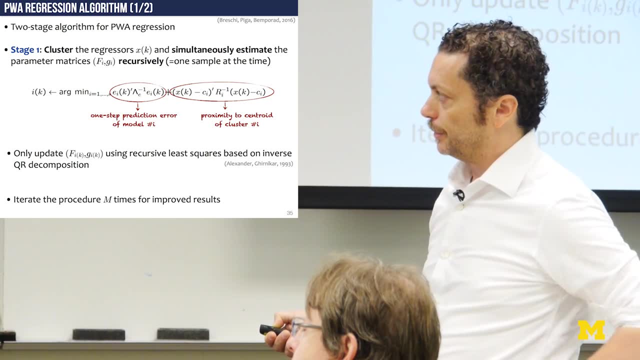 And while you do this, you use recursively squares in a form that we took from a paper in signal processing by Alexander and Giernikar. that is very, very efficient. It's based on inverse QR decomposition updates For solving recursively squares. you only 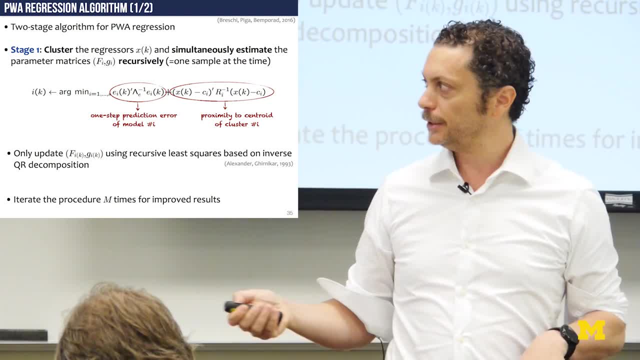 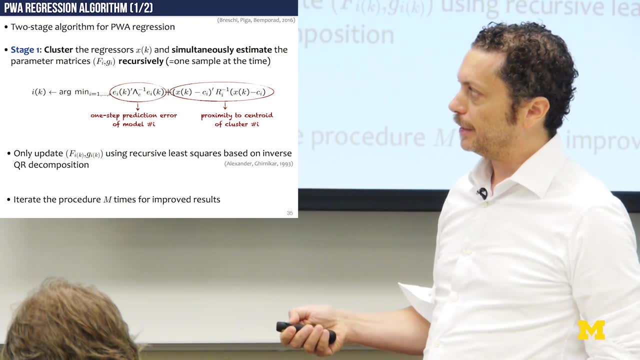 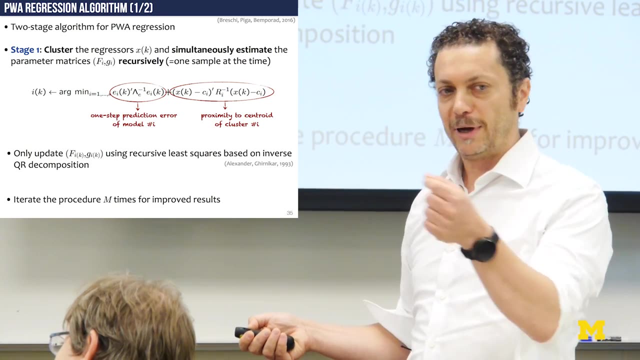 update the parameter vector that is associated with the mode that you are currently assigning to the data point, And this, in the end, after you process all data, gives you a set of models. Actually, you can run this multiple times, So you can use the results to initialize a new pass. 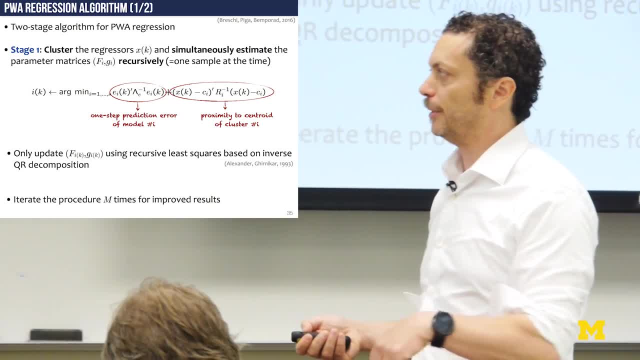 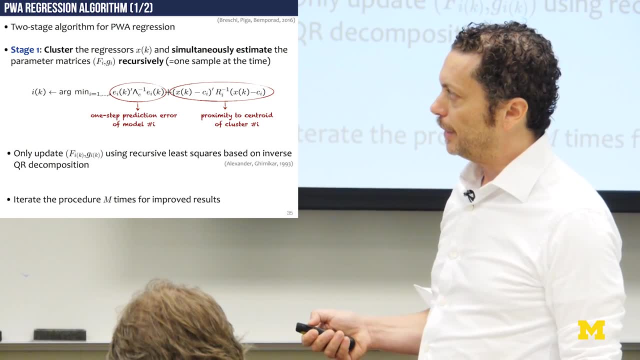 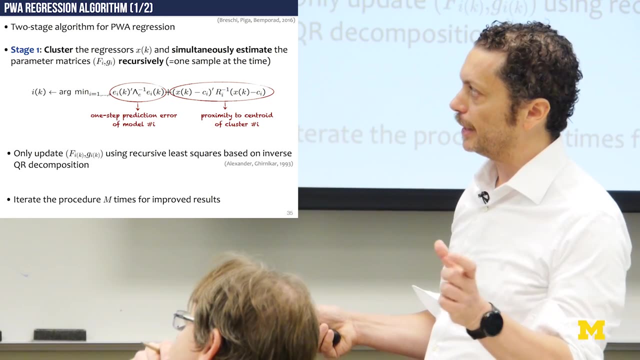 on the same data points, You will obtain a different result. Usually it's a better result, And you can keep doing this a few times, say 10 times, And then, once you have obtained the models and the clusters- so you have obtained subsets of the data points- 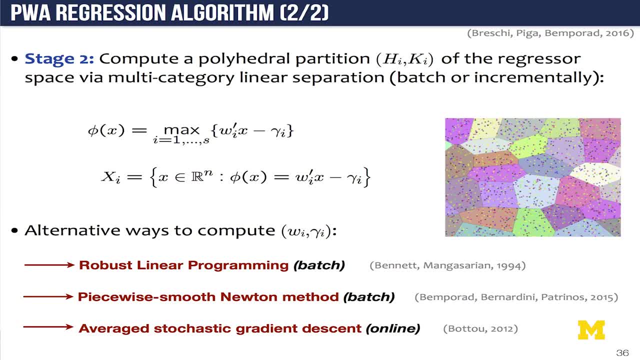 corresponding to different models. then you can solve a piecewise linear separation problem. That is, the problem of finding a function- phi, which is the max of linear functions- that defines the regions in your piecewise affine partition. So this is a way to separate clusters. 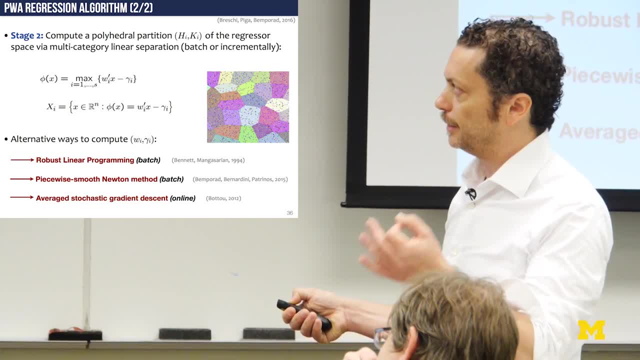 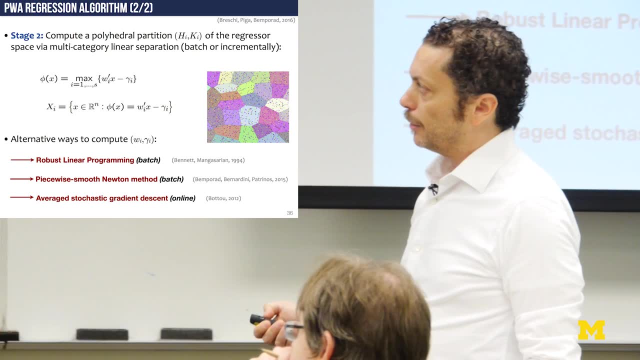 If the clusters are piecewise linearly separable, you will get an exact partition. Otherwise, you will have some points that go in the wrong set. This is solvable. It can be solved. This is a standard approach to solve this robust linear programming. 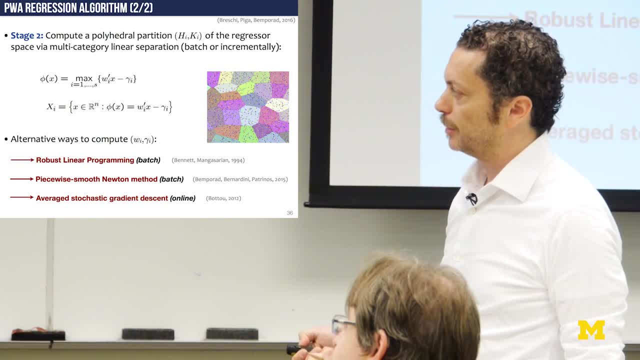 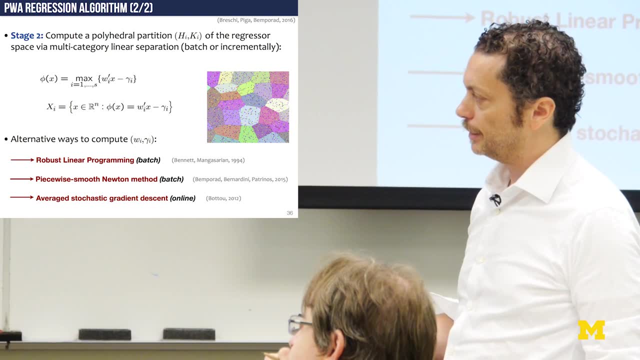 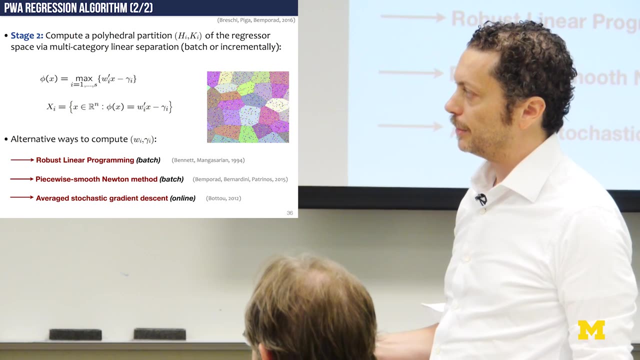 We came up in this paper with an approach which is quite somewhat more efficient, based on a piecewise smooth Newton method, to solve the same problem, The problem of finding this function, phi here- And also an incremental version which is based on average stochastic gradient descent. 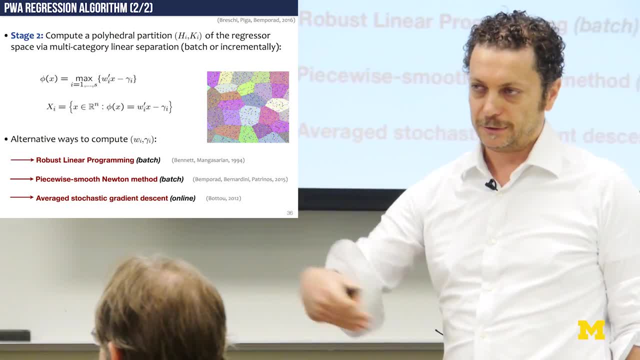 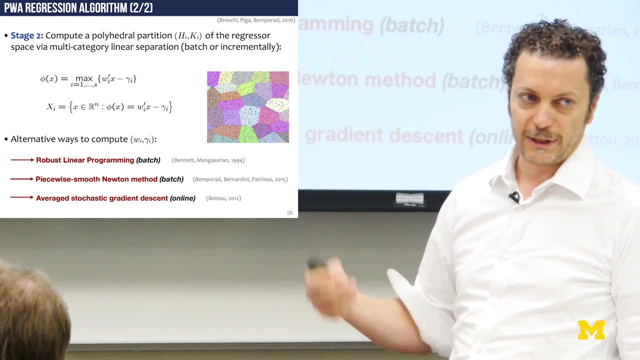 that it's amenable to process the data in real time online when new data become available, And actually it turns out to be even more efficient, when you have huge data sets, compared to the other two methods. And here are some results. 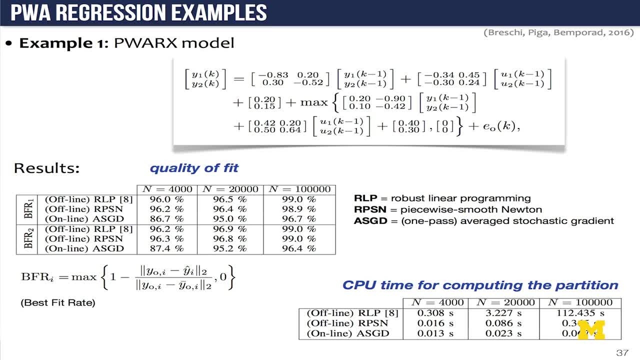 So this is actually the underlying model is piecewise linear. We want to check whether we can solve it. We can retrieve the model using the algorithm. Actually you can. So this is the best fit rate. This is two outputs, two inputs. 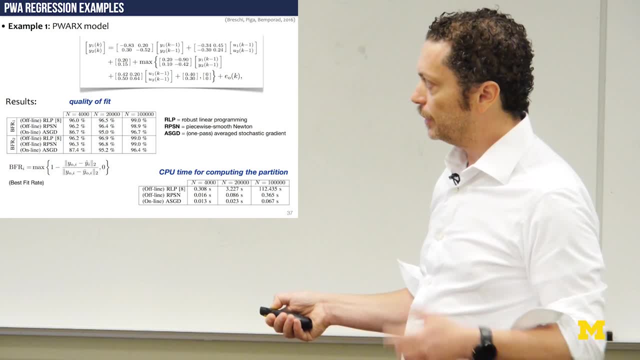 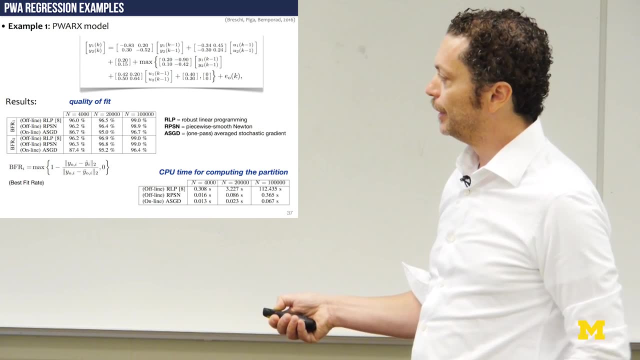 The best fit rate, which is a figure telling you how good is your predicted output in simulation on fresh data compared to the data that you have collected for validation. So these are the best fit rates on the two Outputs. you see as you collect more and more data points. 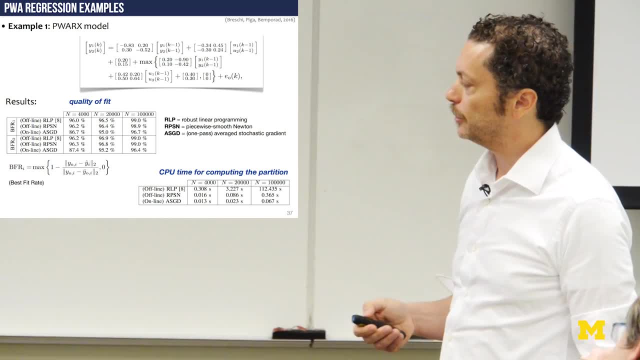 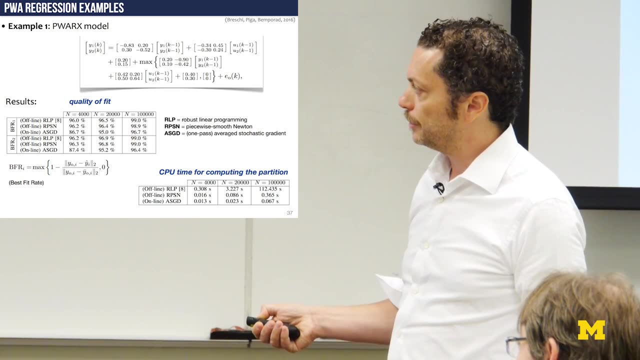 you get closer and closer to one, which is the maximum you can achieve. And here is the comparison of the method for piecewise linear separation: Robust linear programming is actually the slowest, And incremental optimization using average stochastic gradient descent is actually considerably faster. 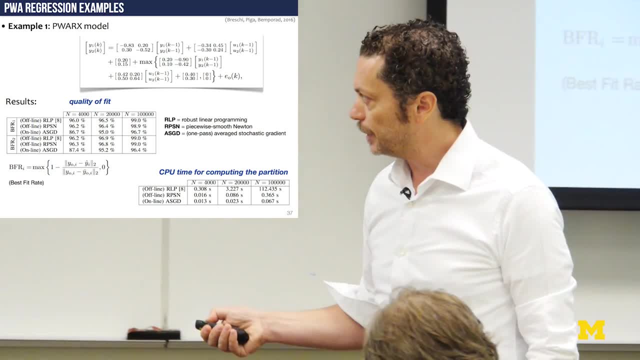 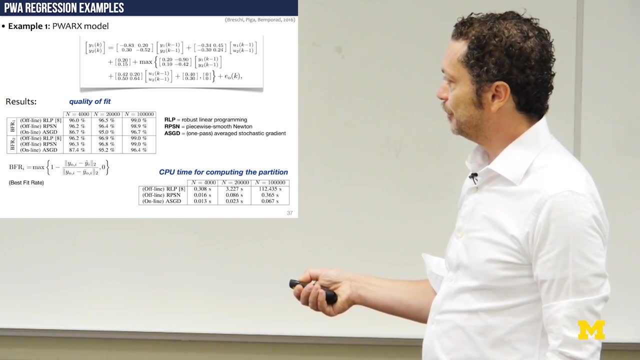 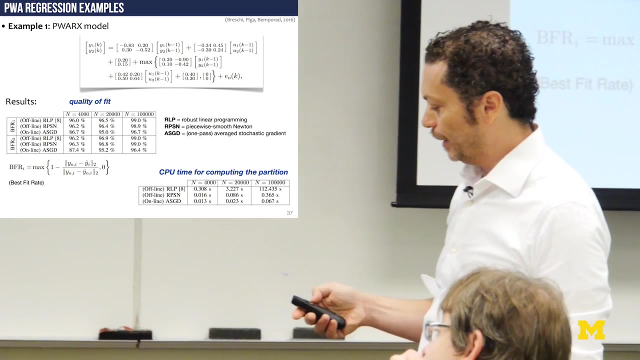 when the number of data points is large. So in this case, for example, one, This one, 100,000 data points. It's about how much Three. You can see the figure is orders of magnitudes faster. And here is another example. 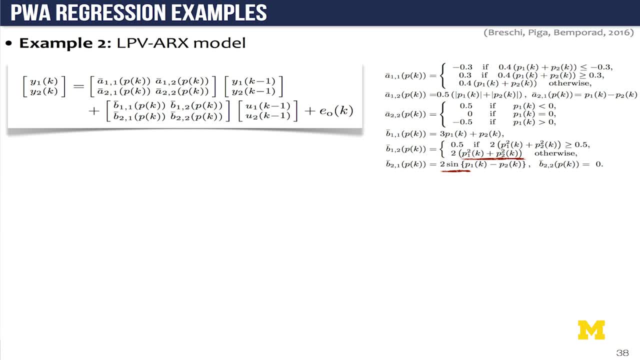 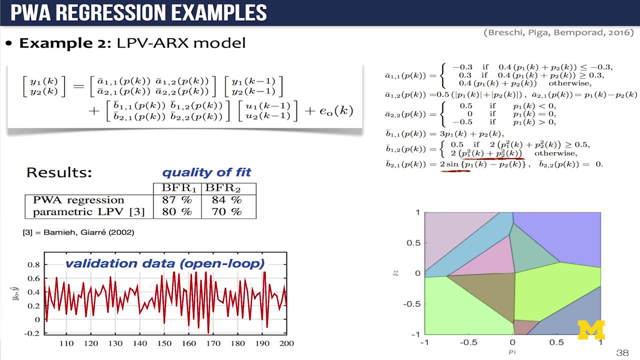 Now the underlying system is nonlinear. You see, here you have quadratic terms and thresholds and sinusoids. This is what you get out of the algorithm. So you select: You want to have 10.. You want to have 10 possible modes, And this is how the algorithm figure out. 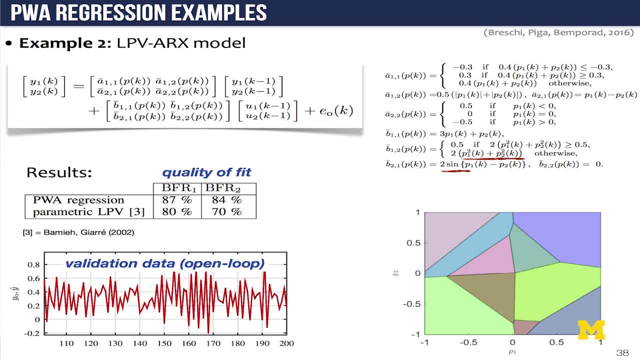 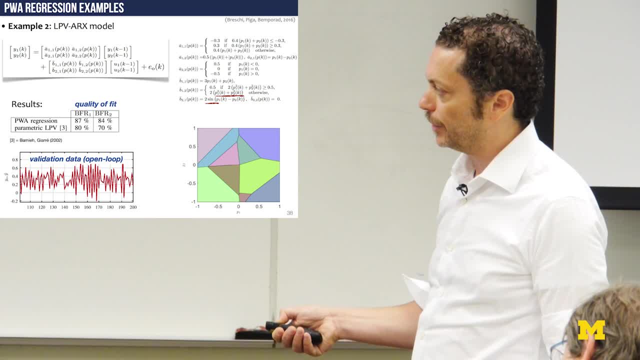 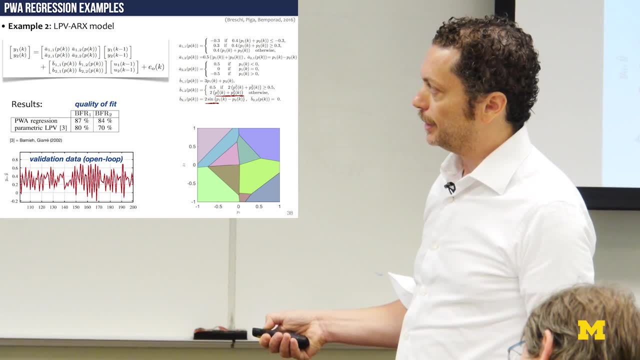 what the clusters are, the partition is, And this is the best fit rate you get, So it's quite high. Here is an open loop simulation of validation data. You actually cannot distinguish much the prediction, the open loop prediction, from the data. 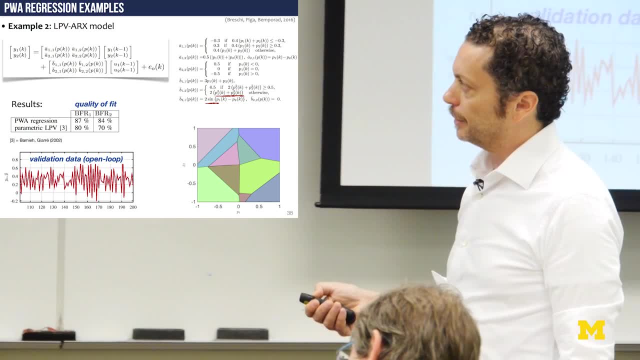 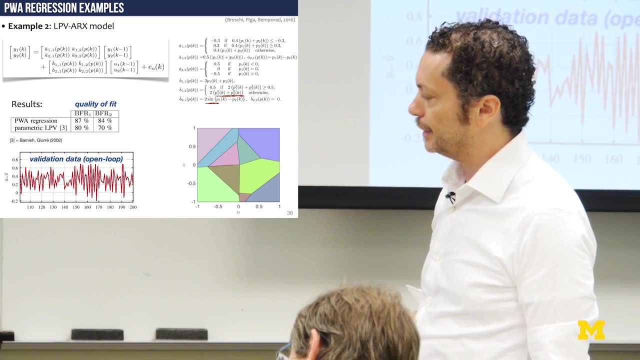 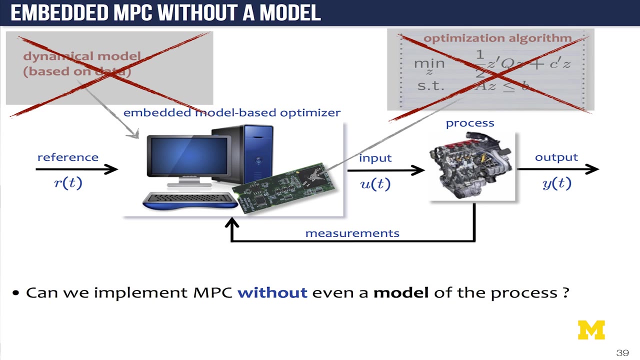 So this is a good way of approximating nonlinear model. Now, last item: Can we do MPC even without a model of the open loop process? 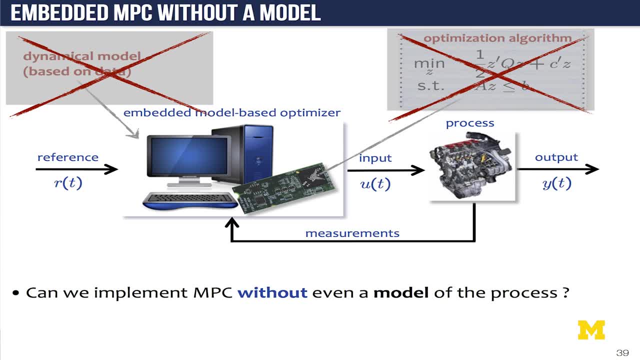 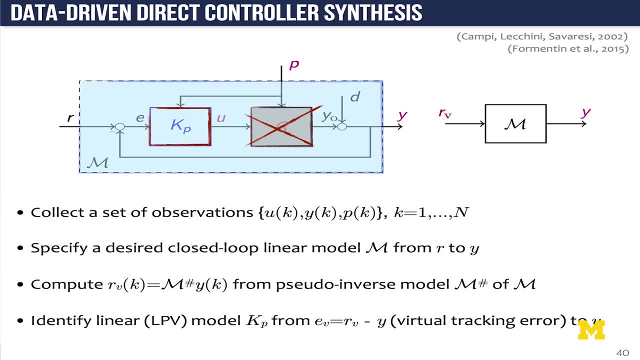 So got rid of the solver using. Now can we get rid also of the prediction model? The answer is again yes. Here is an idea: and control the synthesis from data from Campi Lachini, Savagnese, back in 2002,. 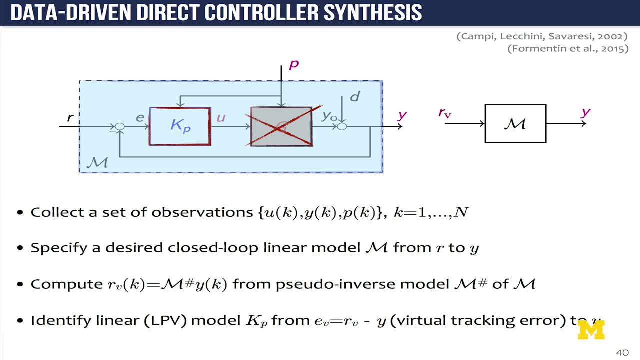 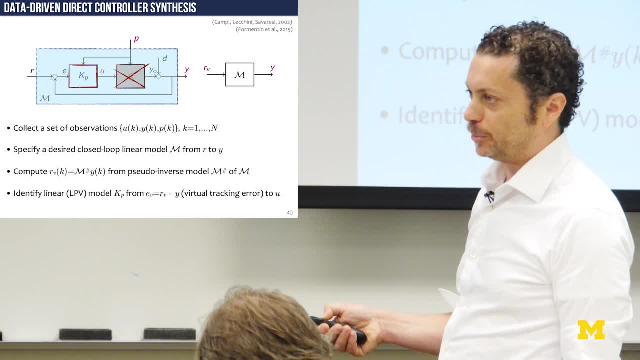 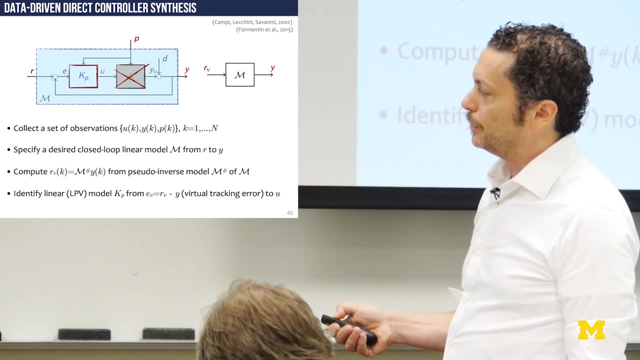 and Simone from, and others Last year. let me tell you what the idea is. You don't know the process. You only have input, output data and possibly parameters affecting the process. Now what you want to do is to impose the closed loop. 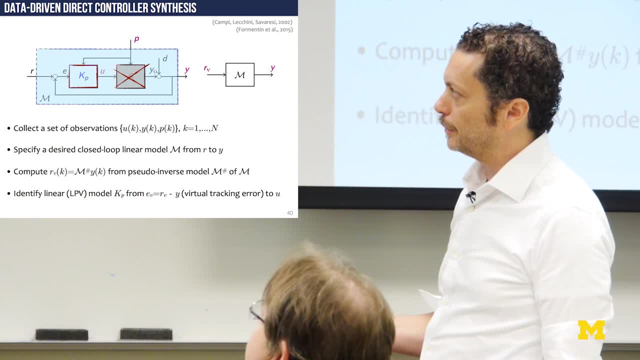 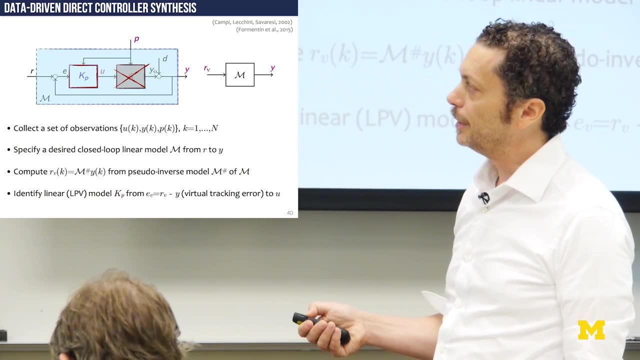 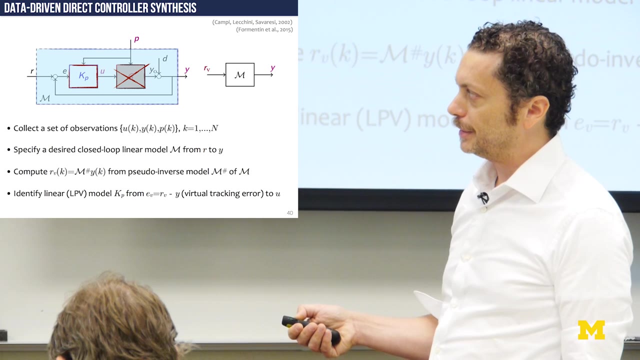 function. say I want the closed loop from the reference to the y to be, let's say, a first order function, linear function. Then you can identify the controller directly, rather than going through first the linear open loop process of the system, then designing the controller. 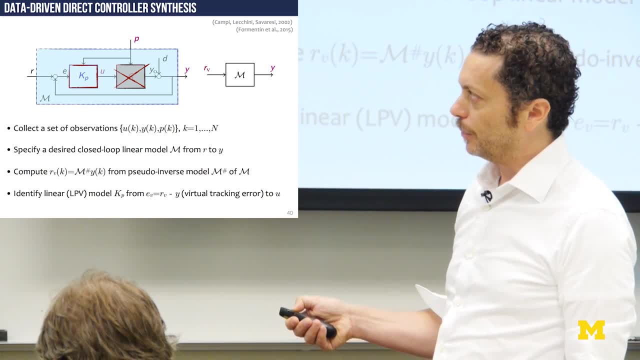 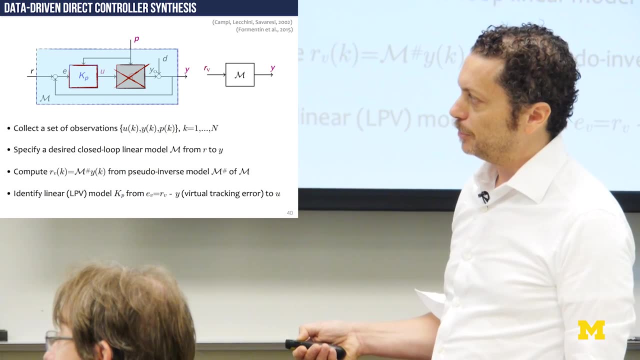 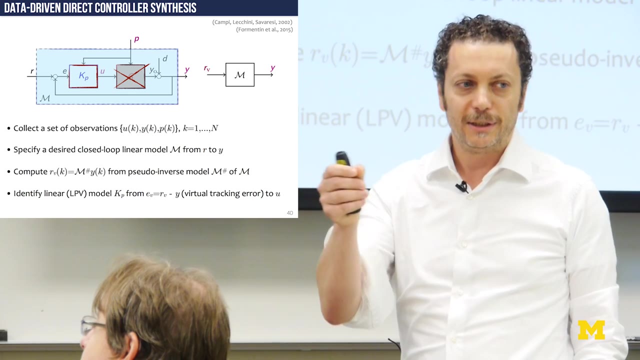 And here is how it works. So you collect the data, You specify what your desired model is, Then you take the output samples And go backwards and do a pseudo-inverse of the model to figure out what the references would have been to get those outputs that you have collected. 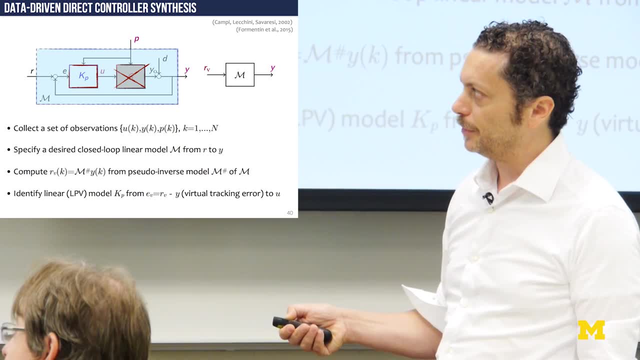 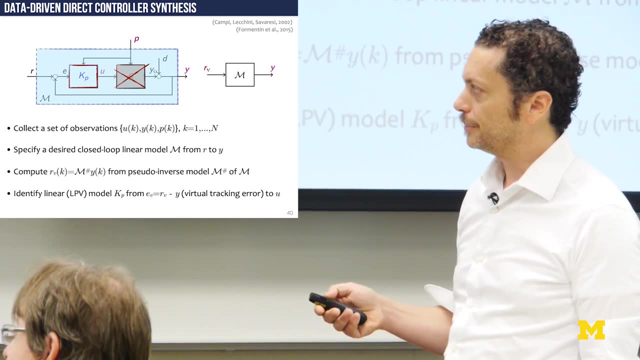 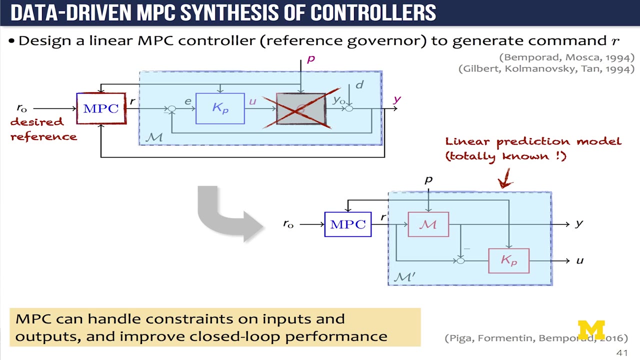 And once you have the references, you can compute the tracking error. And then you have inputs and outputs of the controller and, eventually, parameters to be able to identify the controller. And then, once you have this, even without having the data, Having specified what the open loop model of the process is. 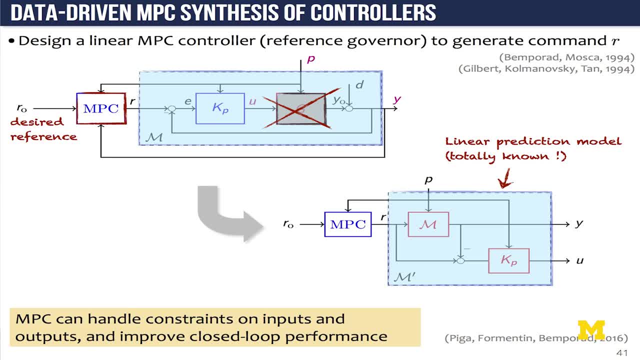 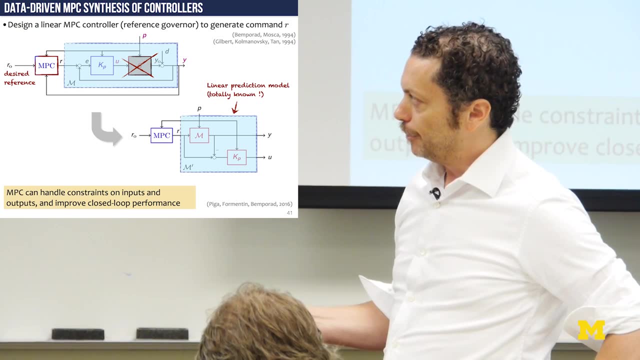 you now know what the closed loop is, which is your model, assuming that your identification process is successful. So you have figured out a controller that reasonably well makes the system in closed loop behave like m. So y would be the output of m. 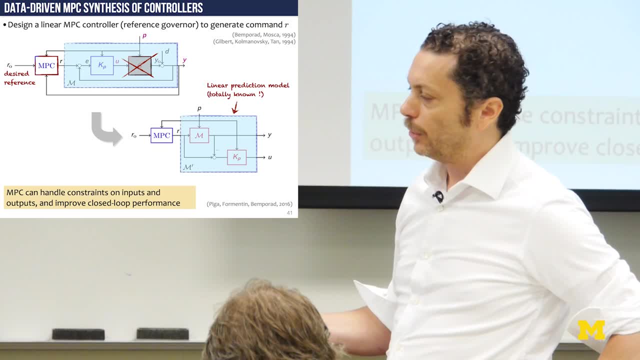 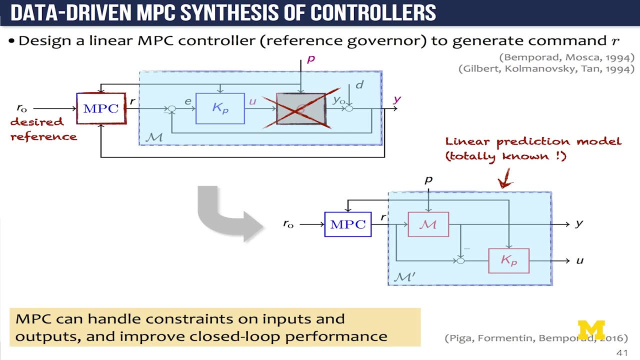 And? u is the output also of a known system, which is m cascaded by the controller, And now we use ideas from reference governance, some topic that Ilya and I are very familiar with, as we did our PhD on this topic many years ago. 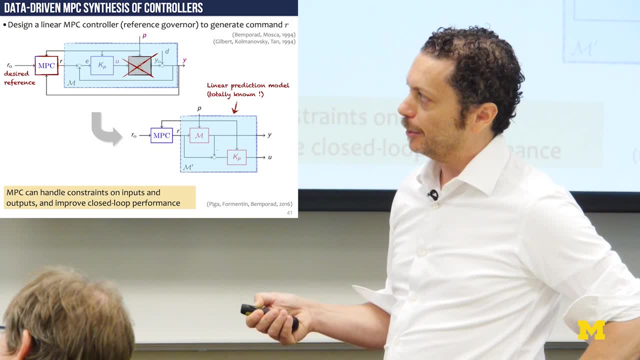 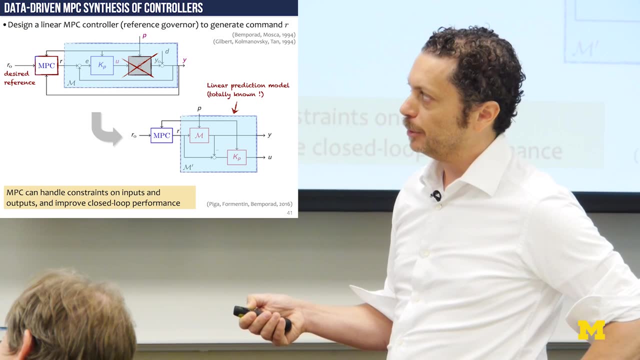 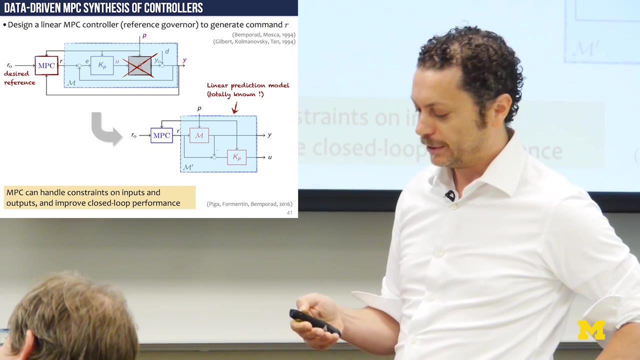 So the idea is really to use the MPC as a reference governor on the closed loop system specified by m, So to improve performance over the m you have specified, and also to be able to improve performance To impose constraints on input and outputs, And here is an example: 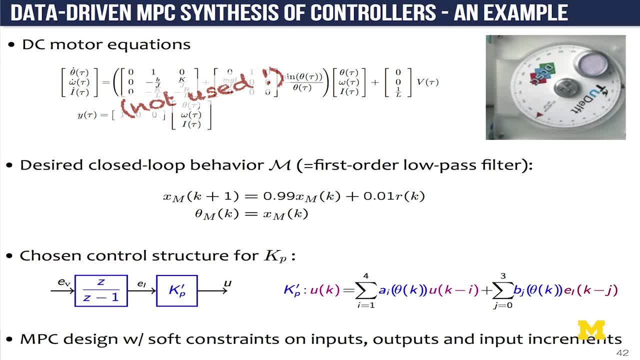 This is an experimental experiment we had the courtesy to get from DELT. The model is actually non-linear. It can be modeled as an LPV system. We actually don't use the model. This is just to give an idea what the model is. 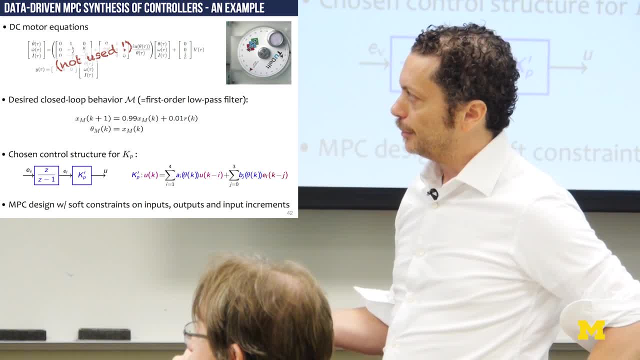 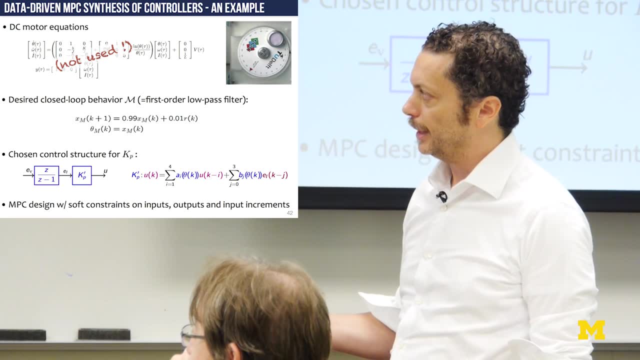 We don't use this model. This is the closed loop we want to achieve. So slow, first order dynamics, And this is the parameterization of the controller. So the controller is parameterized. 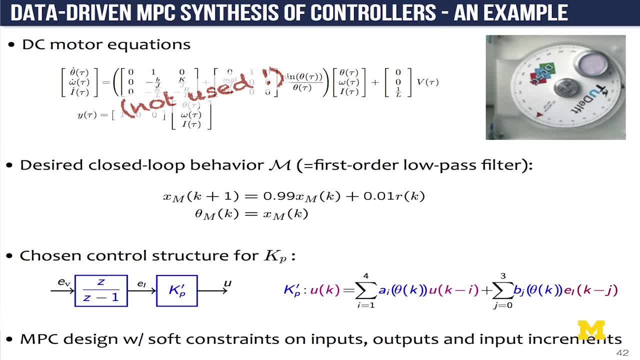 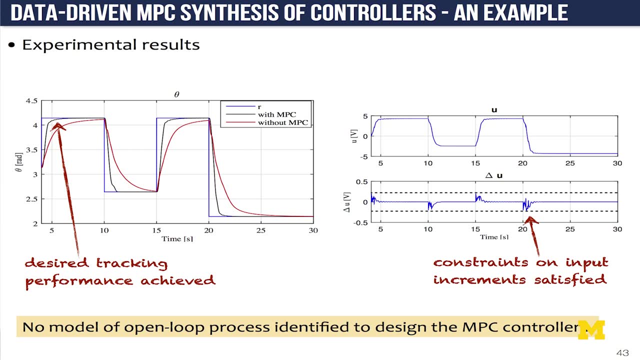 as an LPV controller where the parameter is theta is the angle of the device. And then we do an MPC design on top of this model to enforce constraints and improve performance. And here's some results. so the blue one is the reference you want to track. 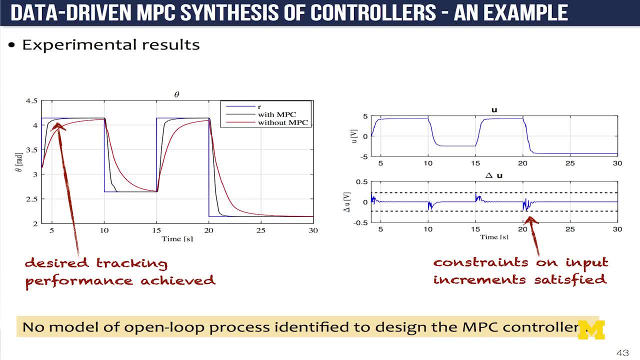 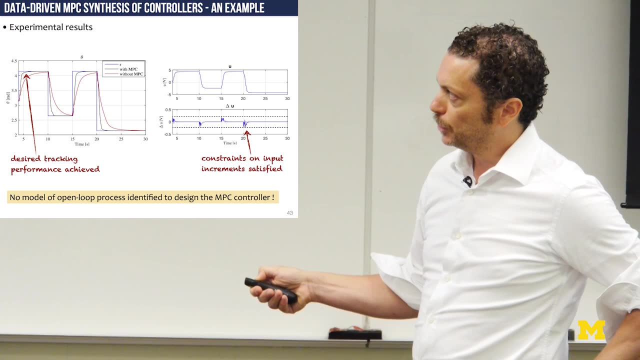 The red one is what the nominal model M would do. So it would actually track the reference, because the controller you have obtained KP from identification is pretty good. It's a slow system, So that's what MPC does. It will improve performance and satisfy input constraints. 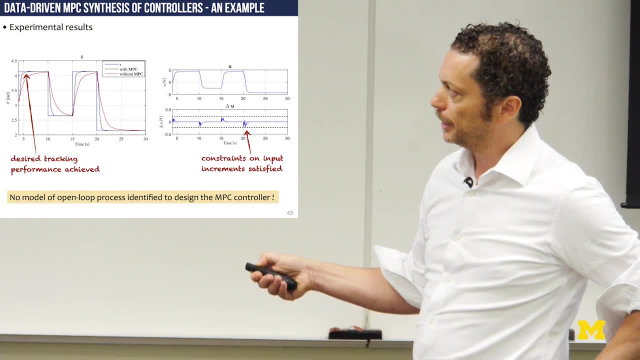 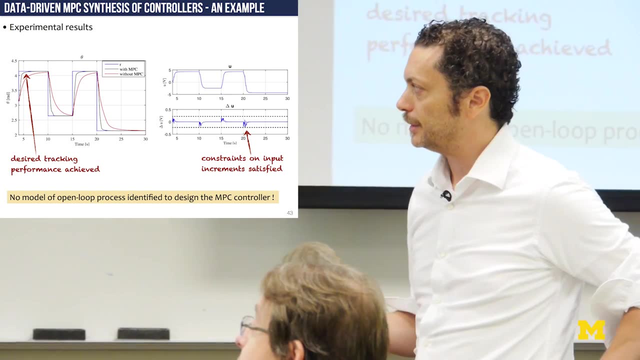 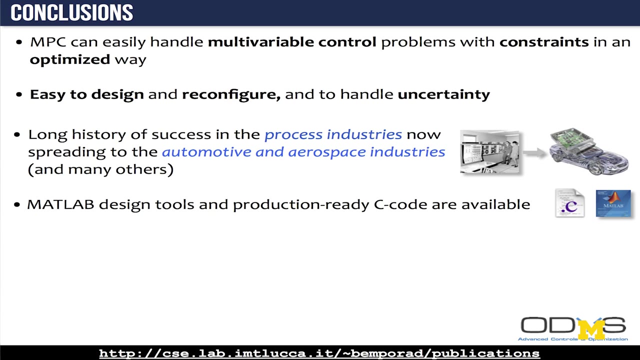 and constraints, even on input increments. So to do the tracking in the presence of constraints, again without having specified an open loop model of the process. All right, That's a good time to come to my conclusions. So I hope I gave you the idea that MPC is quite 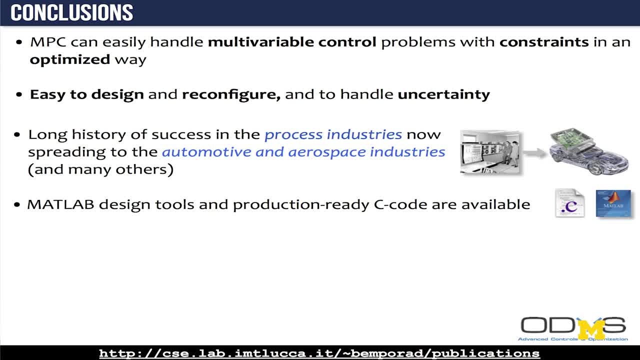 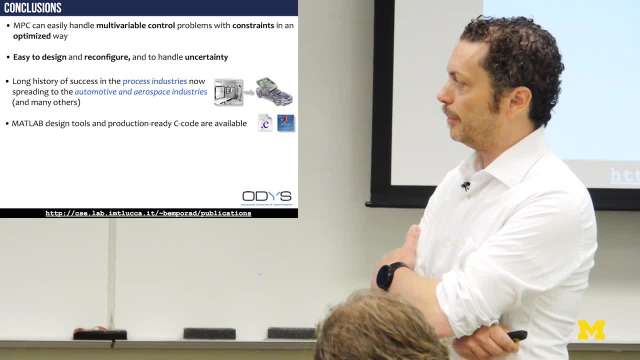 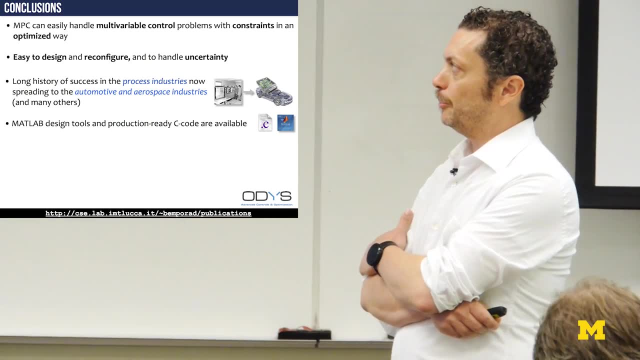 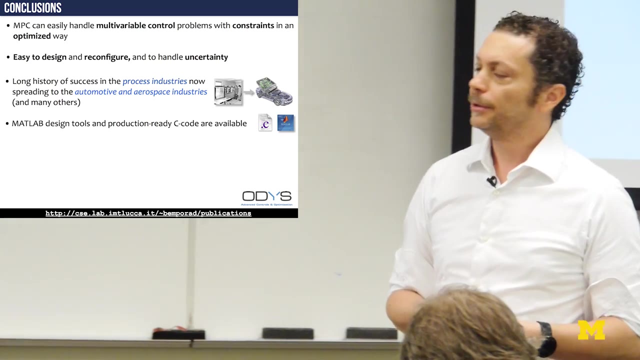 a nice and versatile technique to handle control problems where you have multiple input and outputs and constraints And you want to drive controllers that optimize certain functions. Another feature I didn't mention is the possibility of MPC to reconfigure itself easily. Say, an actuator gets stuck at some point, what do you do? 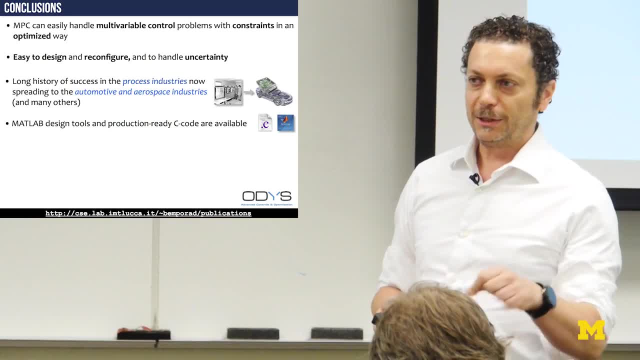 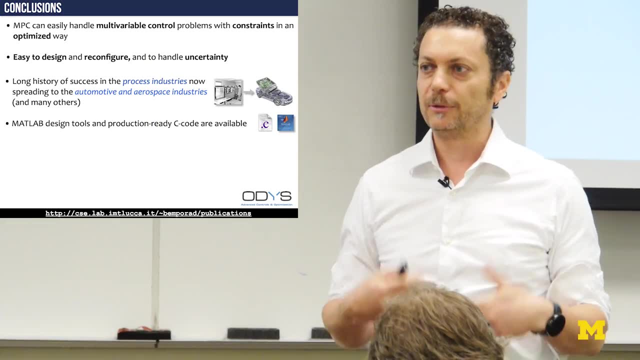 You just impose inequality constraints in the QP. Say U1 equals 0. And then you don't have to change anything else. You just solve the QP with these additional equality constraints And it will still give you the best solution you can achieve based on the current configuration. 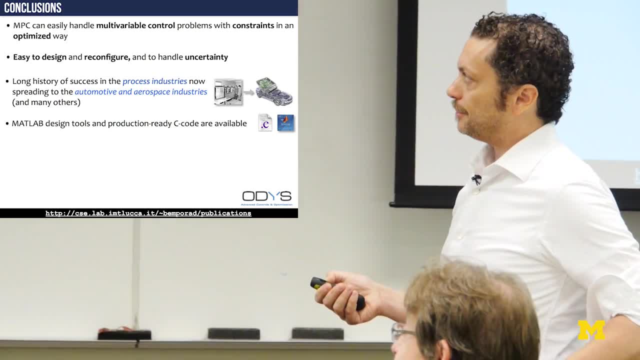 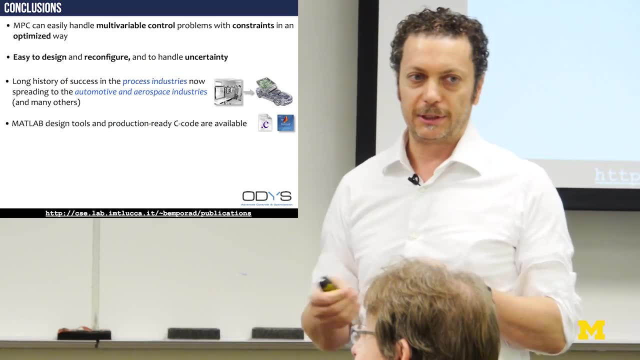 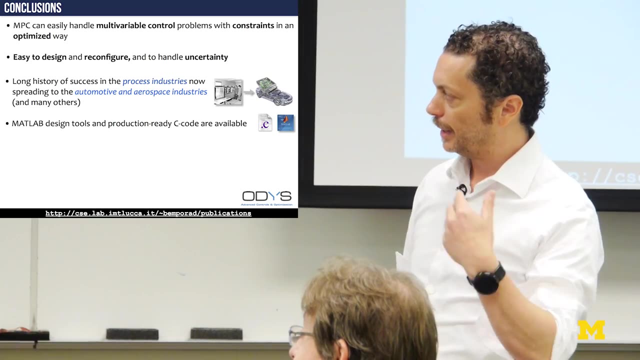 It's actually also a good technique to maintain the design. So once you have a design, if anything changes in the model- say you change a part of the process- then you just have to revise the part of the process in the model And then you can try the same set of weights. 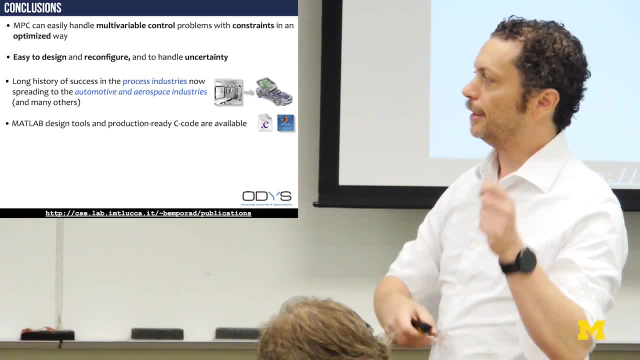 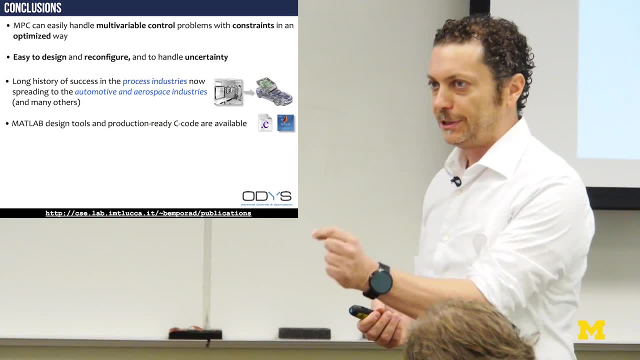 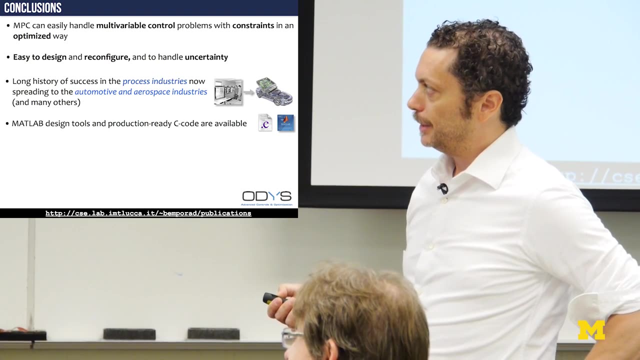 or slightly revise the weights, But you don't have a very complicated control law, that is say finely tuned for a particular configuration and is not easily moved to a different configuration. It has a long history of success in the process industries I was mentioning before. 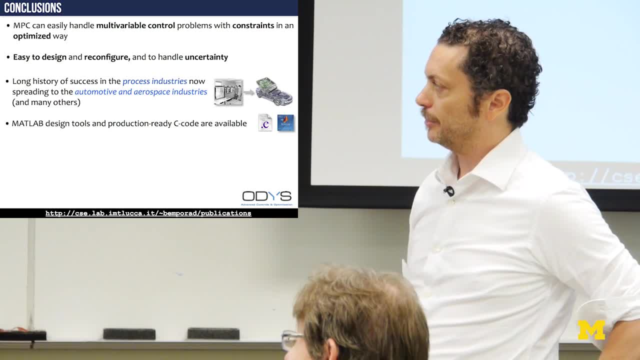 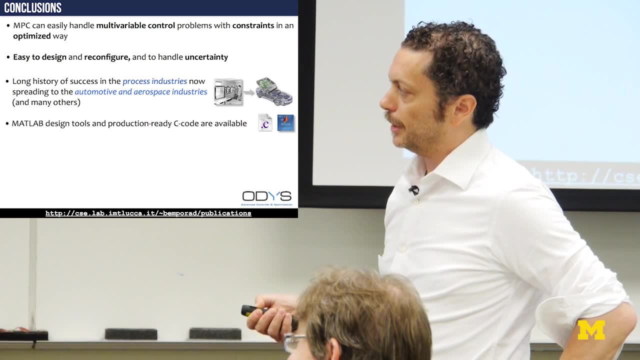 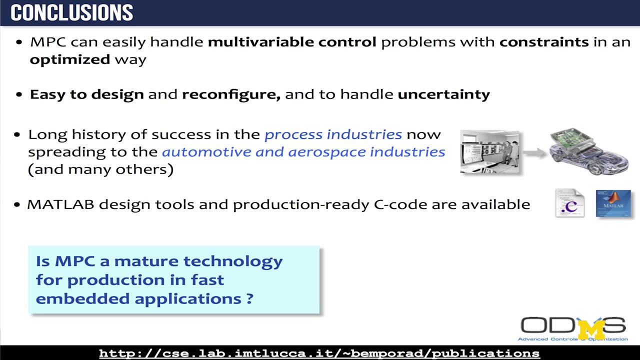 It's spreading Now. you see, it's spreading in the automotive industry and in the aerospace industries more slowly, But it's happening there And it's also very important. there are good tools to support the design. That's actually what makes the technique spread in industry. 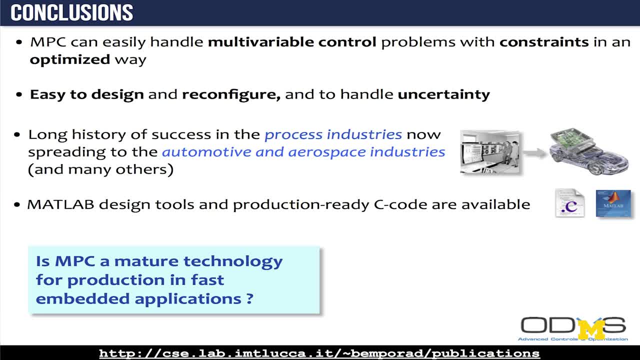 So if you ask me if this is a model with mature technology for production in embedded application, my answer is definitely yes. No point, It's there, It's technology, It's happening. And with that I conclude my presentation. Thanks a lot for your attention.